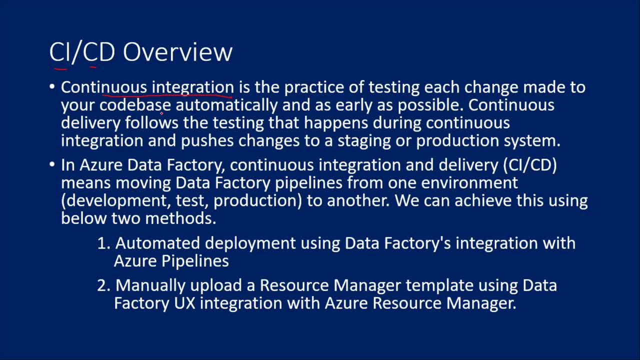 practice of testing each change made by your code base, automatically and as early as possible. Then what is continuous delivery? So this continuous delivery? actually, it follows the testing, what happens during continuous integration, and then it will push or publish the change, changes to a staging or production system. right, So staging or production environment. 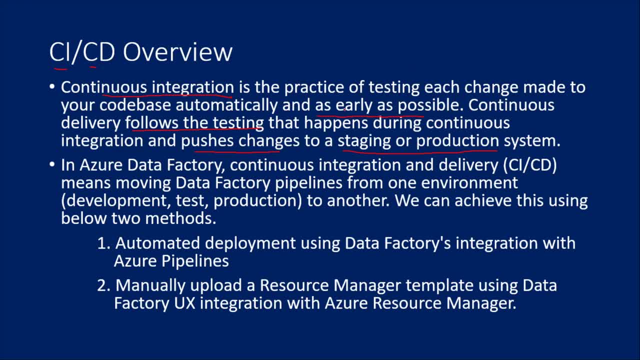 So, once you test your changes as quickly as possible using automated fashion, using continuous integration, this continuous delivery is going to follow the same path: whatever you tested right, it is going to take that code and it is going to automatically deploy that code into staging or production environments, depending upon your configuration. So this is what people 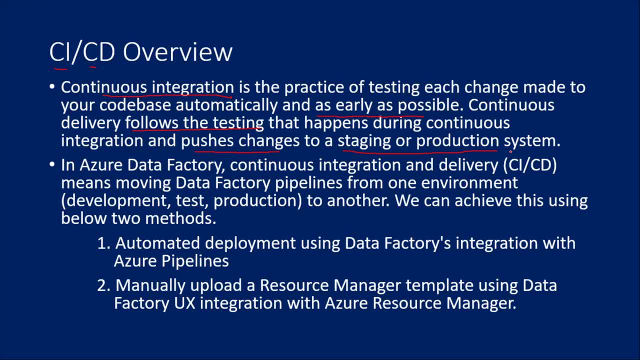 used to call it like continuous integration and continuous delivery. Everything should be in a automated way. So how to implement this continuous integration and continuous delivery in azure data factory and what it exactly means in azure data factory. In azure data factory, continuous integration and delivery means moving your data factory pipelines from one environment to another environment. 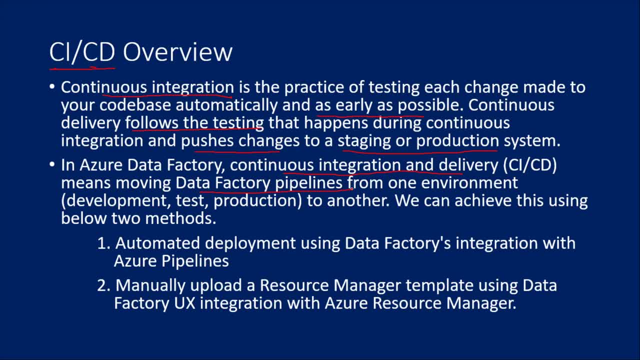 in an automated fashion. That means, let's assume you have a dev data factory and you have a UAT data factory and then you have a production data factory Now inside the dev data factory, if you have implemented any new pipelines there so that 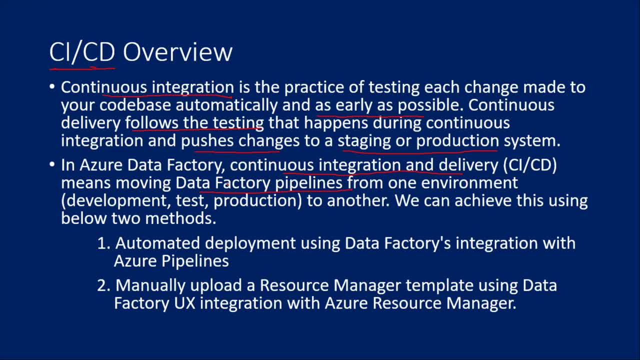 pipelines once you feel it is good and you have tested, fine. So what you want? you want to deploy them into the UAT data factory. to do that, if you don't have this continuous deployment concept, then you have to create the data factory pipelines once again inside. 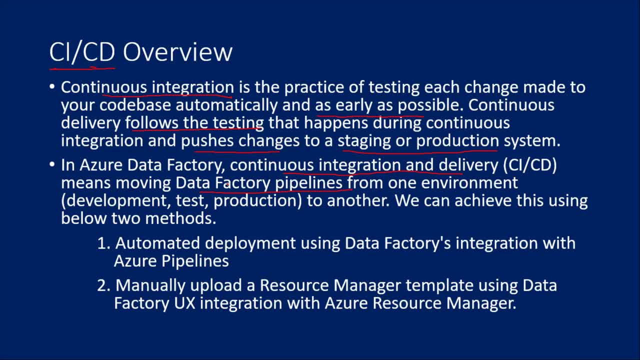 the UAT data factory. Okay, but using this continuous deployment concept, what you can do? define an automated release process which will take your pipelines from your dev environment to uat environment automatically and it will change the configurations. also, you can control everything. okay, don't worry all this. we are going to look that in a practical now. so this: 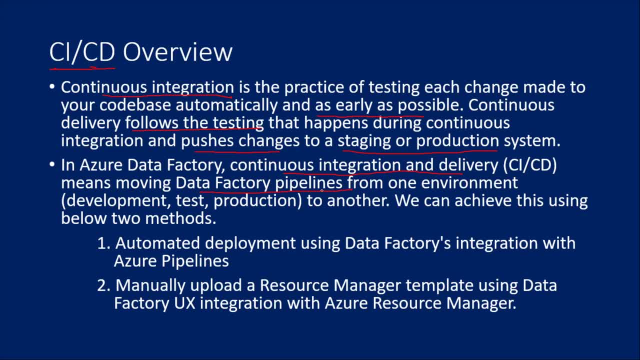 deployment of pipelines from one environment to another environment. it can be happened in two ways. one, as i said, using the automated deployment, by using azure pipelines. so inside azure devops there is something called azure pipelines where you can have your release plans and you can execute that release plans to deploy your changes. okay, so you can do that- or manually. 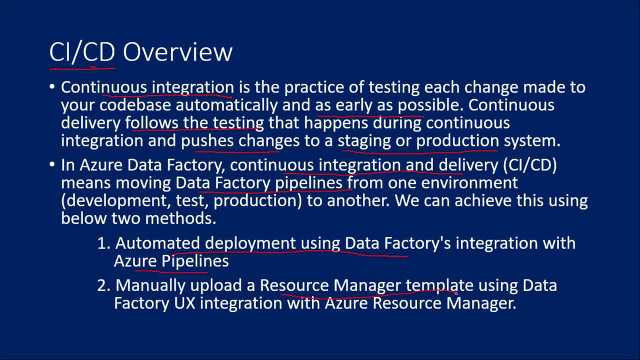 also you can do it. there is something called resource manager templates in the data factory so you can use them to manually create or to manually deploy. okay, so we are not going to look at this second approach. what we are going to look up at is the first approach. so this approach we 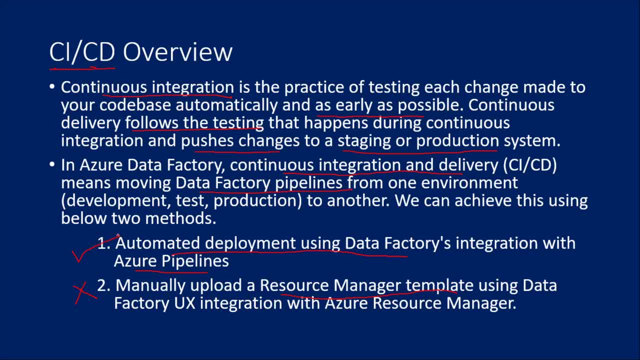 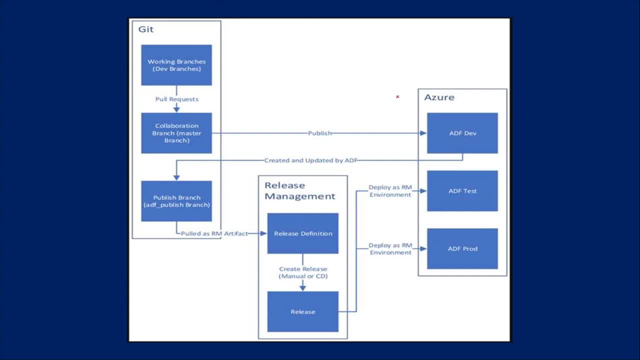 will call it like continuous delivery, sorry, continuous deployment. okay, so let me move back. let's go to the next slide. so this visual actually help you to understand how the process, the whole process, works. so let's assume you have three data factories: adf dev and adf test. let's assume this is the test environment- and then adf prod. that is the 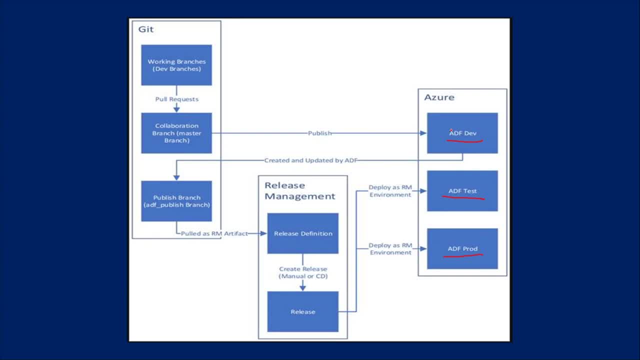 production environment. so adf stands for azure data factory. so now, in our past videos, we have already discussed about how to configure your adf with git repositories. right, you can configure your adf with github, or you can configure your adf with azure devops git. so we 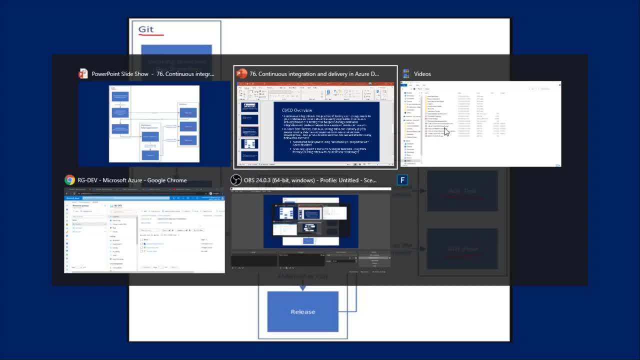 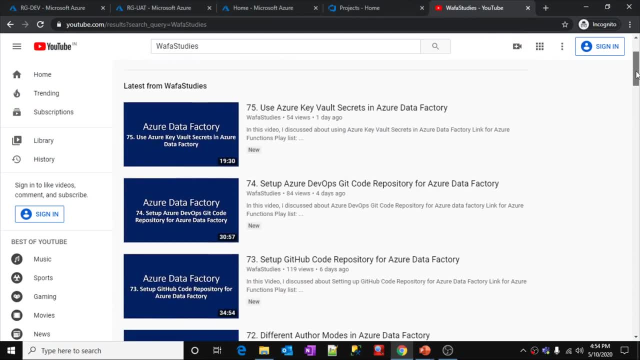 have already seen that in a practical, so please watch them in a practical or to understand them. so let me show you that if i go to browser inside my wafaa studies channel, right inside the azure data factory playlist itself, in part 73 i have discussed about how to set up a github code. 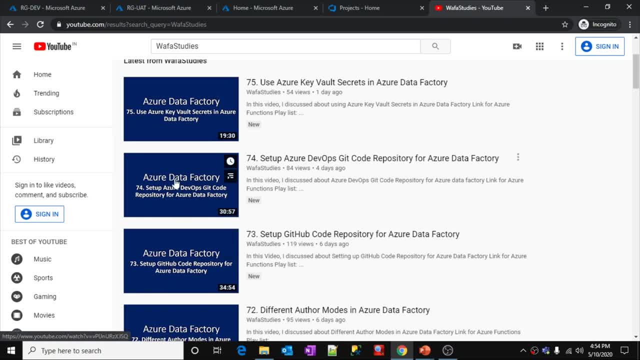 repository for your azure data factory. and in part 74, i have discussed about how to set up azure devops git code repository for your azure data factory. okay, so please watch these videos before watching this video. okay, because in these videos i have a detailedly explained how this entire cicd life. 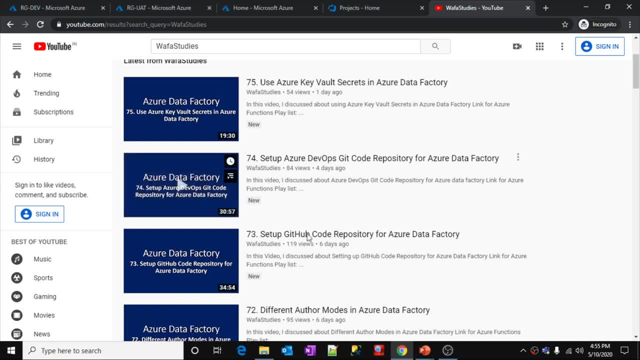 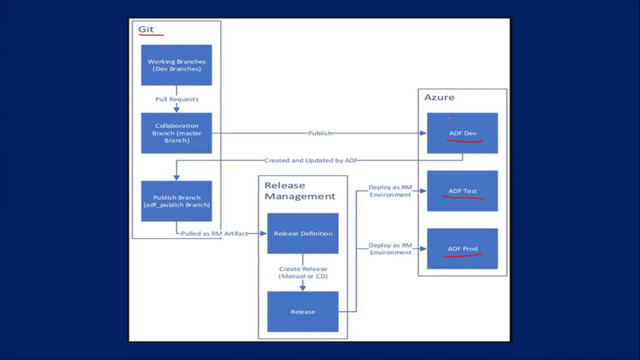 lifestyle will work. i mean, the life cycle will work. i have clearly explained here. okay, so let's go to presentation. but still, let me quickly explain here. so once you configure a code repository for your azure data factory, what will happen is you will be working on your changes in 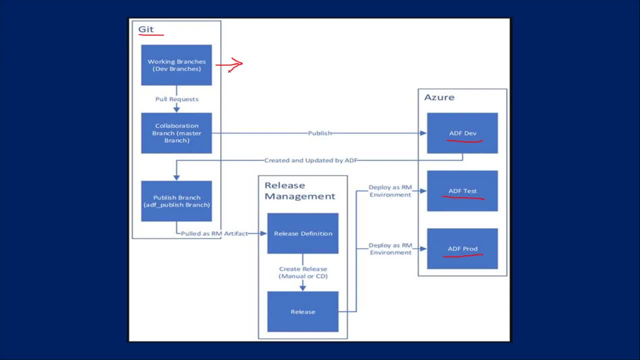 the future branches. right, so we will call these. future branches are nothing but working branches. so here it is saying: working branches, these working branches are nothing but future branches, as i said in my part 73 and 74 videos. okay, so developer will be developing their pipelines here. 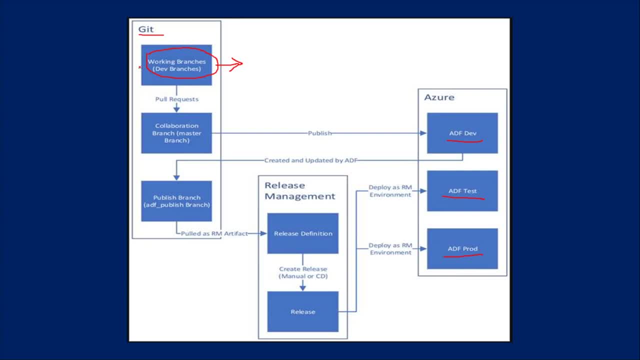 once he tests the pipeline, once he feel it is good what he has to do, he has to create a pull request. using the pull request he has to merge the changes, whatever he has implemented, into the collaboration bank branch. so usually master branch inside your repository is going to as a collaboration branch. 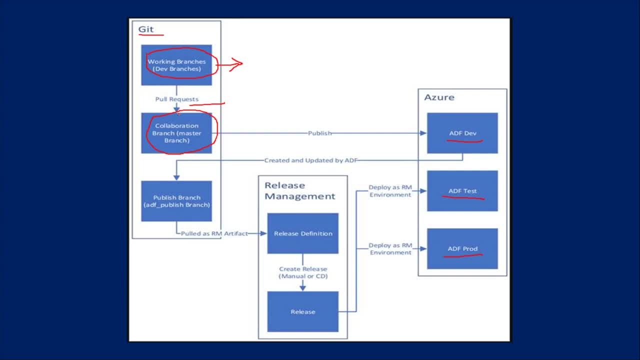 but it is totally up to you which brand, which, which branch you want to keep it as a collaboration branch. so it is purely developers decision. okay, but in real time usually people used to have the master branch as collaboration branch. so on, what is collaboration branch and what is worker branch? 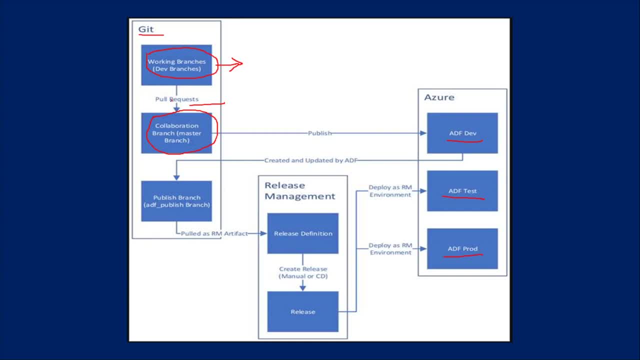 or future branch and what is pull request. everything i have discussed in my past video in detail in 73 and 74, so please check that. so once did happen, once me given a pull request and once you created a pull request and once you moved your changes to. 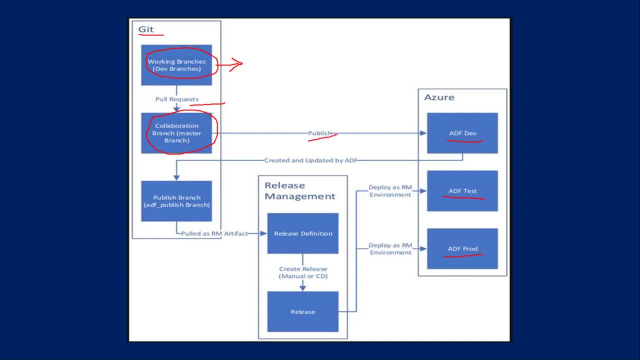 the collaboration branch, what people used to do. they will use to publish the changes into azure data factory service. so once they publish the changes, all changes will come into azure data factory. that means behind the scenes, what will happen is actually a new branch called adf. underscore publish will be created inside your repository and inside that branch, erm. 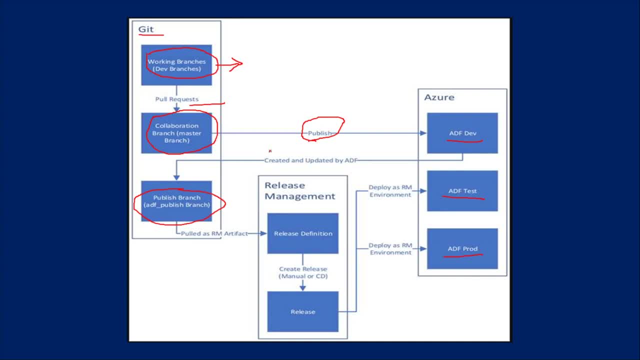 templates will be generated for your data factory and pipelines, okay, and the changes also will be for you in the azure data factory services. we have seen all this in practical in 73 and 74 right. so after that, how the continuous deployment approach will work is you you have to set up. 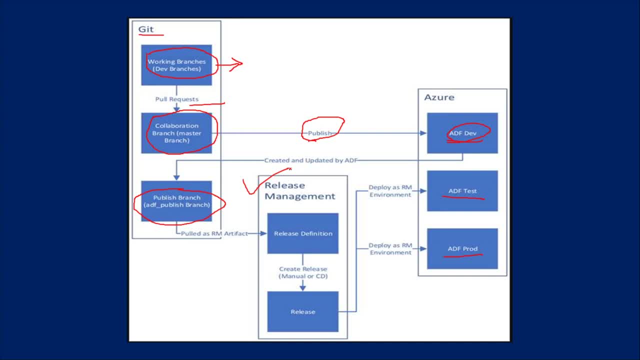 a release management system there using azure pipelines inside the azure devops. so you have to define the release there so you can define the steps. so once you define the step, you can schedule them or you can manually run them. so that is the automated approach actually. so using that, 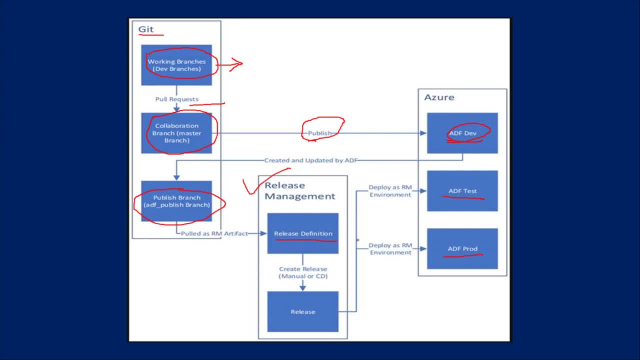 approach. what will happen is whenever you trigger that release, they are going to take the changes from this adf publish branch where you have the arm templates for your azure data factory and they will take that arm templates into adf test environment and also adf production. 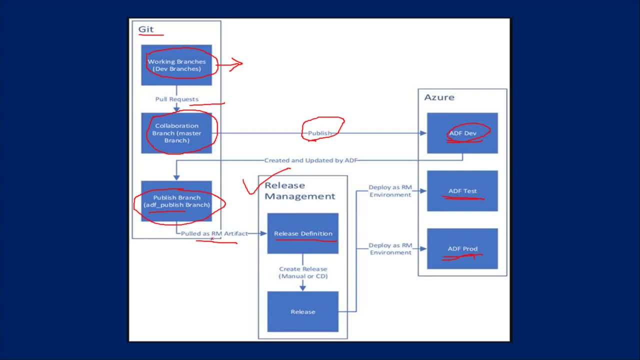 environment. whatever the environments you have configured, they will take them directly from here to here. okay, and everything will be. everything will happen in an automated fashion. you no need to do anything. the initially you need to set up a release management system, and then you need to set up a trigger there. so in that way it will work. so that means the deployment will be automated. 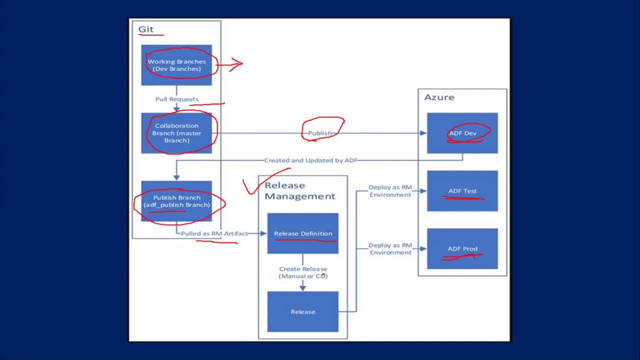 automatically right and also you can schedule. i mean you can have a triggers. that means whenever any publish happens, at that time this adf publish branch is going to update it right. so you can create a trigger there inside the release management which says whenever any uh changes. 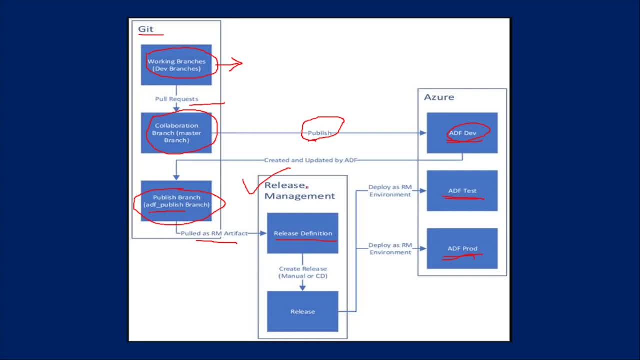 occur in this particular branch, then immediately take that changes and deploy them into adf test and adf production. you and you can do that okay. So don't worry all this approach of continuous deployment, what I am explaining here, because we are going to look at that in a practical implementation now. 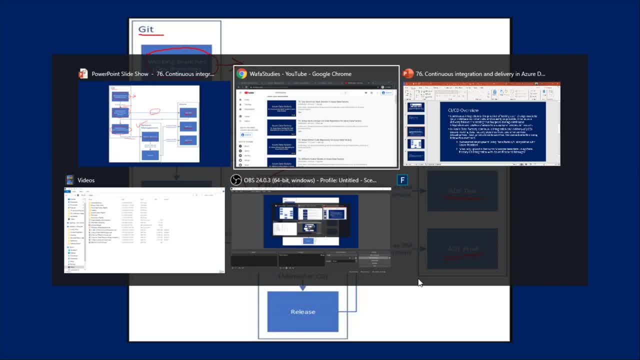 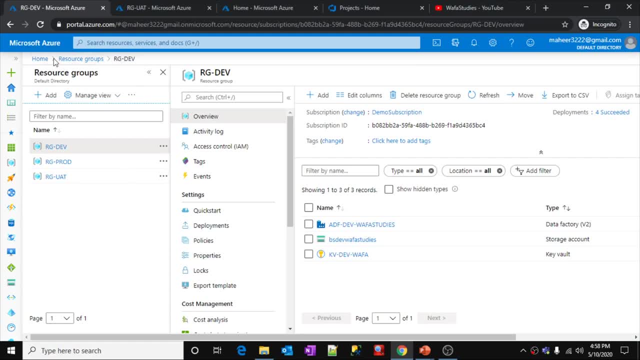 So now let's go to my azure portal first and let me explain you the requirement. So this is my azure portal. closely observe here. right now I am under resource groups. I am under resource group called rg-dev, right? see, these are the resources I have inside. 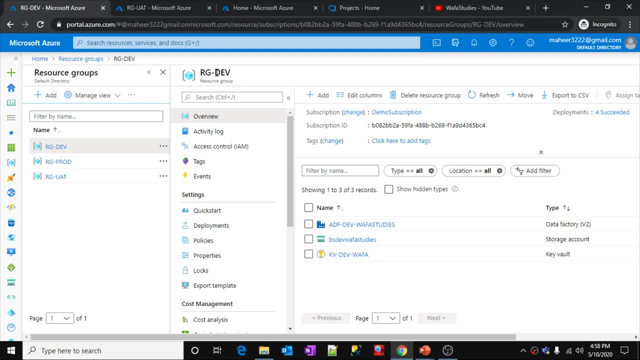 rg-dev. that means rg means resource group, dev means dev environment, let's assume. So I have three resources here: a data factory, a blob storage and a key vault. So inside this key vault I have a secret which actually store the connection string for this particular blob storage. 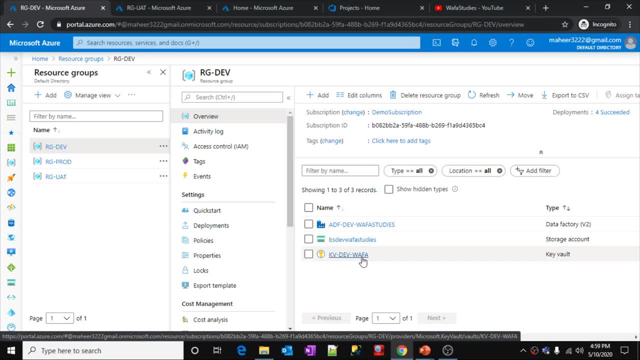 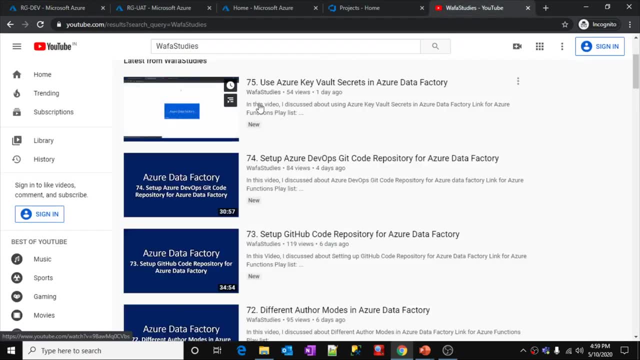 So how to store the, how to create a secret here and then how to use this key vault secrets inside your azure data factory- everything I have discussed in my part 75. So please watch that video also, Because that is also one of the prerequisite for me, so I am not going to explain all this. 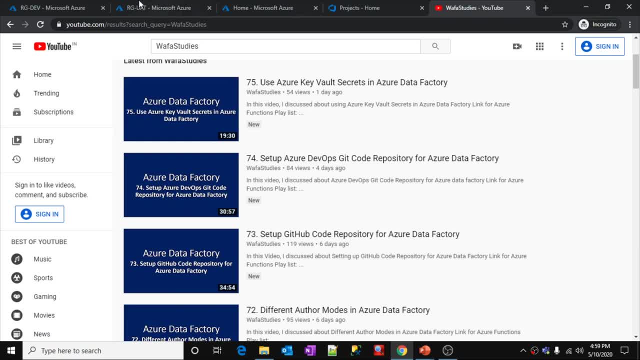 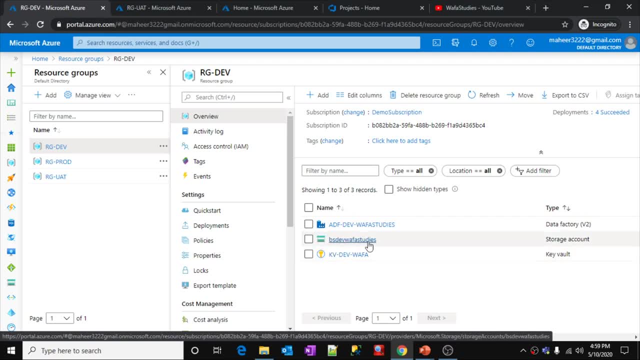 in detail, because I have already covered here with a lengthy videos, right, So let's go to our portal. So this key vault has a secret which actually holds connection string for this particular blob storage. okay, and there is a data factory called adf-dev-ofa-studies- okay. 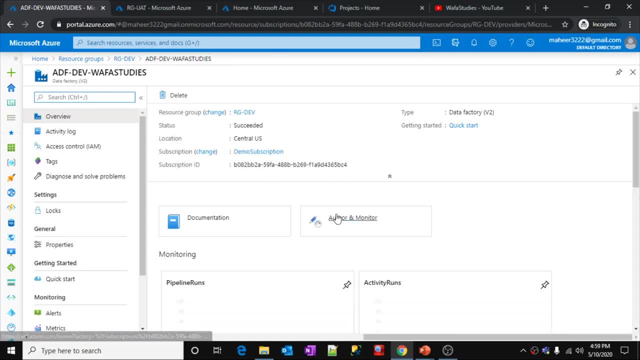 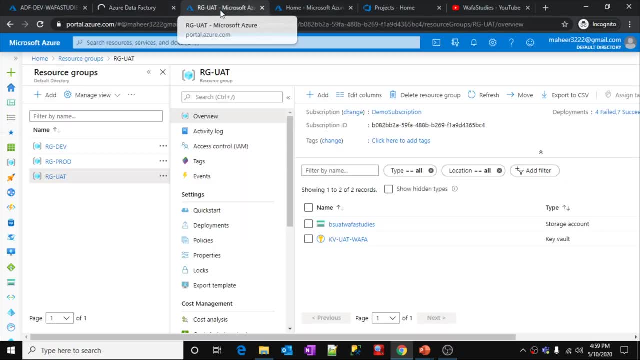 So let me open this data factory. let me click this author and monitor tile, which will open my data factory here. So my data factory, This is going to open now. so meanwhile, let me open another tab here. if you see, here right now I am under RGUAT. that means resource group UAT. this is the UAT resource group here also. 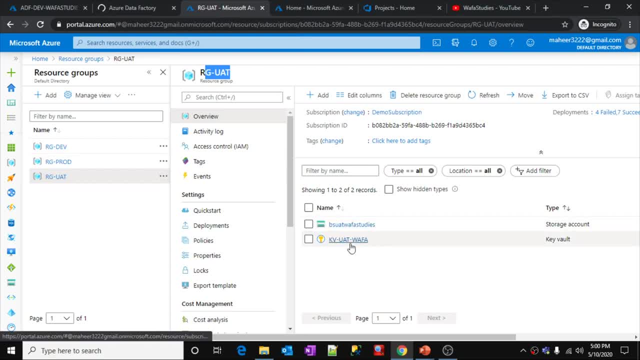 I have a blob storage and here also I have a key vault. So again in this key vault, I have a secret which will actually hold connection string for this blob storage. okay, So right now, what I want is here. here I want a data factory called adf-uat-ofa-studies. 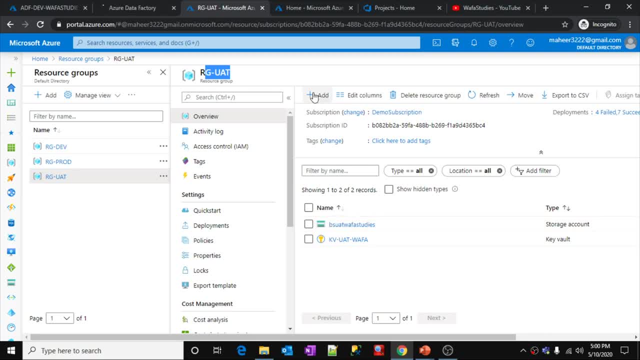 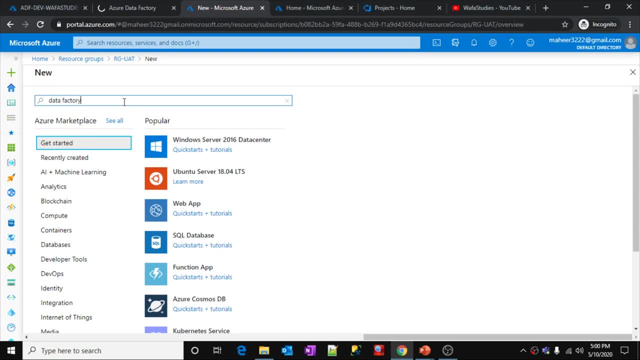 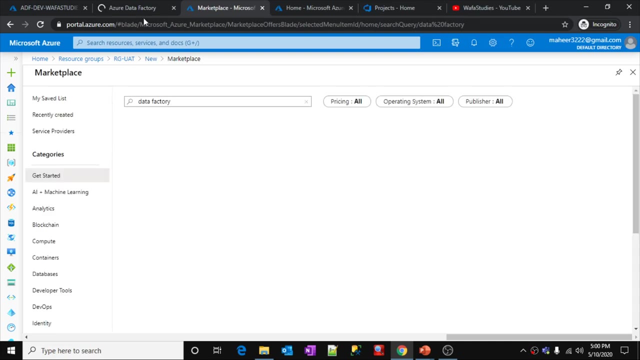 So why I want it, you will come to know in just a bit. Let me click this plus sign here and let me add a new data factory to UAT resource group. So let's say data factory. So I want to add that. So why I want to create it is because once I do any implementation in this dev data factory, 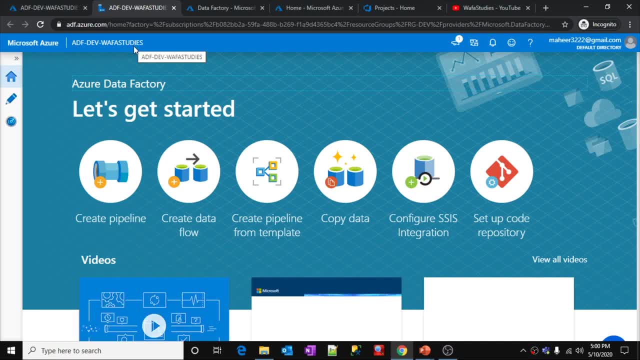 I am going to create a continuous deployment pipeline. that deployment pipeline will take the changes from this adf-dev-ofa-studies And it is going to deploy them into the UAT resource group. So let me click this plus sign here and let me add a new data factory to UAT resource group. 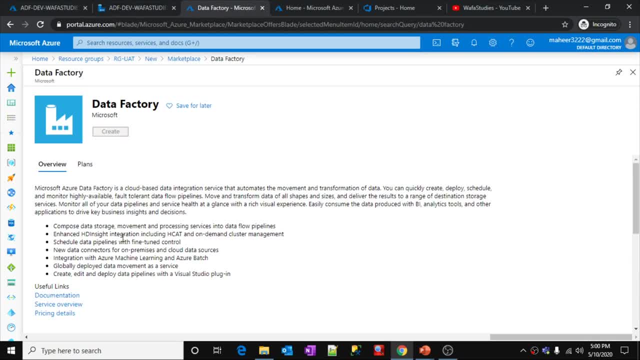 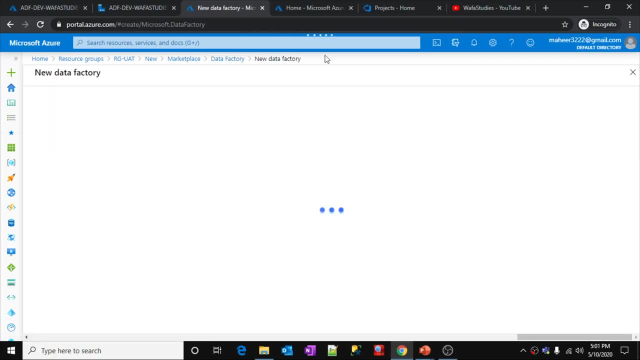 So let's say data factory, So let me add a new data factory in the UAT, which I am going to create now. So let me create a data factory here first. So I have clicked the create button, So it is going to ask me to enter these details. 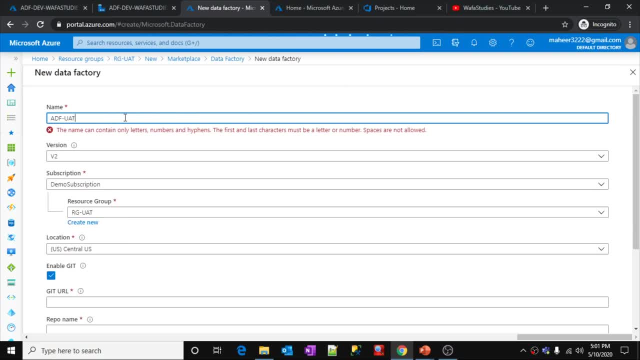 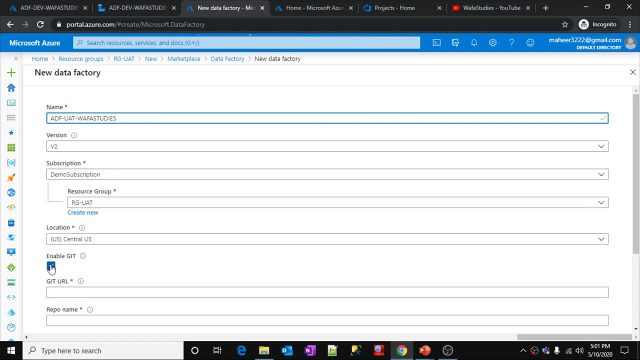 So let me say my data factory name is adf-uat-ofa-studies. This is my data factory name. resource group is fine. I don't want to enable git here. click create button here. So this is going to create a data factory for me, okay. 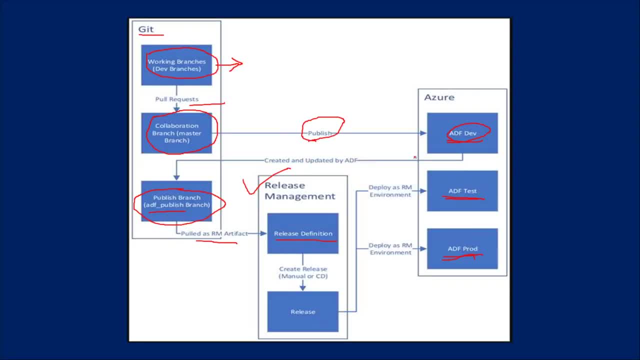 So let me go to presentation once again. Let me explain you that if you closely observe here, the test or UAT environment related data factory and also production related data factories are not connected with any git repository. Only the dev environment related data factory is connected with the git repository. 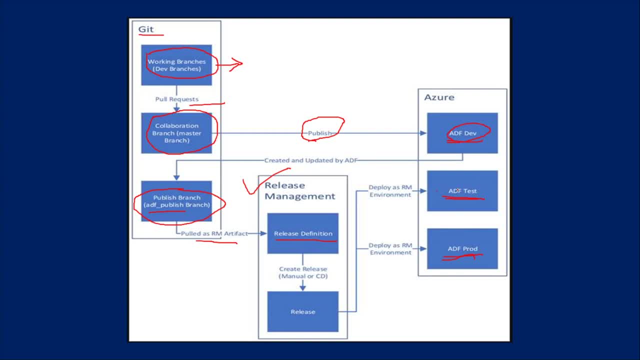 You are getting it right: all the changes from the dev data factory are getting deployed into test and production data factories using this release management system. right, okay, So this is the same approach we will. we will follow. So under this approach was the test and production data factories. 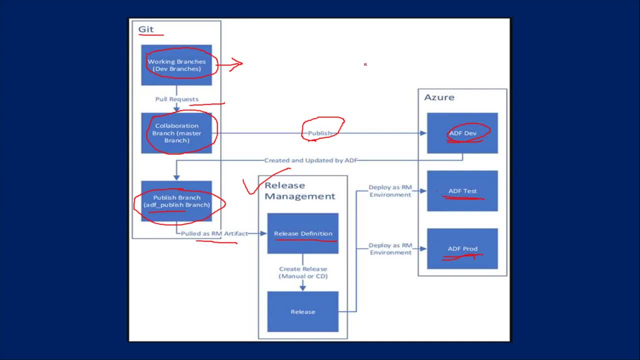 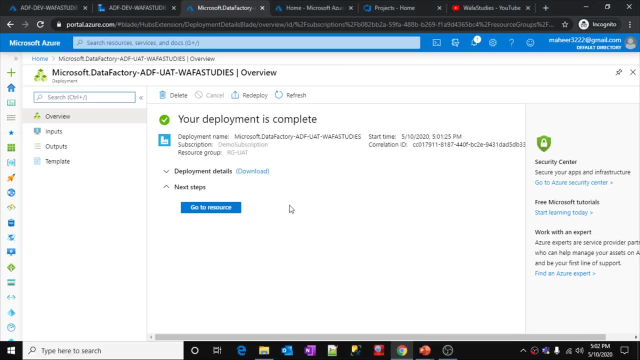 So this is the same approach we will. we will follow, Because the test and production data factory was suggested by Microsoft. okay, If you read the Microsoft official document, this is the approach they have suggested us. okay, So let's go to here. So my UAT data factory also got created here. that is fine. 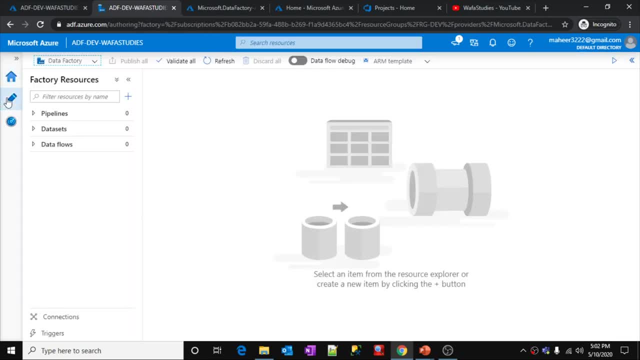 Let's go to our dev data factory. So right now, let me click this author tab here. So right now, I have nothing in this data factory. There is no pipeline, There is no data set, There is no data flow, Nothing, right. 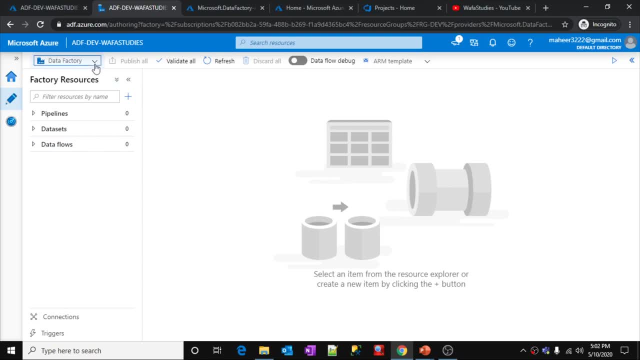 So now what I want to do First thing is I want to set up a code repository. So let's click this setup code repository. so this is going to ask you to select a core repository to setup, and all these things we have already discussed in my past videos. 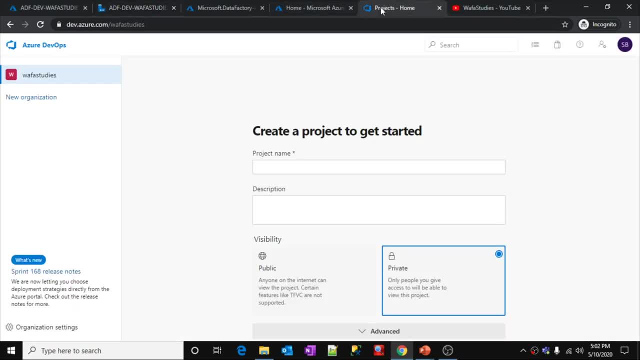 but let me show you one thing. let me go to my devops portal. this is my devops portal. let me quickly refresh this. so devazurecom slash wafastudies- this wafastudies is my organization name or my account name, so right now I don't have any project here. 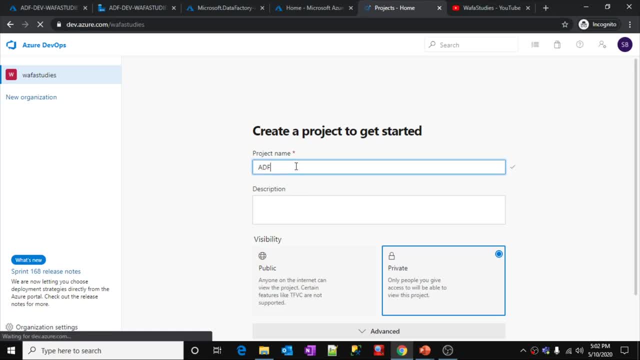 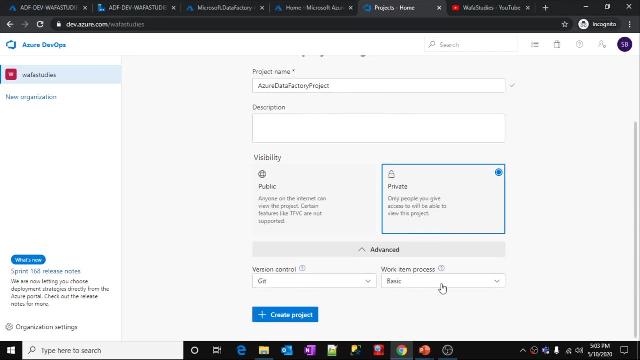 let me create a new project. my project name is maybe adf or azure data factory project. this is my project name, so let me scroll down here. let me click this advanced tab so I want the version control to be git. that is fine. basic work item process: fine. 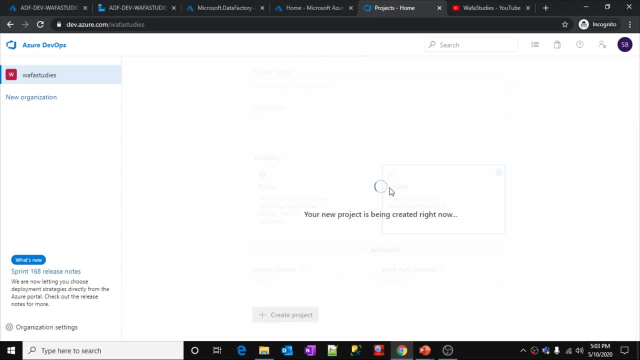 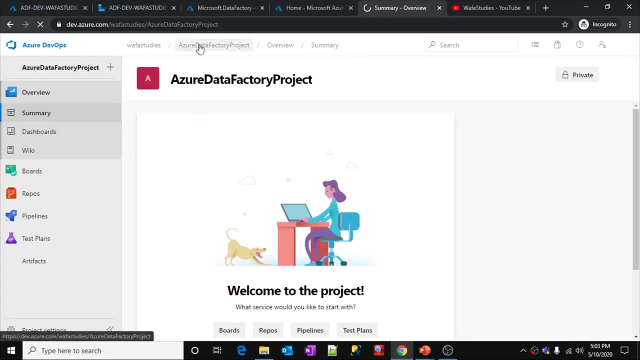 let me click this create project button. this is going to create a project for me and I have already discussed the hierarchy of project and repositories inside azure devops. so you will be having account first, then you will be having your project name. inside the project you will be having all these. 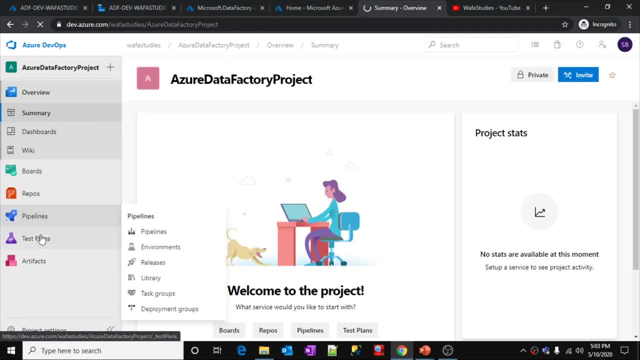 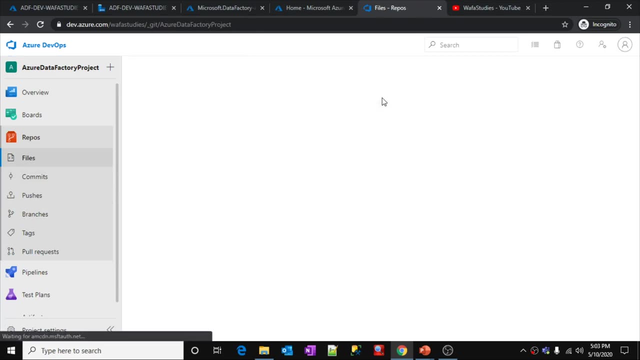 overview boards, repositories, pipelines, test plans, artifacts, everything. so whenever you create any project- in this case I have created azure data factory project- whenever you create any project, by default you will get a repository also with the same name. let me show you that. let me click this repos button here. 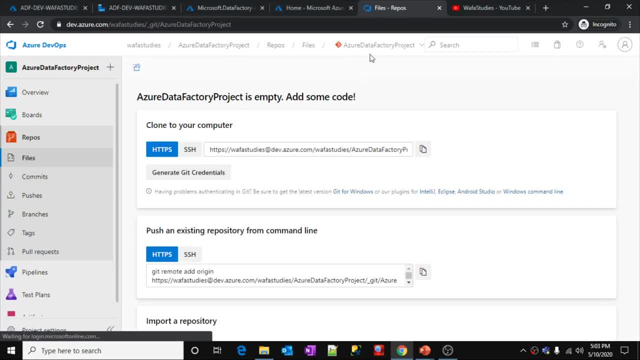 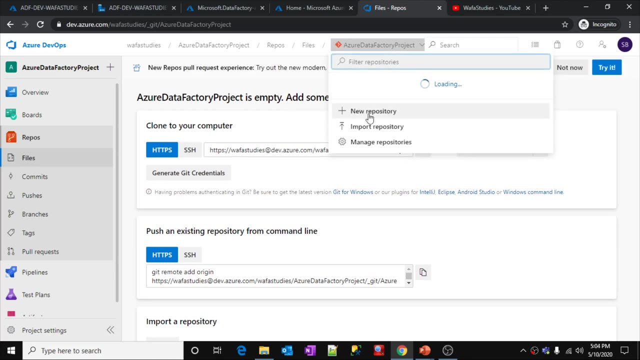 you can find that azure data factory project repo also there. you can see here this is wafastudies account- and then inside repositories, inside files. I have a repository called azure data factory project. click this drop down here and you can create a new repository also here. 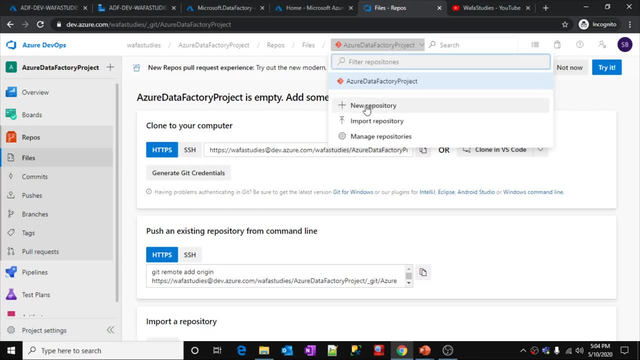 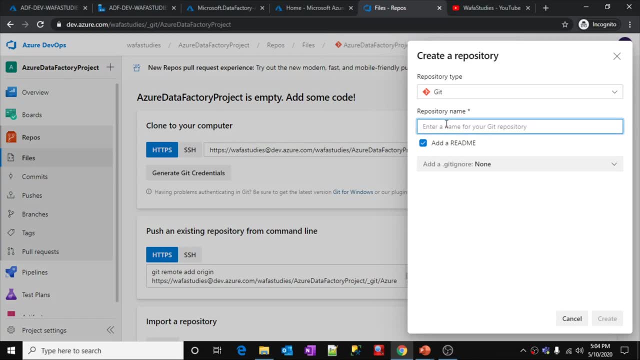 by clicking this, you can see there is already one repository. if you want to create a new one, you can create it. let me create a new one. let me click this new repository. so I want the repository name should be maybe ADF repo, ADF repo. this is the repository name. 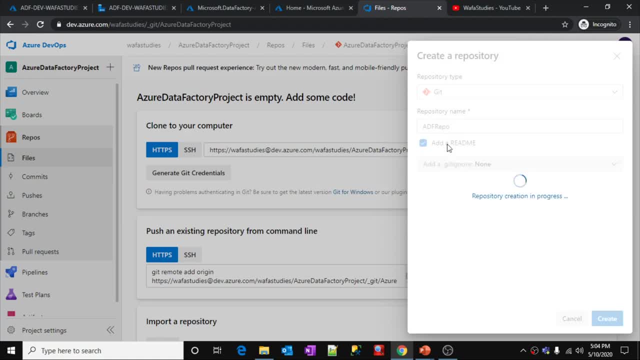 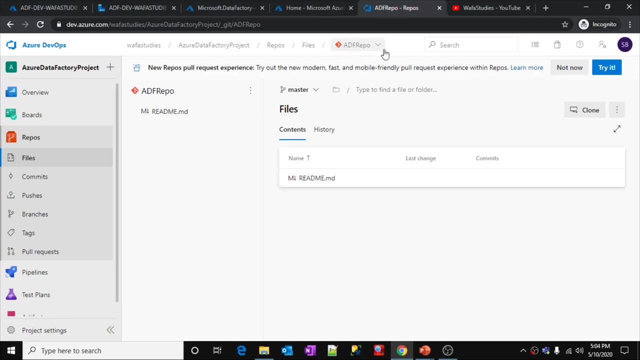 so click create button. this is going to create a new repository called ADF repo, so let's wait for the repository to get created. you can see ADF repo repository got created. you can see there is one branch, also master branch. let me click this drop down button here. 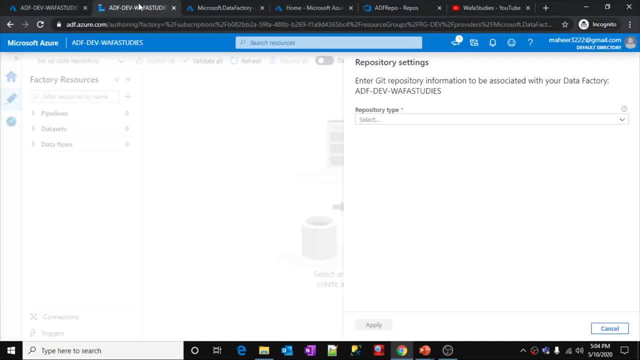 right now we have only one branch, which is a default one, so that is fine. let's go to our data factory. here let's select the repository, trypass azure devops, git. then here you need to select your account and then you need to select your project. 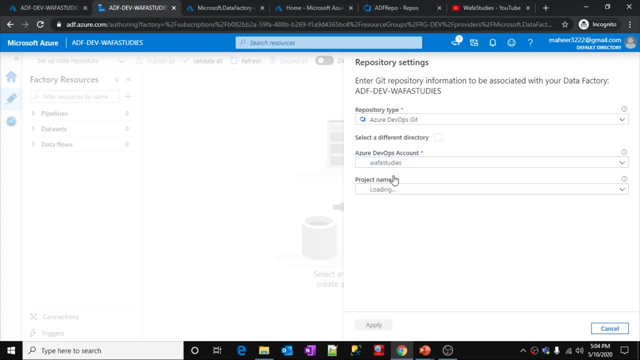 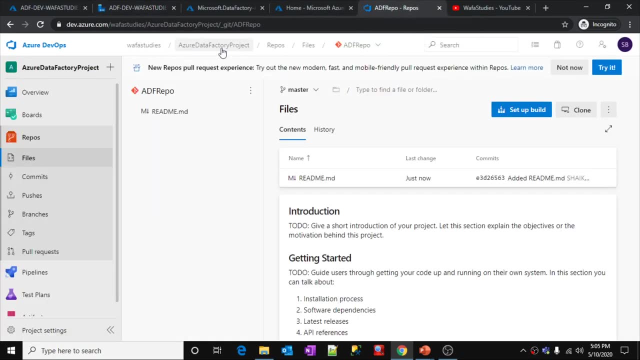 and then you need to select your repository. let me select my devops account, wafa studies. that is the account name, right, as I said here. if you see here wafa studies, right, then project name is azure data factory. project repository name is ADF repo. let me select all these values. 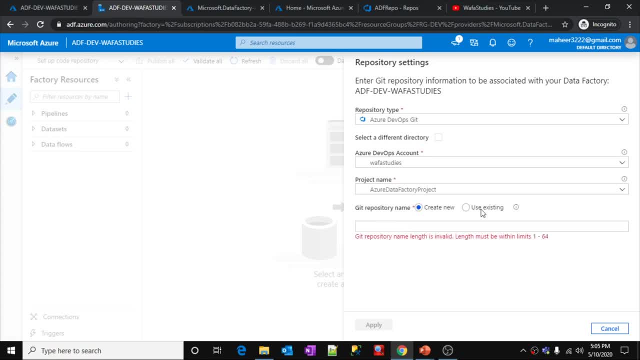 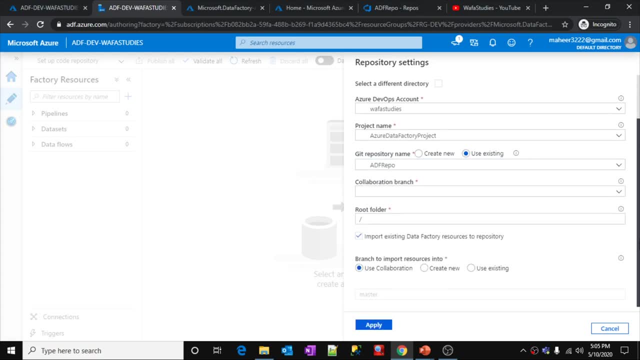 so the project name is azure data factory project. that is good. the repository name: let me use existing. I have a repository called ADF repo. I want to use this repository, so that is fine. the collaboration branch: so, as I said, usually people will have master branch as a collaboration branch. 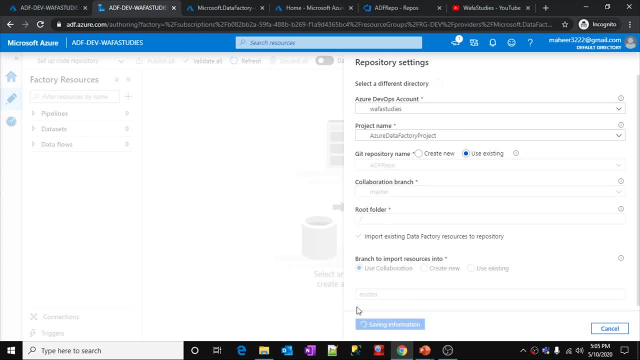 so that is fine. let me click this apply button. so this is going to configure azure devops git repository for my data factory. this is the dev data factory. remember all of this happening on the ADF: dev wafa studies data factory right. so why I am doing all this? 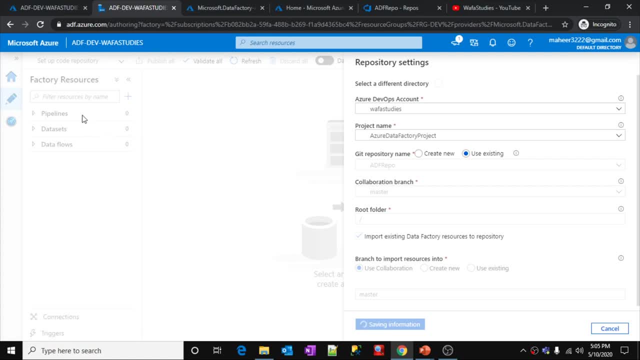 because once I set up this core repository, I am going to implement few changes here and then I am going to deploy that changes into azure data factory. so once I publish them, after that I will be going into azure devops portal and I will be creating a deployment plan. 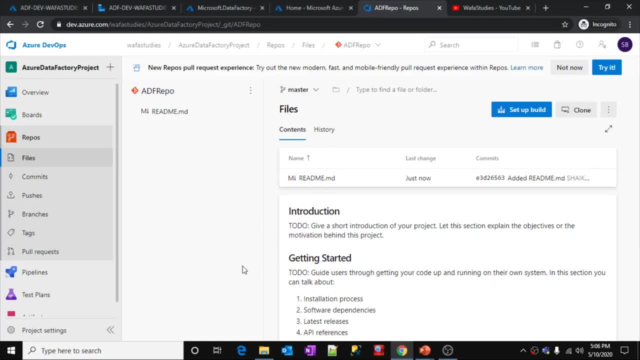 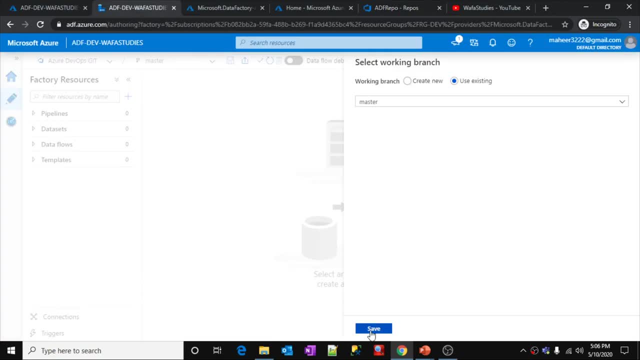 automated deployment plan then. so there, what the deployment or release plan will do is it is actually take the changes, whatever I implement here, into UAT data factory also. ok, so let me show you all that in a practical demo now. so I have clicked save button, so right now you can see I am at a master branch. usually people. what they will do is they will create a new branch called future branch, and on that new branch they will implement the changes and then they will create a pull request to merge the changes with the master branch. after then only they will publish the changes. that's what usually people will do. 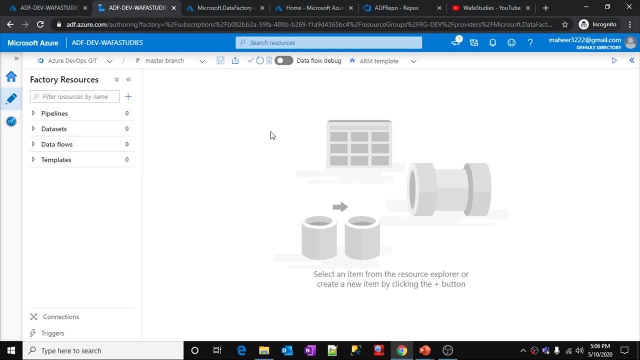 but now what I want to do is: I am not going to do all that. I will be directly implementing changes in the master branch for time being. so let me create a new pipeline. so let's say: this is pipeline 1, this is the pipeline. so now what I want to do is: 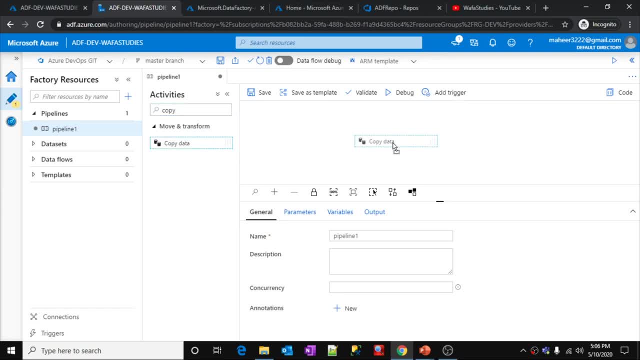 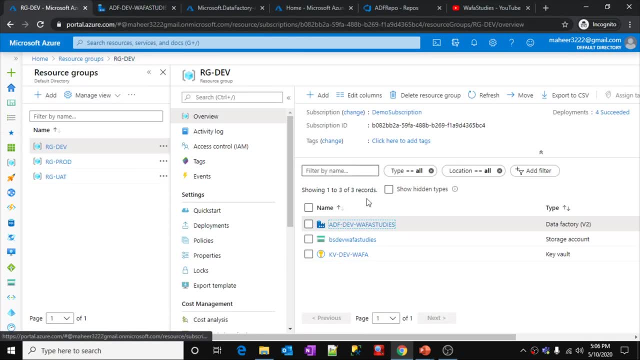 let's assume I want to perform a copy activity. ok, so what I want to do this is the dev environment. let me go to my dev resource group once again. see. my requirement is this one. so I have a blob storage in each environment. what I want. let me open this blob storage. 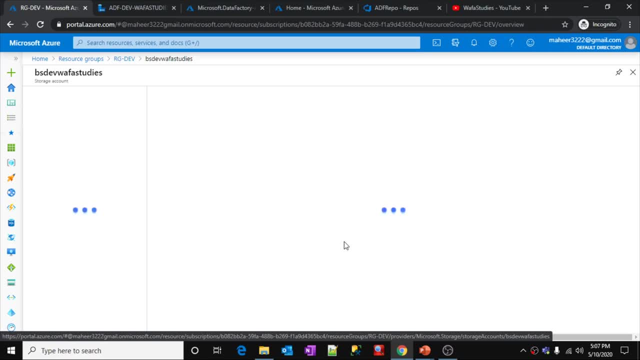 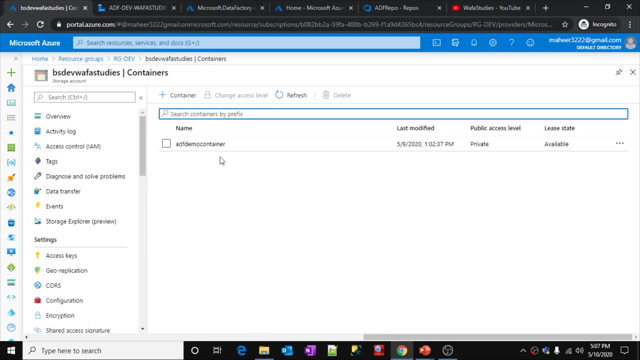 inside this blob storage I have a container called ADF demo. let me open that and show you. and there is an input folder also. let me click this containers button here, which will actually open ADF demo container. this is the container name. let me open a container. 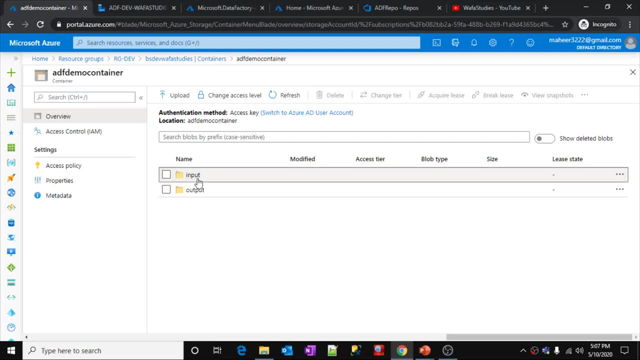 ok, see here I have an input folder. inside this input folder I have a file called employeecsv. I want to copy this file from input folder to from input folder to output folder maybe. so inside the output folder right now I have already employeecsv file. let me delete this file here. 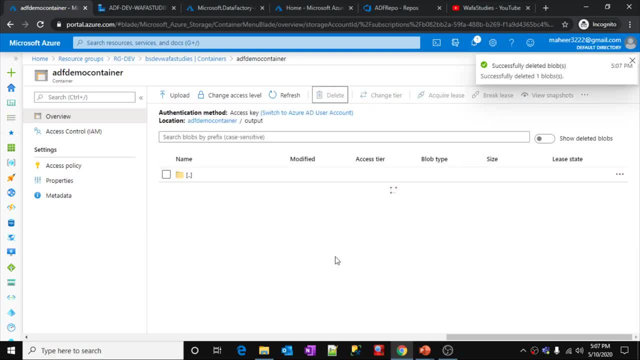 why? because I want to copy that freshly, right so to make you better understand. I am deleting this. even though I don't delete, nothing will happen. actually, it will overwrite the file. that's fine, we deleted it. so let's go back to our container. right now I will be having only input folder. 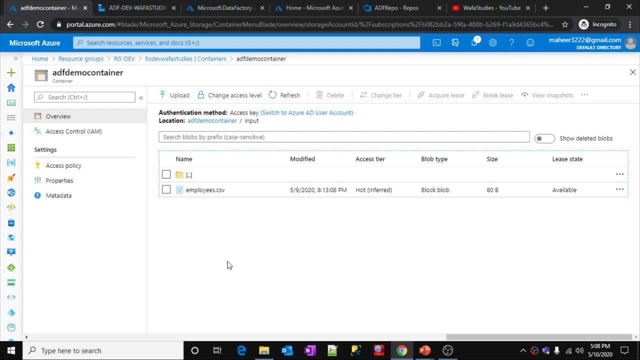 so I want to take that employee file from there and I want to move it into output folder, so output folder will be automatically generated for us if the folder is missing. so no worries. so this is what I want to do it. so let's go to our dev data factory. 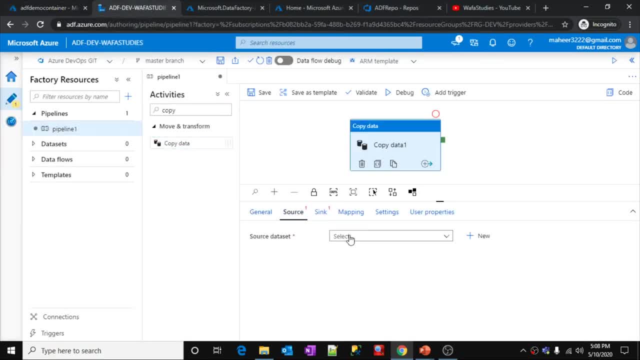 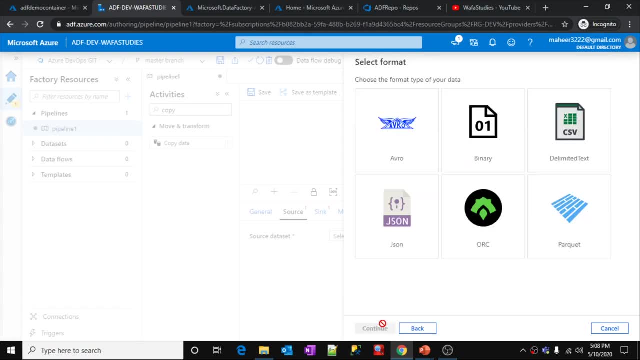 so I have a copy activity. so I need to have a dataset for my input folder- employee file. so let's create a new dataset. so blob storage. click on continue. this is going to be the csv file. click on continue. so first row is header. that is fine. 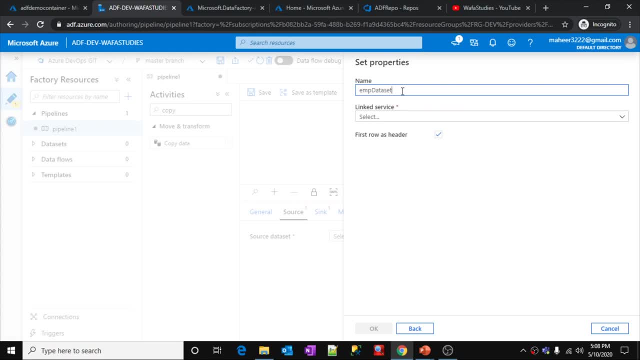 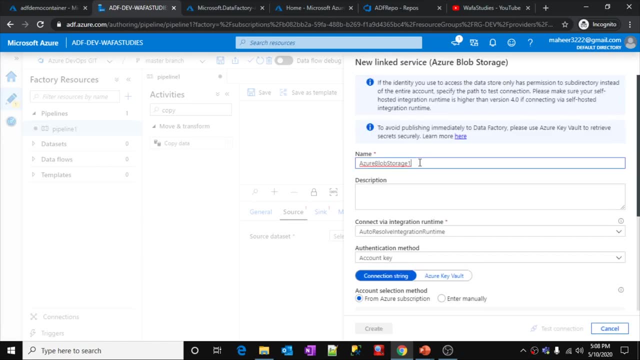 so let me give a name for this dataset. this is maybe emp dataset. this is the name. now I should have a linked service for my blob storage, so let me create new button here. so this is linked service for blob storage, right? so this is what I am going to use. 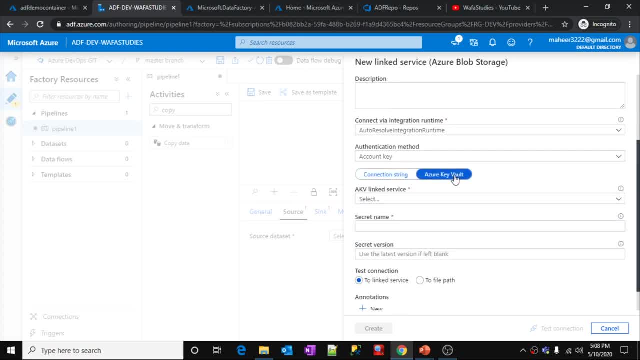 here. right, I am not going to use the connection string, I am going to use a key vault. why? because key vault is the secured way. you no need to have your credentials saved somewhere. and also I am going to deploy whatever the changes here I am implementing. I am going to deploy them into ued data factory. 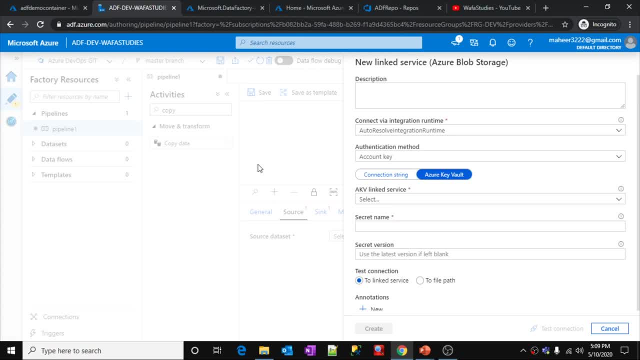 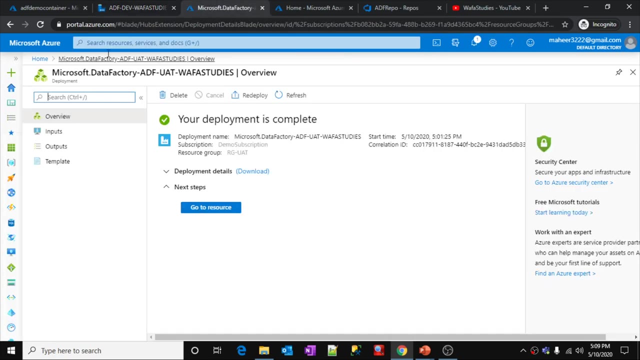 from azure devops, azure pipelines, using the release management system. so when you are implementing such approach for the continuous deployment, it is best way to use the key vaults. why? because I am going to change for ued environment. because if you go here, let me go back to my home. 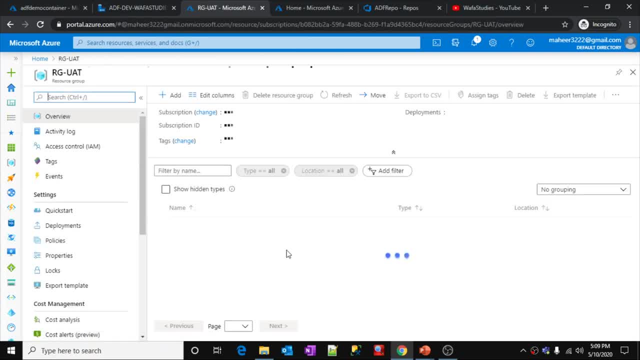 and let me go back to ued resource group, the same pipeline. in case of ued, what it should do is actually it should take the file from the ued blob storage. see, I have a ued blob storage and connection string for this blob storage is available in the ued key vault. 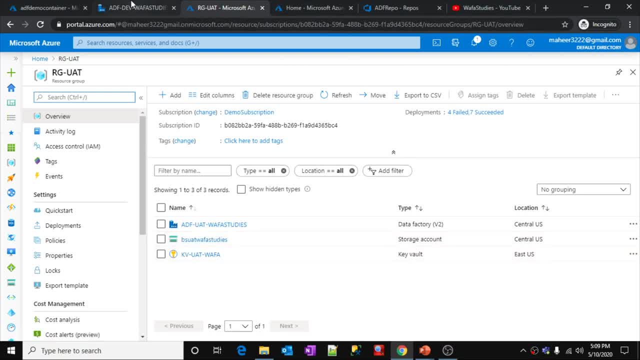 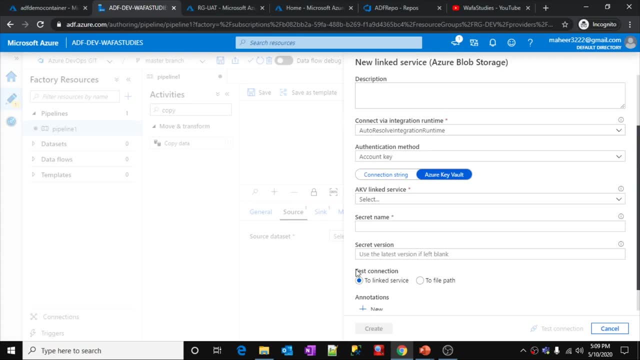 so automatically this copy activity and this linked services and also datasets, everything has to point to ued automatically when you deploy these changes to the ued. that's what my need. so in ued environment I should not refer dev related resources. I should refer ued resources only. 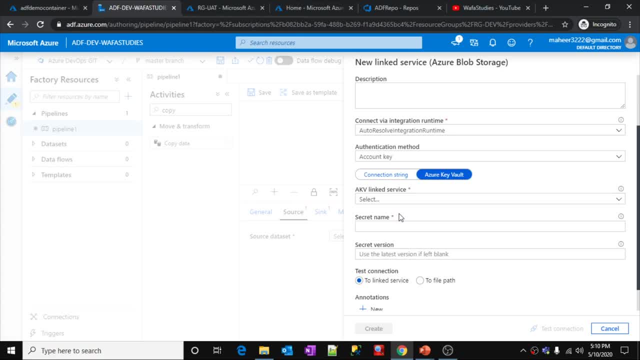 so to handle that everything properly, when you are continuously deploying using that release management system, you should use the key vault. that is the best way. so how it is going to be helpful for you. don't worry, you will come to know that in just a moment after completing few steps here. 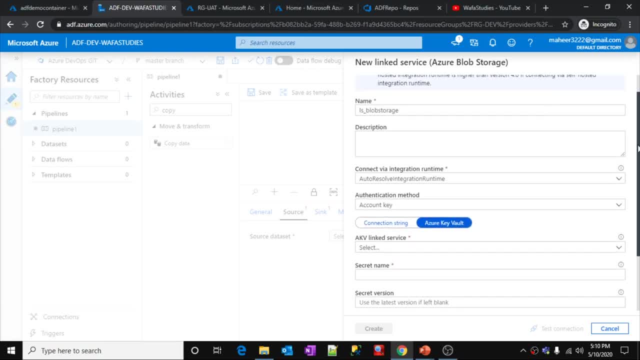 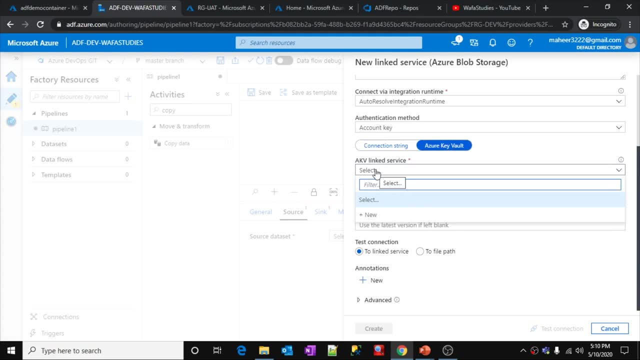 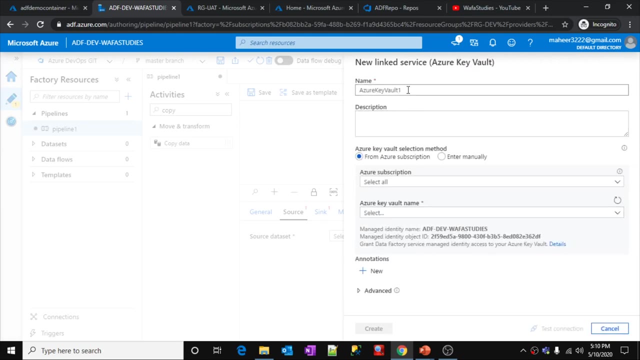 so I am using azure key vault. I have given a name for my blob storage: ls: linked service, blob storage. fine, so here I need to select the linked service. sorry, key vault linked service. so for my key vault I should create a new linked service. first click this new button here. 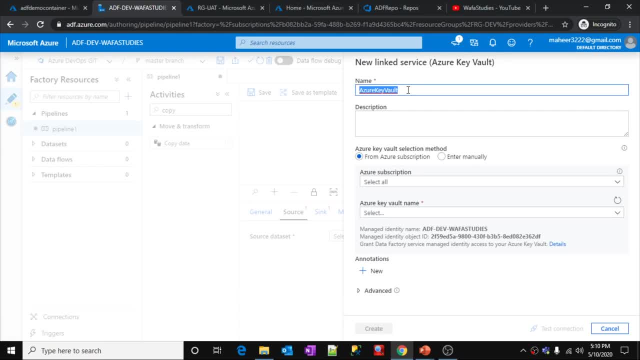 so this is azure key vault. so let me give a name. maybe key vault means kv underscore, sorry, linked service, right, so let's append with ls key vault. so this is what I want to keep it name: linked service, key vault. so now here from this subscription and what is the key vault name? 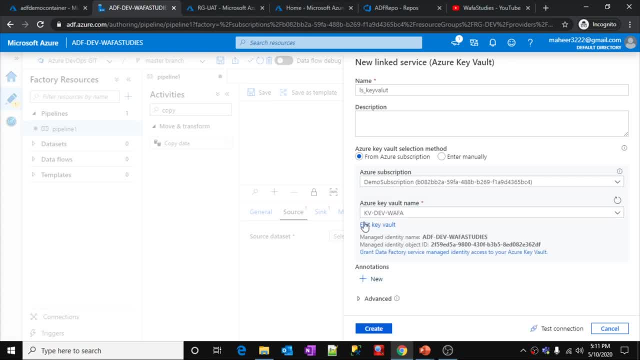 so this is dev environment. I am going to select the dev key vault: kv, dev wafa. that is the dev key vault name, so I selected that. let's click this test connection, which will actually test the connection: whether you are successfully able to create your connection or not. 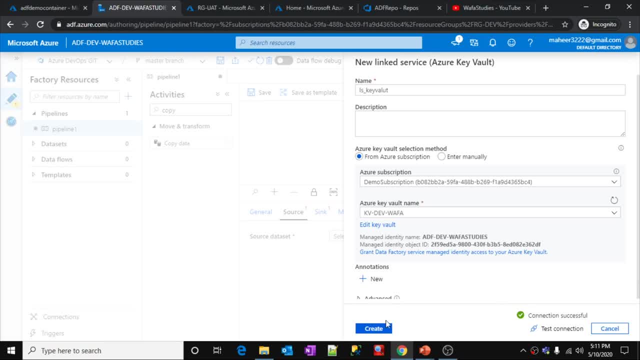 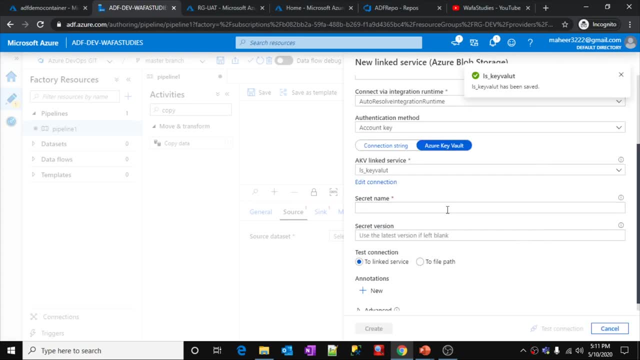 ok, so let's wait for couple of seconds. so test connection was successful. click this create button, which is actually going to create a linked service for your key vault first. ok, so your linked service for key vault got created and this is where it is automatically selected. now you need to provide the secret name from the key vault. 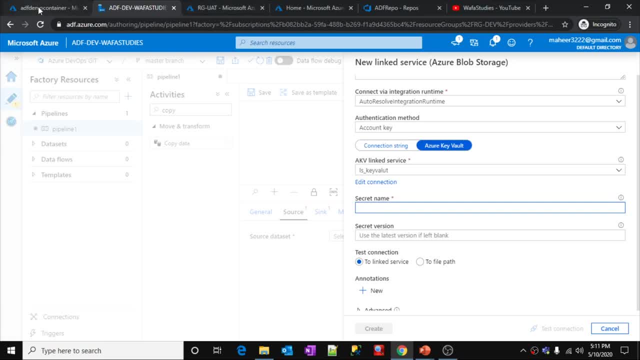 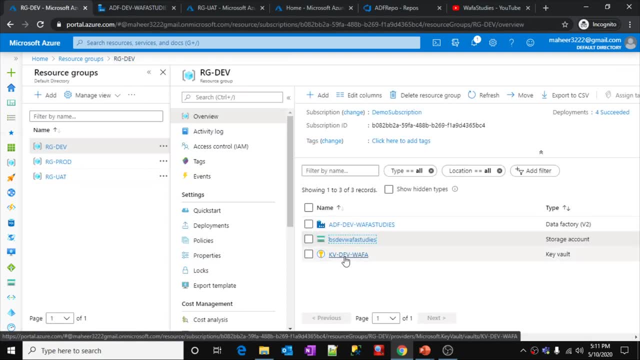 where you have connection string for your dev blob storage. so let me go to my dev. this is the dev blob storage. so let me go to my resource group. so inside the key vault kv dev wafa, let me open this key vault. so let me copy the secret name from there. 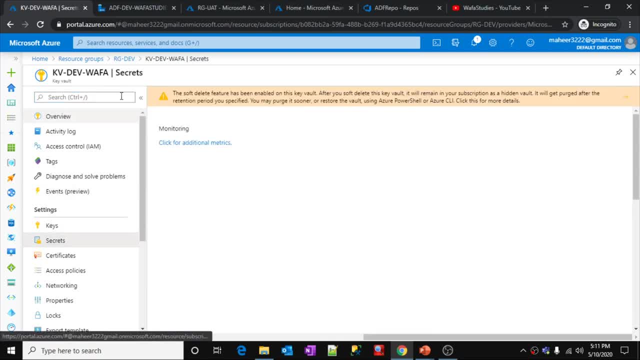 ok, so let me go to secrets. I have already discussed everything: how to create these secrets and how to save them here, everything I have discussed in my past video, and also you need to provide some access policies there. I did that already. I have already discussed in part 75. 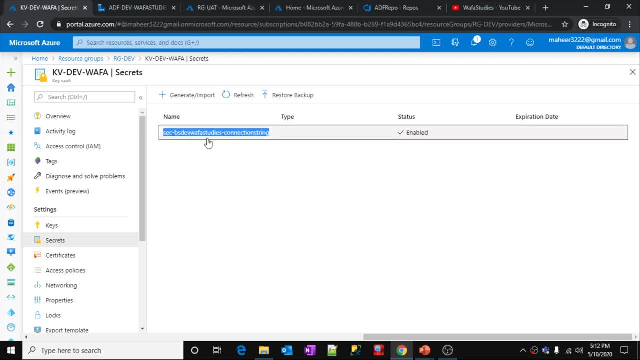 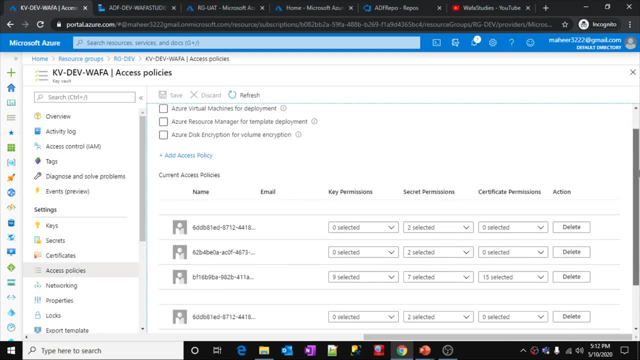 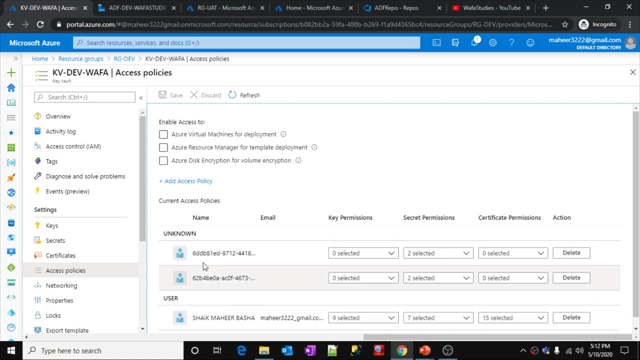 so that is the reason I will recommend to watch part 75 before watching this. so I am copying my key vault name. sorry, my secret name. let me show you one more thing under access policies. if you see here, one second, if you see here, all these values are coming. 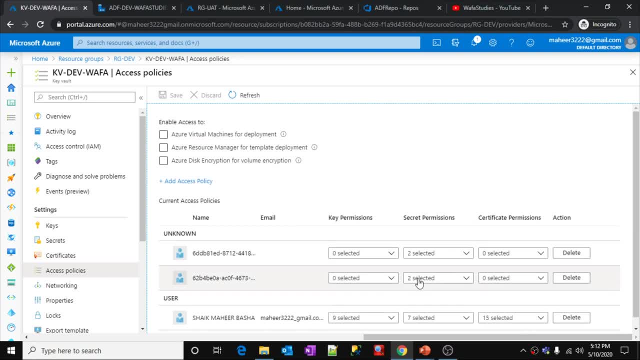 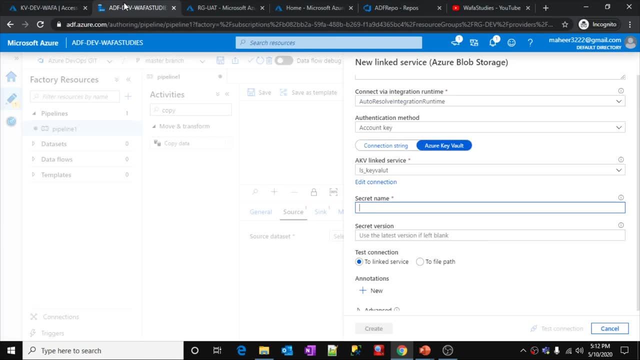 actually all these are coming why? because I have added here, if you see, here under secret permissions I have added get and list secret permissions for this data factory, azure dev wafa studies data factory. so I did that in my part 75. that is the reason you can see. 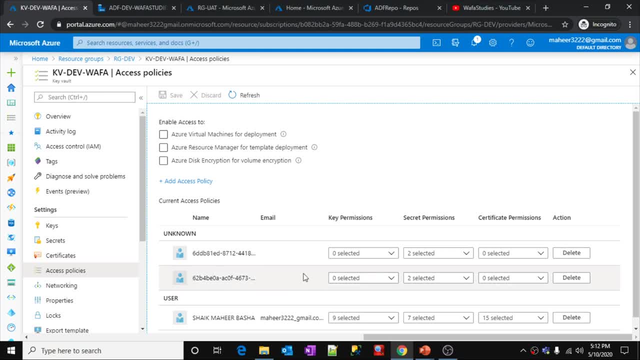 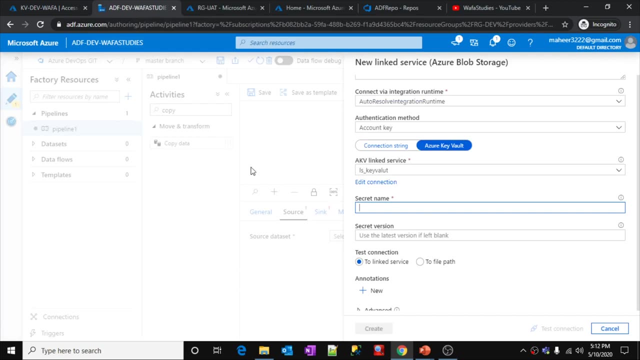 this entry here, so please watch that video how this entry came. this entry should be there. if this is not there, your data factory will not be able to access your secret. if your data factory wants to access your key vault, what should be there is for every data factory when you create it. 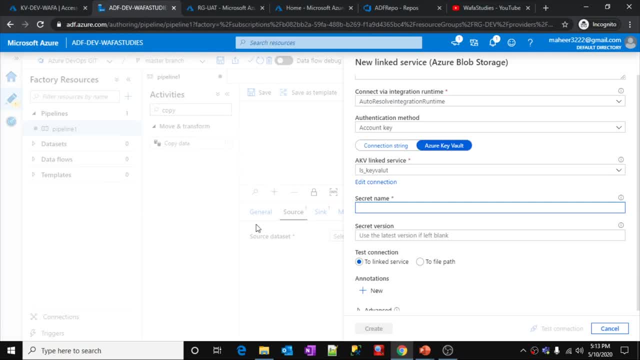 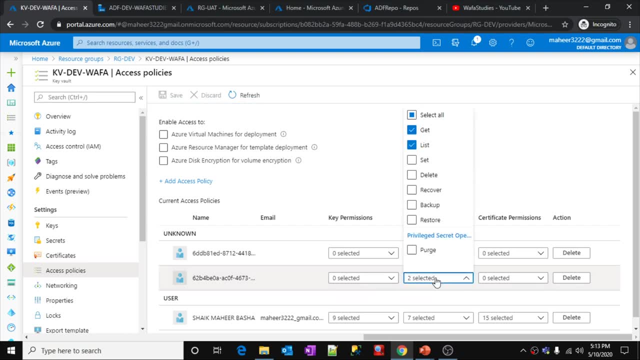 there will be a MSI created behind the scenes. MSI means managed service identity. it will be created automatically. so for that managed service identity, you need to add this: secret permissions, get and list. then only your data factory will be able to access the secrets. so that I have already did it. 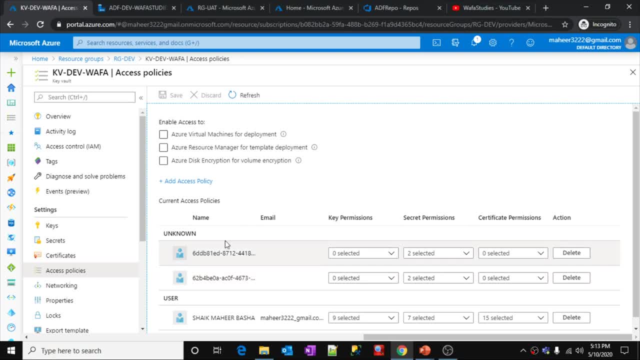 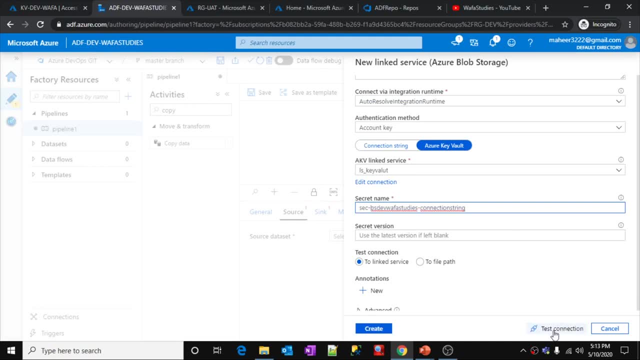 this entry is appearing here so I am not going to repeat that. so please watch my part 75 video to understand that. so let me go to my azure data factory, let me place this secret value here now, let me click this test connection. so if I would have not done, 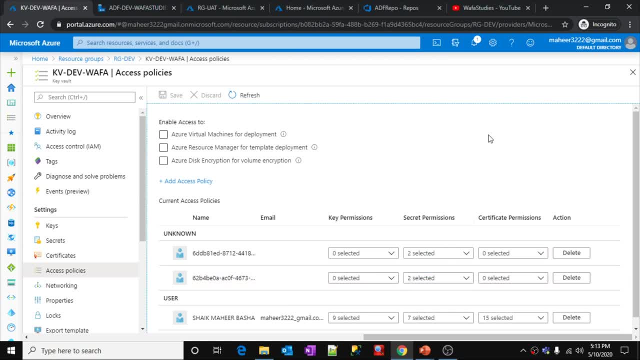 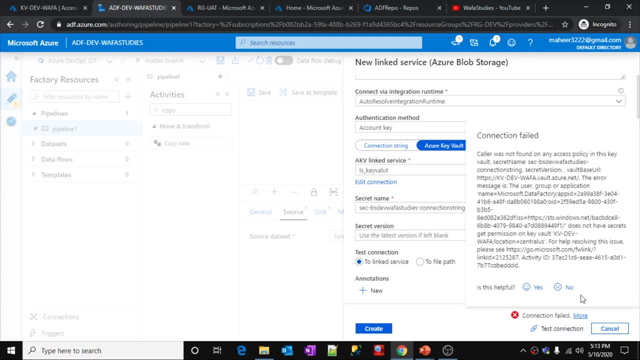 this entry right. access policy entry for secret permissions, get and list. then here: right, the test connection is going to fail. ok, it looks. my test connection is going to fail. ok, it is saying access policy is missing. ok, don't worry. I think this is the new data factory I created. 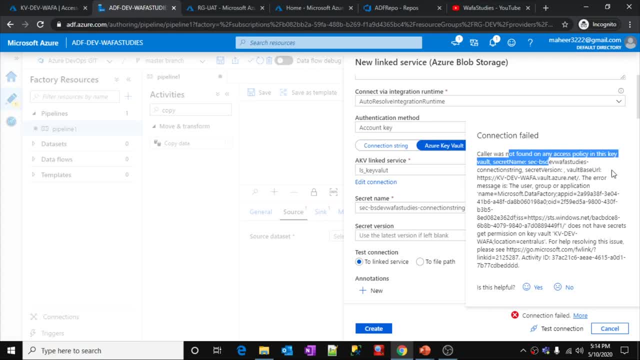 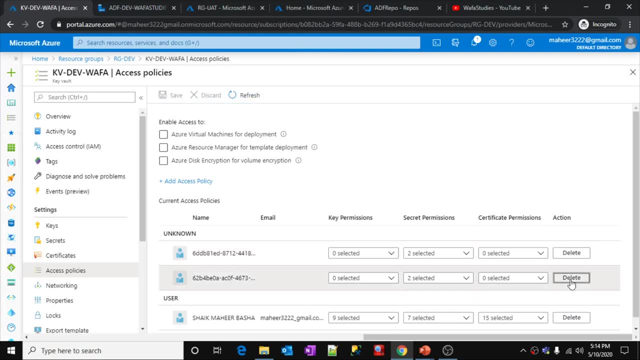 ok, that is the reason that access policy is not there on my key vault, so that is good for us. no problem, we will create them, so let's go here. let me delete these two. these are for whole data factories. I have created that. I have deleted those data factories, so let me delete. 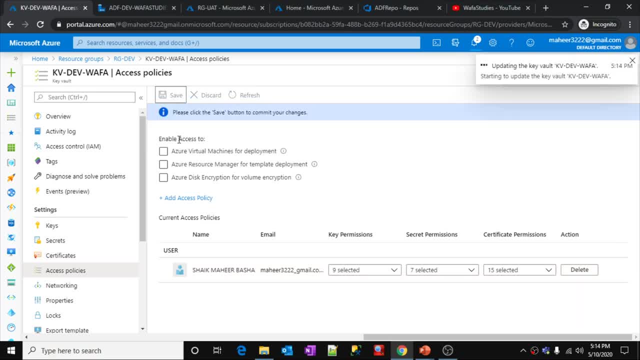 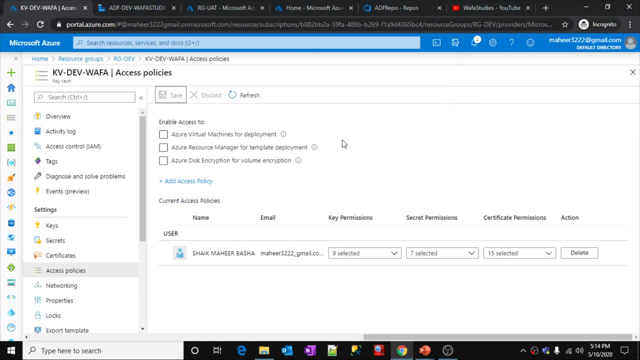 all those. let me save it first. let me save that. so now what I want to do for this data factory: I should add the access on this key vault, especially for the secrets. that is what I should do. right, let me click this. add access policy. so you need to click that. 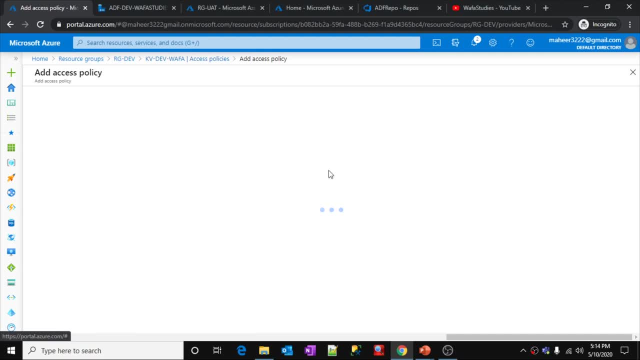 add access policy to do that. ok, so let's wait for the screen to load. it will take few seconds. so here, right under secret permissions, you should select this: get and list. ok, so I am good. then click this: select service, select principal. ok, so this is where you need to actually search. 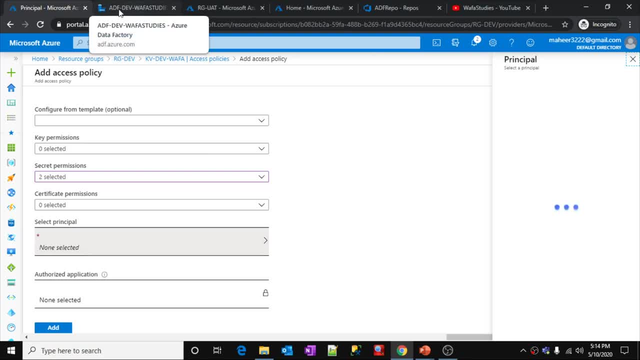 your msi, the data factory related msi service identity. ok, so let's wait for the screen to load. so how to search that? it is very easy. you need to type your data factory name, because your msi is going to have the same name, so just type. 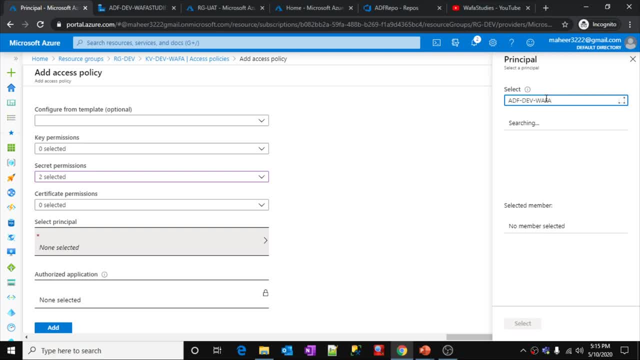 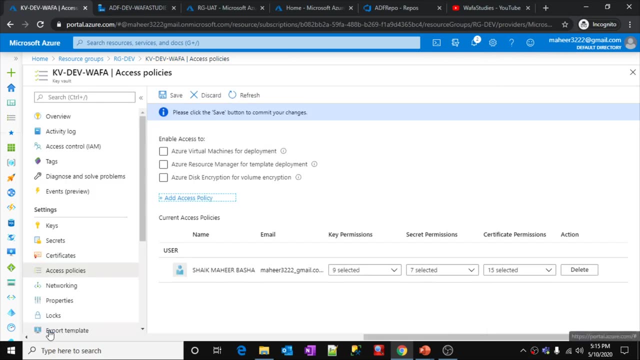 that, like this: adf, dev, wafaa, studies. right, so this is my msi. right, so this is my data factory name. right, so your msi is going to have the same name, see, so let me select that. let me click this select button here, and then let me click this add button. 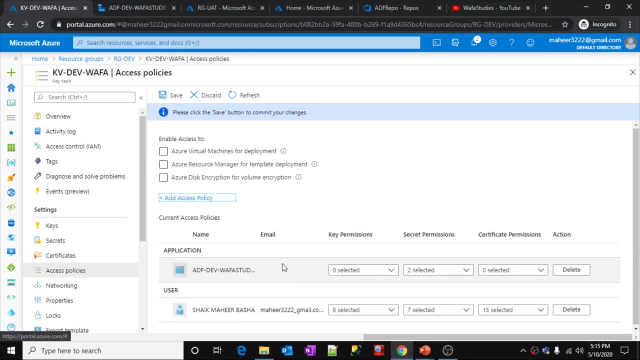 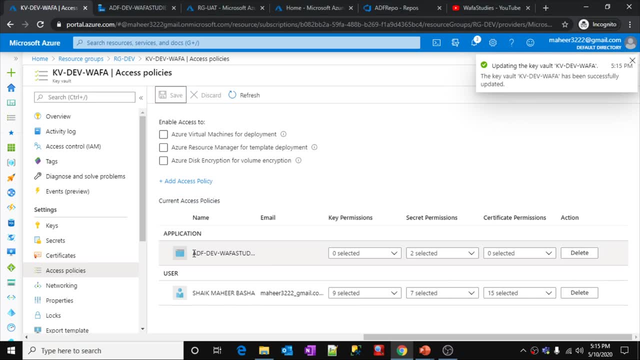 so this is going to add secret permissions on my data factory. let me click save button here. so that means for my dev key vault. I am adding permissions for my dev data factory so that my dev data factory, whenever it refers the dev key vault, it should be in a position. 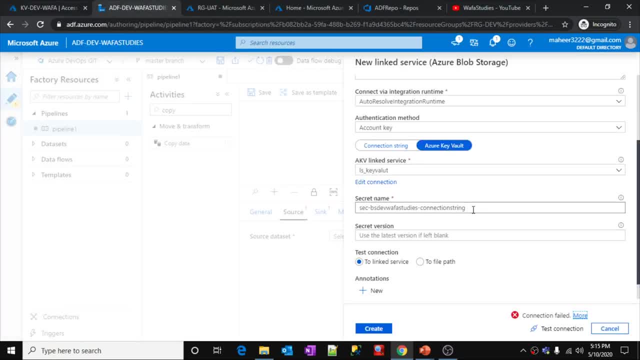 to access the secrets. why? because I am going to use the secret name for my azure blob storage right. so inside this secret I have the blob storage connection string. so let me click this text connection now. this time my azure key vault service is going to, that means my linked service actually. 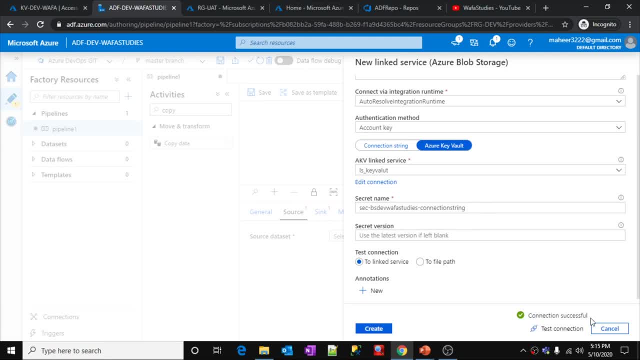 going to establish connection successfully with the blob storage. how it is happening? because inside this secret there is a connection string. since I have added the access policy just now, my data factory is able to access the value inside this secret and it is able to establish the connection with the blob storage. 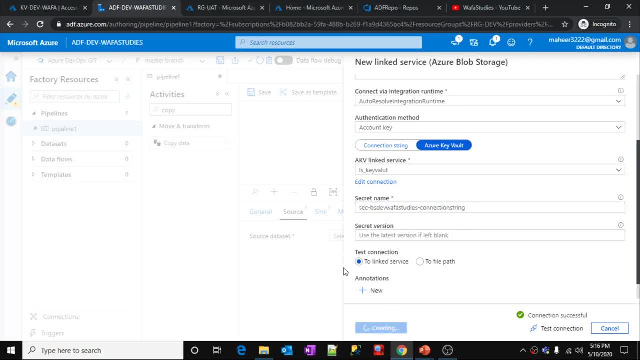 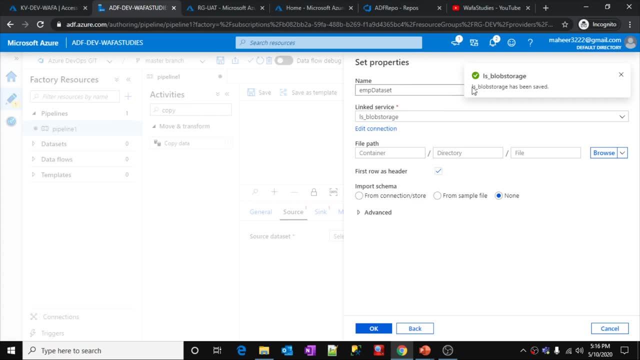 so now let's click this create button, which is going to create a linked service for my azure blob storage. ok, so it got created now. so all this we are doing because we are trying to create an employee data set, right, so let me browse the location now. 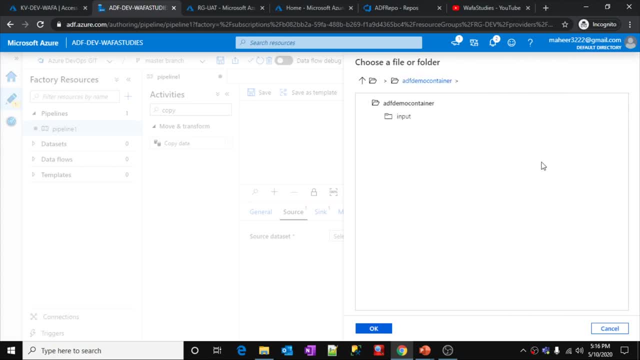 inside the adf demo container. see the same folder structure. everything from my dev blob storage. it is coming inside input folder. I have employeescsv file. let me select that and let me click ok. so let's click ok once again. so this is going to create a data set for my employeecsv. 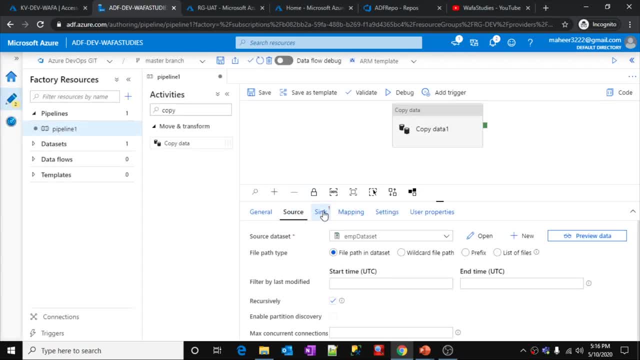 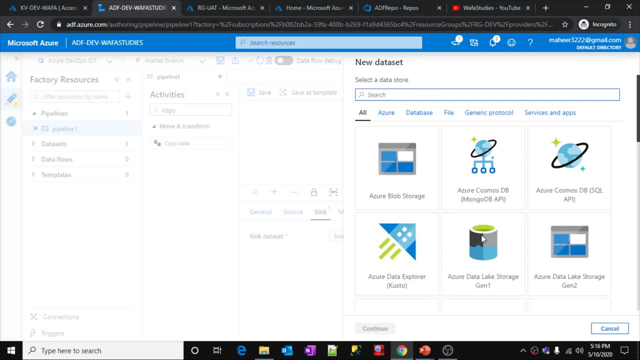 file. ok, that means that is going to act as a source. now let's go to sync. so here what I want to do. I want to create a new data set which should point to my output location. so again: blob storage, click on. continue same csv format, click on. 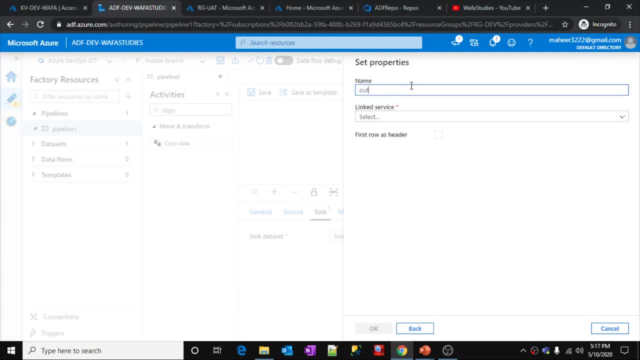 continue, so let me give a name for this data set. may be output data set. ok, so linked service. I just now created it for my blob storage. right, so the same storage. so let me select that then first row as header. fine, so let me browse the location. 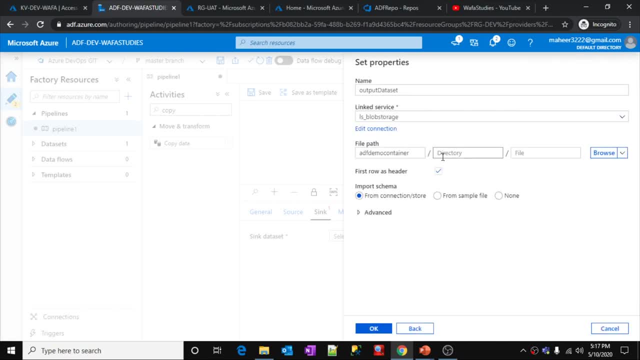 so adf demo container. ok, I don't have any output folder, so I am going to type it there. so even if you don't have that path, it is going to create a data set for you. don't worry. then select this none button and click ok. 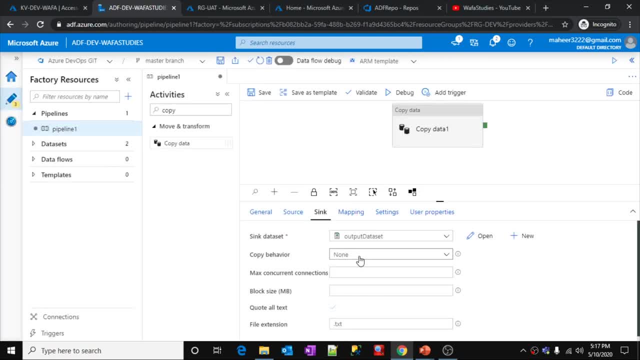 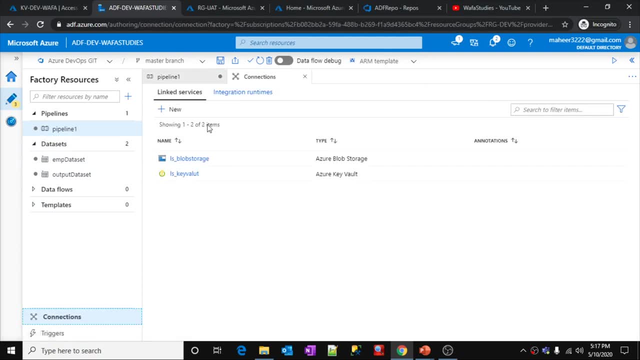 here, which is going to create a output data set. ok, so this is what. so, if you observe, I have created two data sets and also I have created two linked service: one is for Azure key vault, one is for my blob storage, and I have created a pipeline. 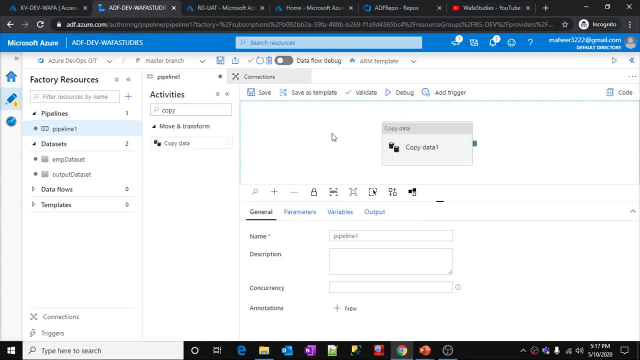 and where I have used a copy activity right. so this is what. so let me execute a debug execution to make sure my pipeline is working fine or not. ok, so if my debug execution is running successful, that means my pipeline is working fine, so immediately I will do the deployment. ok. 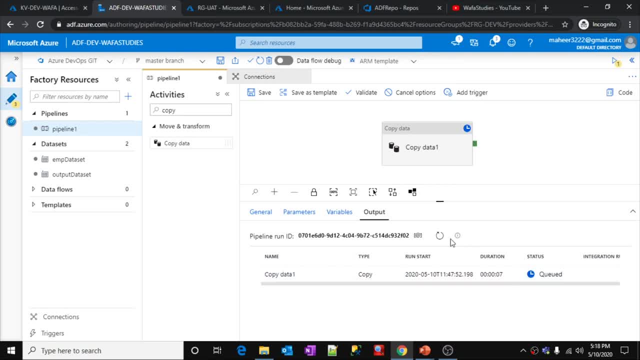 so let's wait for it. you can see copy. activity is in queue status. now let me click this refresh button here. ok, you can see status is successful now, so let's save this changes so that all the changes will get stored into the master branch inside my 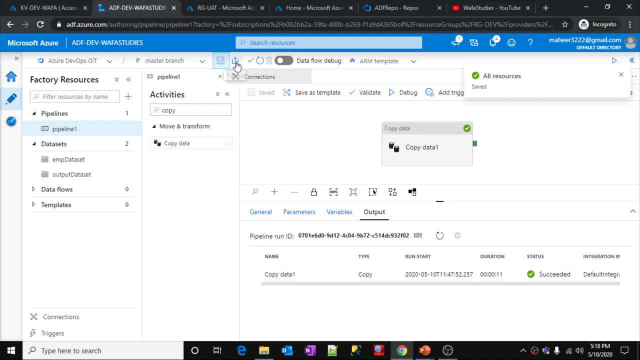 repository. ok, so changes are saved successfully. now let me publish all these changes. so I have clicked this publish button. so what it will do? it will publish all the changes to the Azure data factory and also it is going to create ADF underscore publish repository for us. 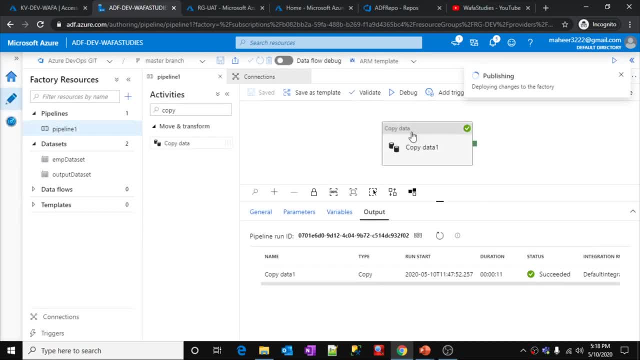 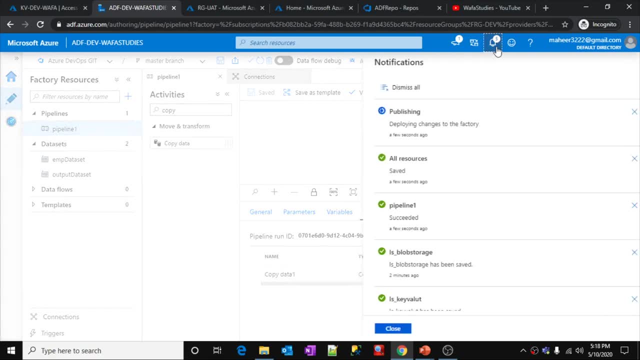 so I have. we have discussed that in our past videos also 73 and 74, right, so don't worry, we will look that practically now. right now the publish is running, so let's wait for the publish to complete. once the publish completed, we will go to Azure DevOps location. 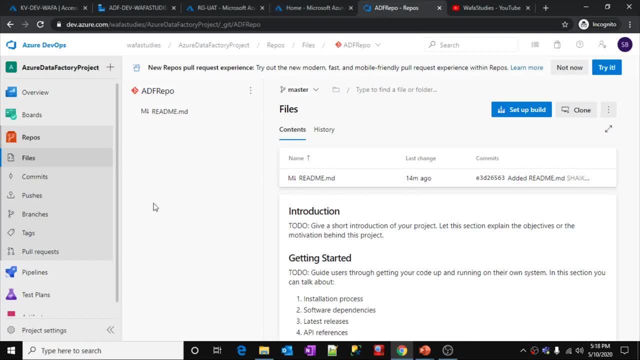 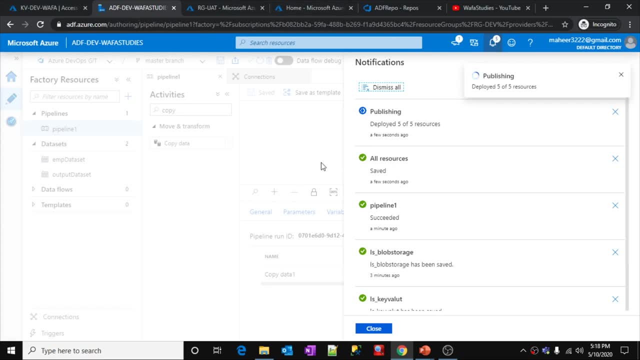 here. so where is there here? and we will try to see whether the new repository got created or not. ok, so let's go to our Azure dev. sorry, ADF dev environment related AIF. so deploying all 5 to 5 changes. yeah, you can see. publish is completed. 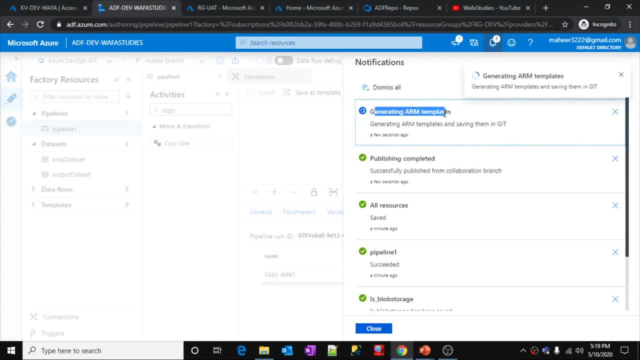 see it is generating ARM templates. as I said, right, whenever you publish the changes, it will generate the ARM templates inside the ADF underscore publish repository. ok, so why? because from from there, only ARM templates will move to the other environments to deploy your changes. right, so see everything. 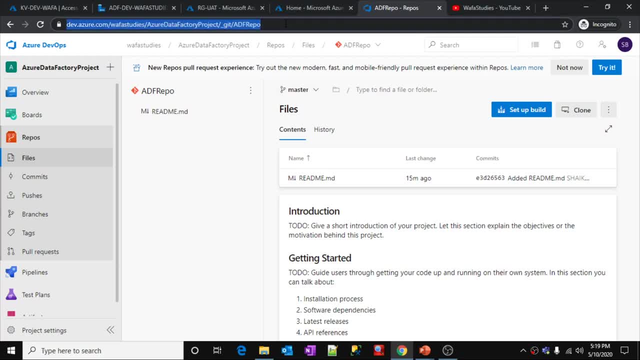 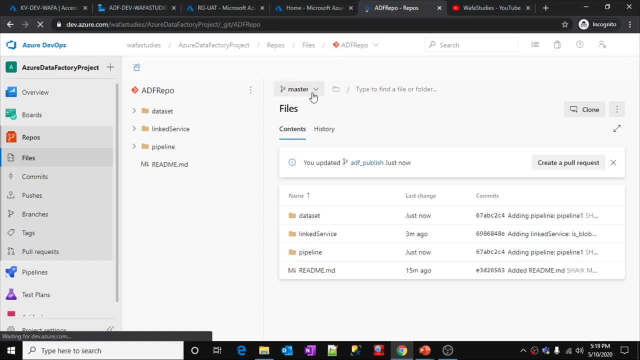 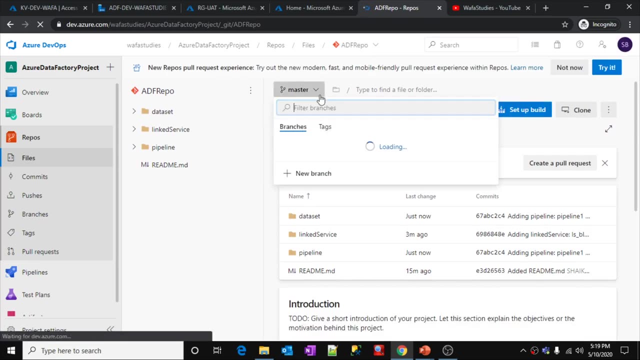 is successful. let's go to my devops. let me refresh this page here. so right now I am under ADF repo- ADF repo repository. this is the master branch. you can see there is a latest update ADF publish branch just now created so I can navigate to ADF publish branch also from here. 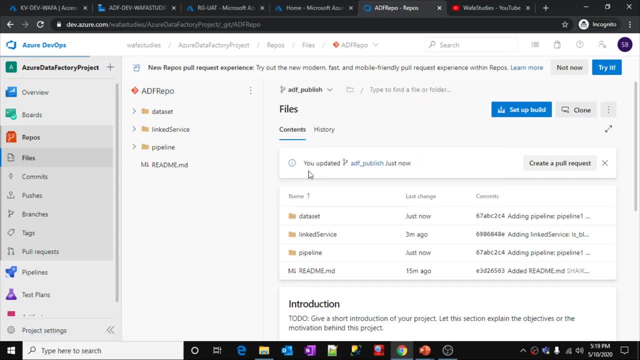 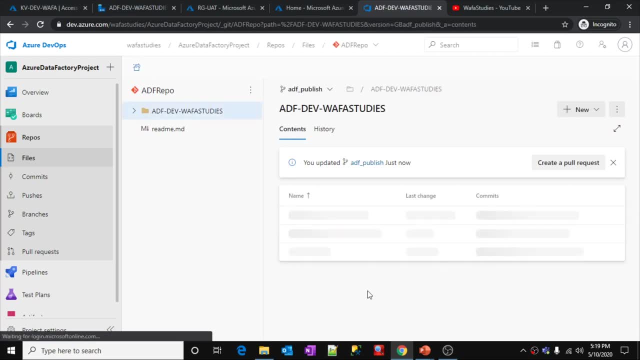 this drop down. also see there is ADF publish branch. let me select this ADF publish branch. see, you can see there is a folder with my data factory name and if you open inside that folder you will have the ARM templates for your. there will be 2 templates. 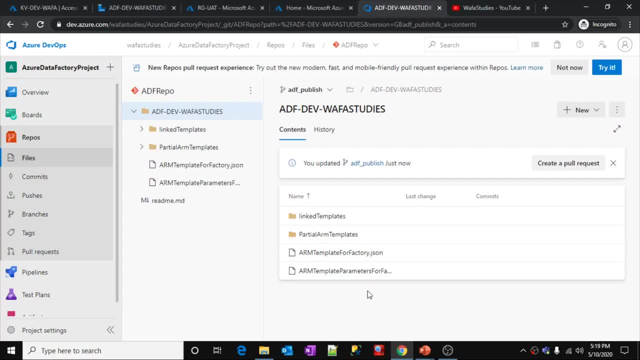 one will be data factory template itself and another will be parameters. ok, see, one is parameters template, one is data factory template. this parameters template we are going to use for different environments. that means, if I am going to deploy this data factory pipeline into UAT, then I am going to specify. 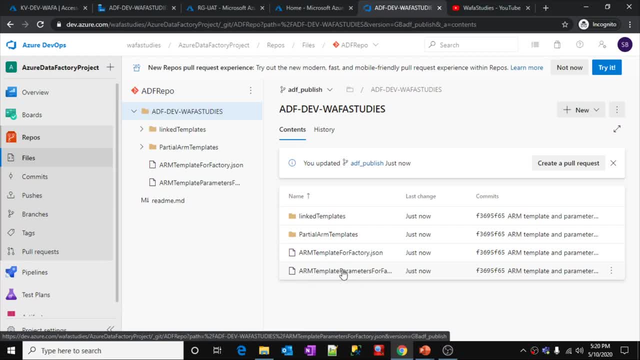 some UAT related parameters here, because I should make sure my UAT pipeline should work with the UAT resources right. so that is the reason. so there will be 2 json: one is for data factory, another one is for parameters. ok, so we no need to open this json. 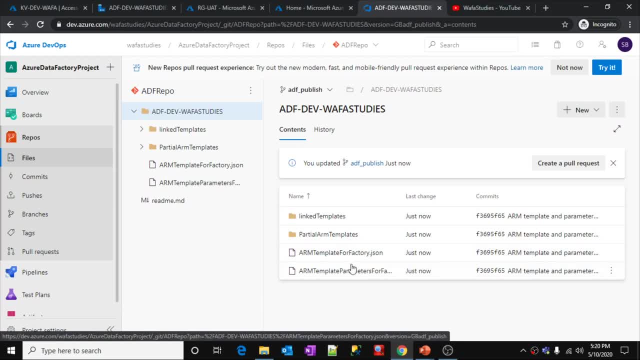 and examine the changes. if you want, you can do that. so for this video that is not, we are not concerned about it. so we are concerned about creating a release pipeline. now let me go to my UAT resource group. let me open this ADF, UAT, wafa studies. 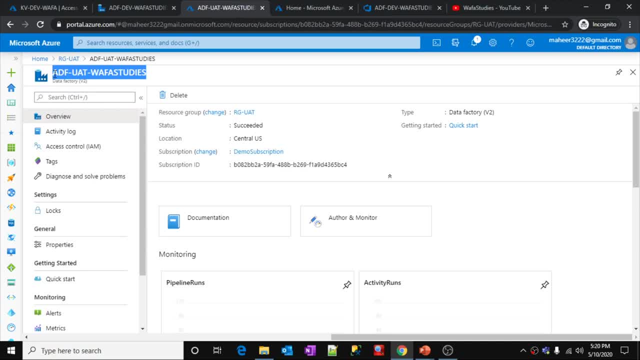 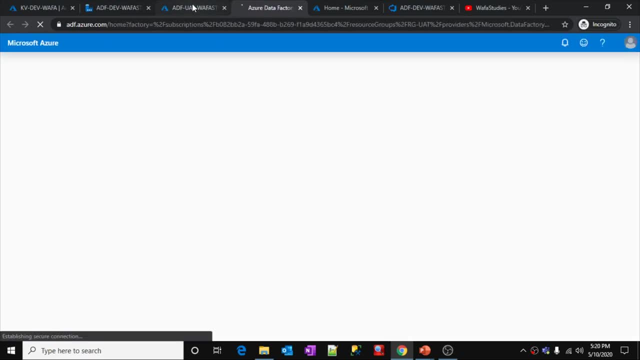 this is the data factory name, right? ok, so let me copy this, let me click this author and monitor tile here. let's see if there are any changes already there. so this data factory we just now created, if you remember, I think, from 10 to 15. 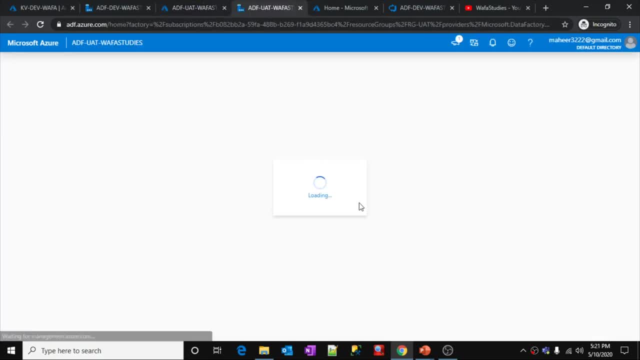 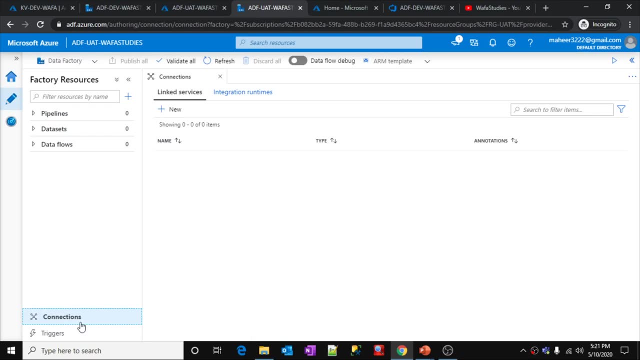 minutes before we have created right. so right now, this data factory is going to contain nothing. that means zero pipelines, zero data sets, nothing. see: zero pipelines, zero data sets. if I go to connections, zero linked services. so this is good. now, once I deploy it from my release pipeline, everything will come here. 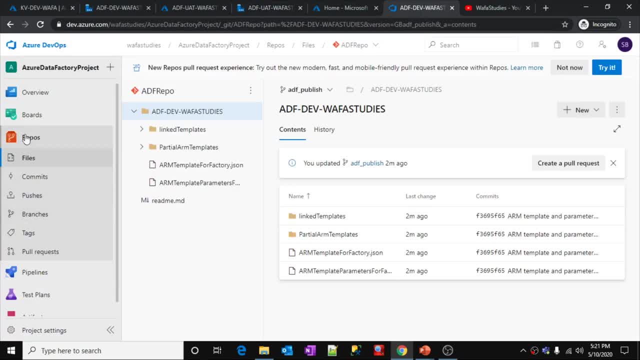 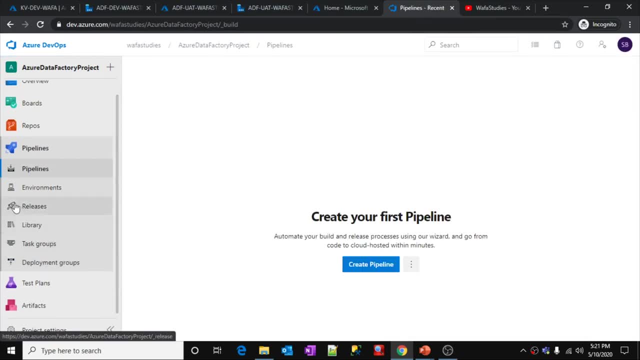 I will show you that now. let's go to my devops account. so here you need to navigate to these pipelines, azure pipelines. so these are release pipelines, ok, so if you go there, there is something called releases, so click on that- releases. so that is where you will actually create. 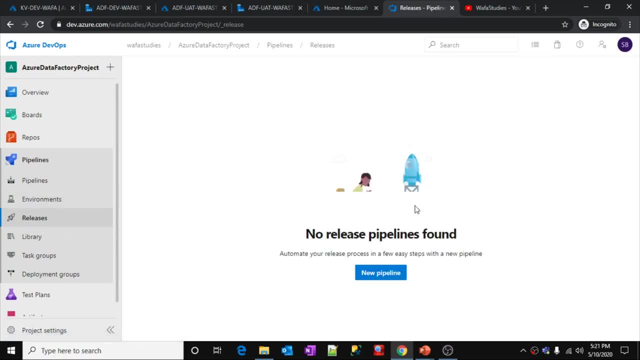 your release pipelines. ok, so once you click that, you can see there is no release pipelines. if you want to create, click this new pipeline. so let me click this new release pipeline, because I want to create a new release pipeline, right, and I want to move the changes from. 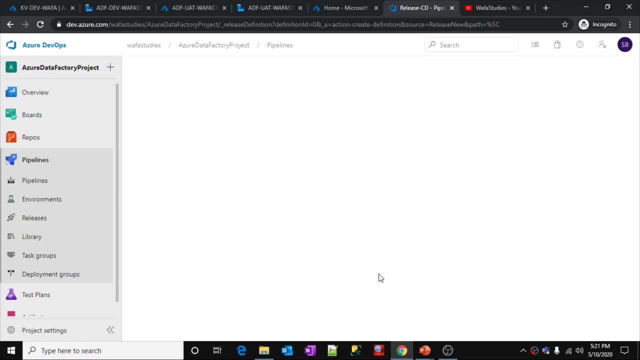 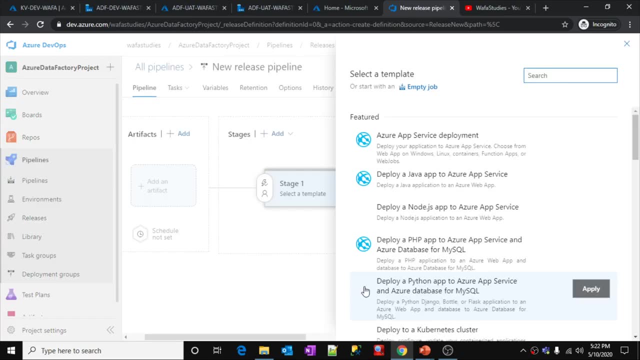 dev data factory to UAT data factory- right, that is what my requirement. so let's wait for the screen to load. ok, screen got loaded. you can see here. screen got loaded right, so you can see. there is something called artifacts, there is something called stages and everything. don't worry, I am going to explain all of 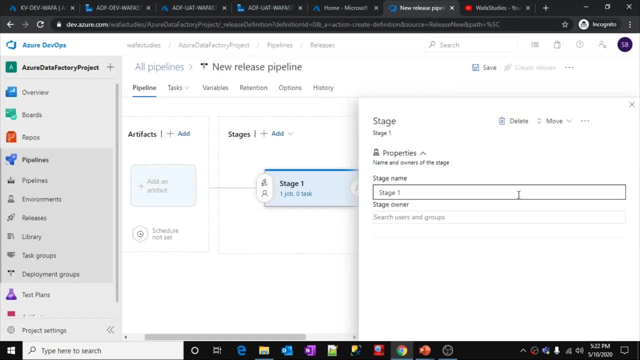 that now. for now, click this empty job because I am going to create empty job. so here there is stages. right, you need to provide a stage name. so right now my pipeline has to. this is not azure pipeline. remember, this is the release pipeline. you can see new release. 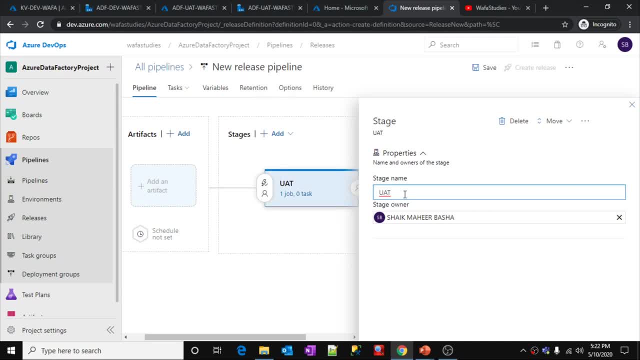 pipeline. so this release pipeline has to deploy the artifacts. that means deploy the pipelines or deploy the data factory related changes to the UAT environment. so that is the reason for this stage. I am naming it like UAT. ok, so let's close that. so in the UAT. 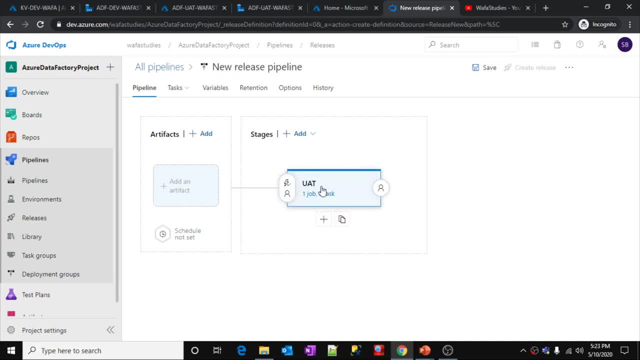 stage it is going to deploy the changes to the UAT environment. that's what it is. so let's let me give a name properly here. first, for this release pipeline, maybe adf release- this is what the adf release pipeline, ok. or else adf wapaa. 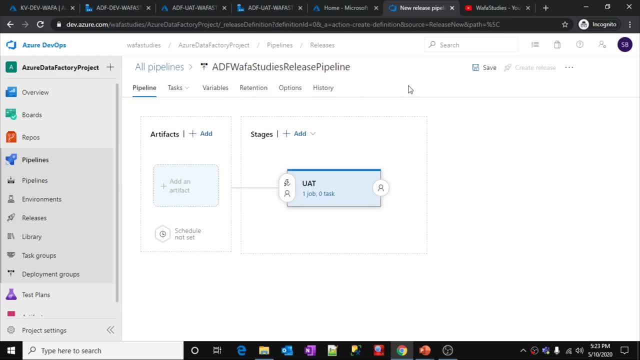 studies release pipeline. this is what my release pipeline name I want to keep. ok, so that is fine. or let's keep simply adf release pipeline. that is fine. why to use lengthy name? so let's keep only adf release pipeline, one second adf right. ok, so this is fine. 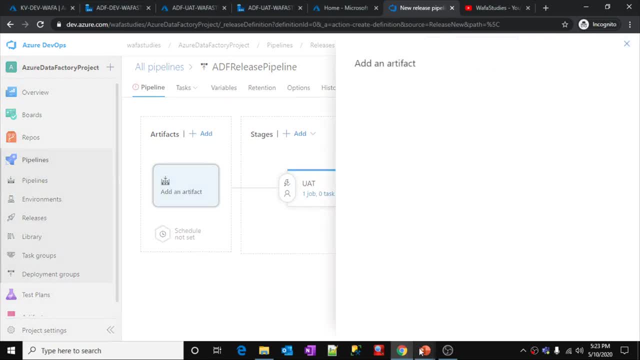 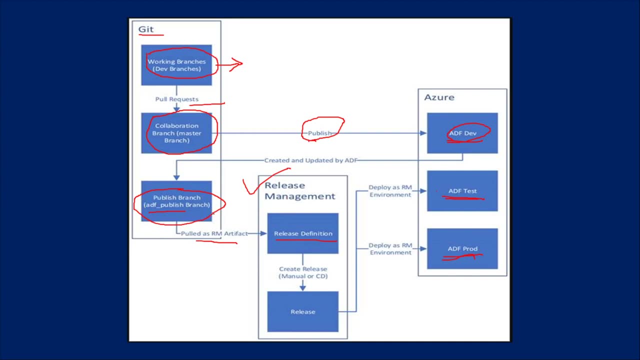 now I need to add artifacts first. so if you remember, let me go to presentation. what I said is: your release pipeline has to take the files from the adf publish folder, that means from the adf publish branch, and it has to deploy the changes into the respective environments. 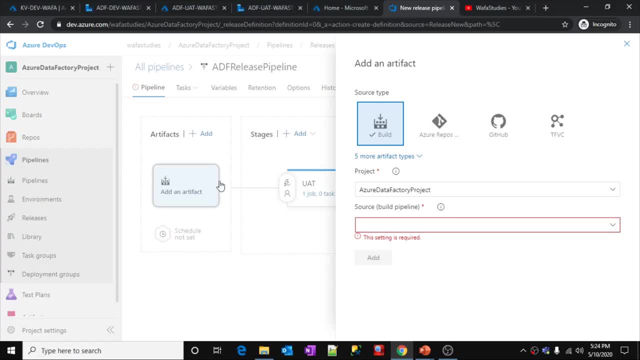 so that is the reason in the artifacts section I should select that adf publish branch. so let's select this. for example, if your code repository is github, you need to select this. so in my case, my code repository is azure repository- right azure devops rip, so I selected that. 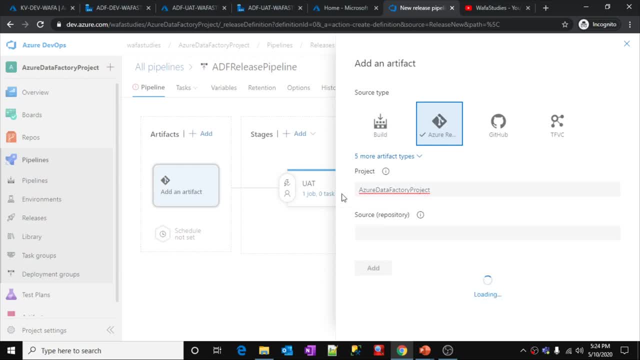 so let me select my project. so, azure data factory project. that is my project name, right? yes, so what is the repository name? so my repository name is adf, repo. right, so let me scroll down. so now you need to select the branch, from which branch you need to take that. 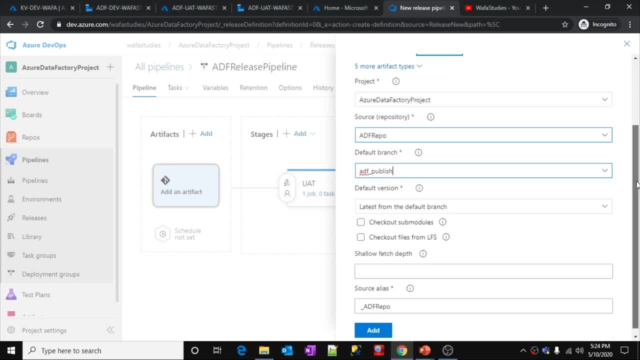 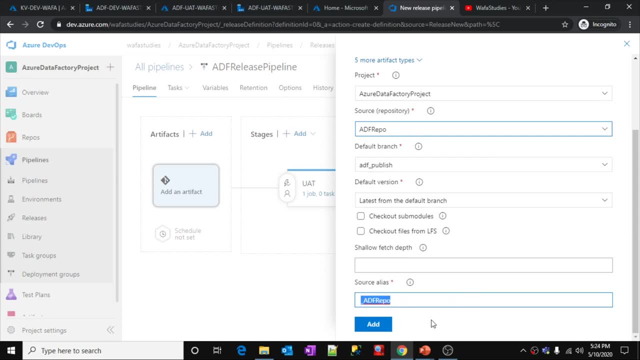 artifacts. so from adf publish. you should take that, ok. so then you can see there is alias name for your artifacts right underscore adf demo. so that is fine. I don't want to change them, so that is fine. let's click this add button. so that means we have configured the artifacts. 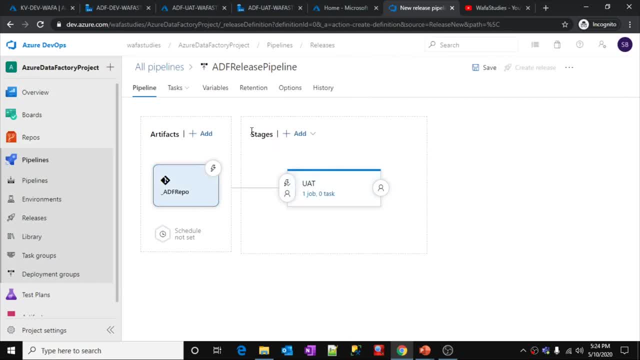 which has to be deployed into the different stages. in my case, I am creating only one stage. if you want to add new stage also, you can add. maybe this stage name is uat, right, you can add another stage like prod, so that means when you trigger once, you trigger this. 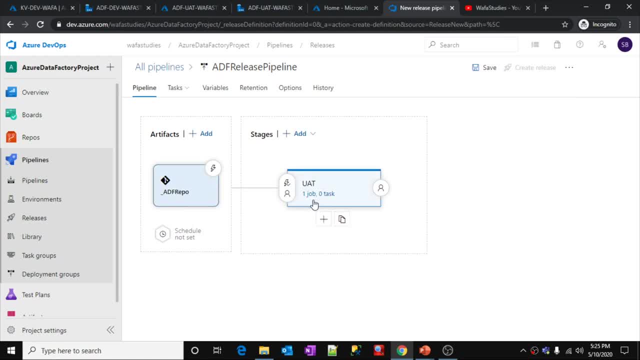 release pipeline. it will take the artifacts to the uat stage and it will deploy here. and then it will take once again the artifacts to the production stage and it will deploy there also, so like that you can add any number of stages here, ok, so right now I am concerned about only one stage. 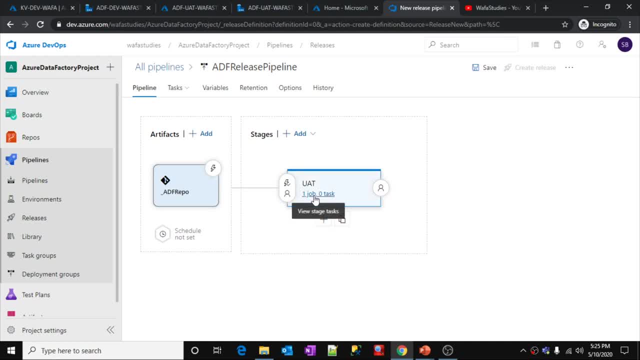 that is enough. this is for a demo purpose, right? so now let's click this job and task. we need to create a task job here, so you can see, here there is already one job, right? what you need to do. you need to add a new job here. 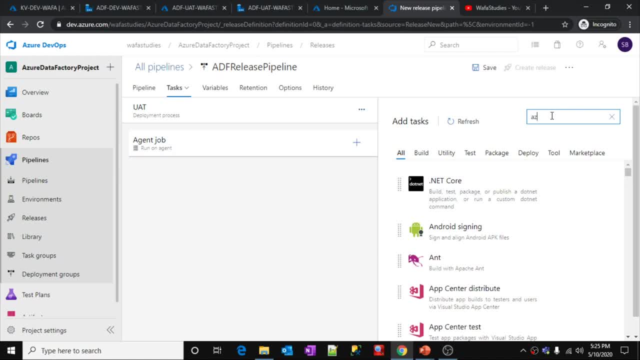 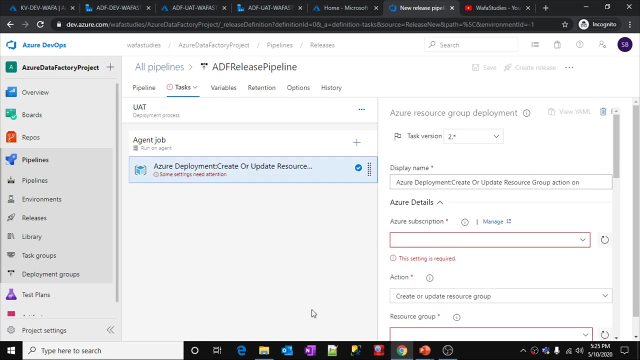 new task actually basically so: select like azure resource, group deployment. you need to use this task, click this add button. ok, so I have selected that particular task. let me click this task now. so here I need to fill few configurations. so the first thing is you need to select your azure. 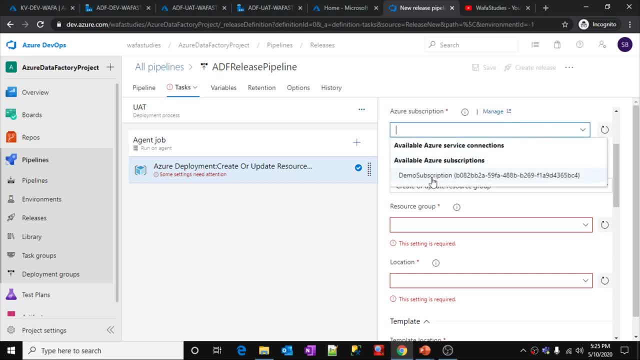 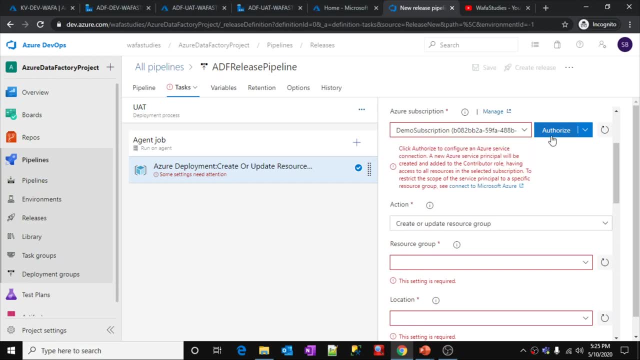 subscription. ok, so let me select mine. so this is my azure subscription. so once you see what it is saying, once you select the subscription, it is asking you to authorize. once you authorize, what will happen is behind the scenes. it is going to create a service principle automatically using 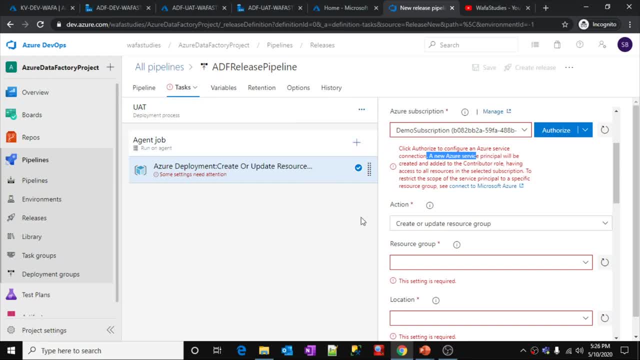 that service principle. this release pipeline is going to interact with azure subscription and then thereby it is going to perform all the activities. so you are, it is making sense right why this service principle is required. so if you guys don't know about what is service principle, let me explain you in. 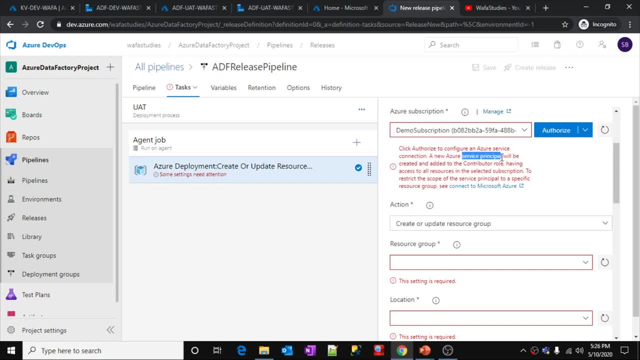 one line service principle is nothing but the identity. using that identity you can access your azure subscription and also you can access your azure resources, depending upon the permissions that particular identity has. that means that particular service principle has you can perform all the activities on the azure resources. 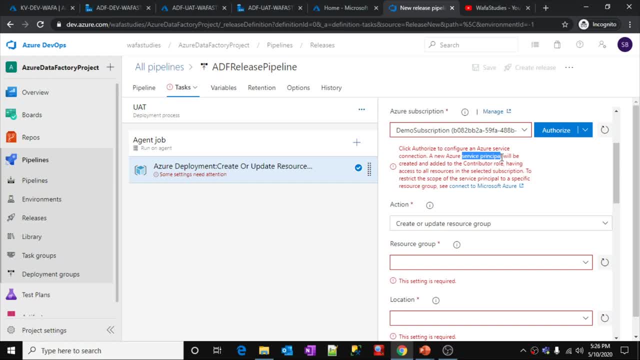 your resource may be blob storage, your resource may be data factory, your resource may be azure sql, whatever may be, it is so all those resources you can access using identities. so if you want to generate a identity for any type of application, in that case you will go with the. 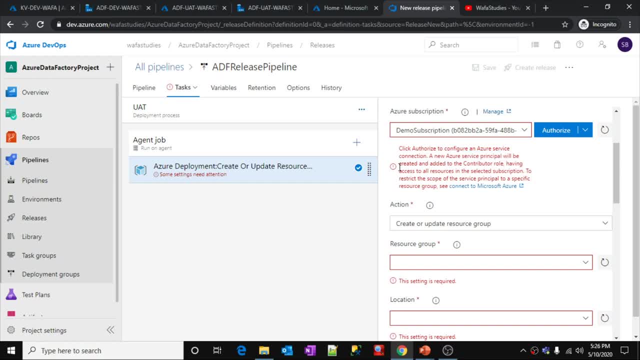 service principles. so in this case, my devops release pipeline has to interact with my azure subscription and also it has to interact with with uat resource group, and it has. it also has to interact with data factory in the uat and it has to deploy the changes. so to do all these, 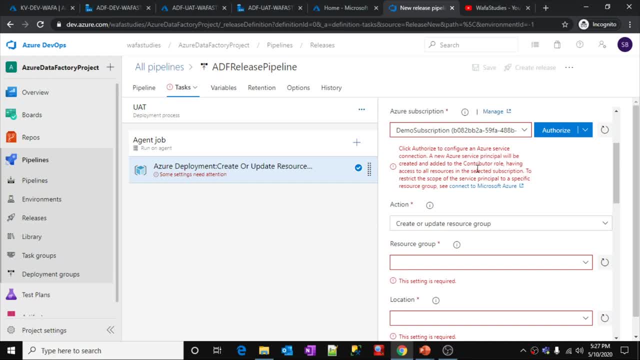 activities. it should have the access first right. so you should have one identity first. for that identity you should have some access on your subscription so that that identity can do all these activities. so that is the reason it will ask you to authorize, so that behind the scenes, 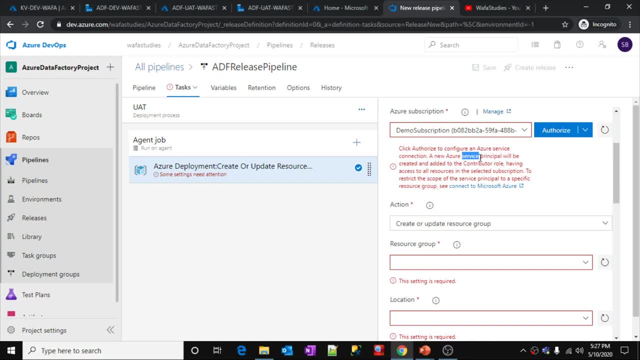 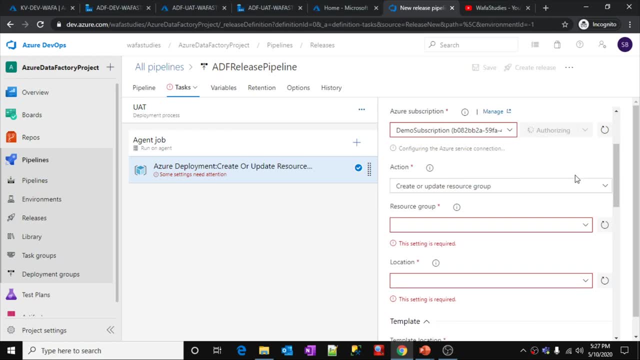 azure devops will create a service principle for you automatically inside your subscription. using that service principle, it will do all the deployments. so let's click this authorize button. so this is going to create a service principle for you inside your subscription automatically, okay, so remember that point. 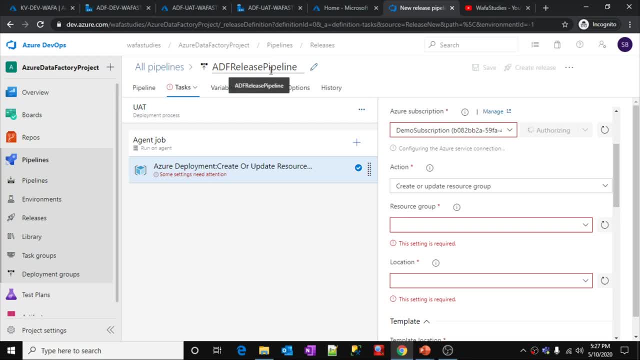 so because you might be wondering how your devops release pipeline is going to interact with your azure subscription and how it is going to change the resources there, right. so behind the scenes, the logic is because of the service principle. when you authorize, the service principle will get create, right. 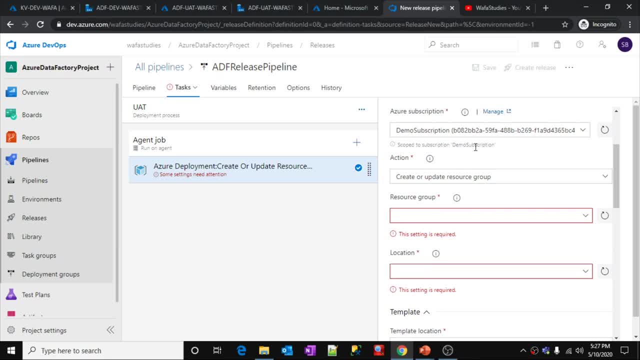 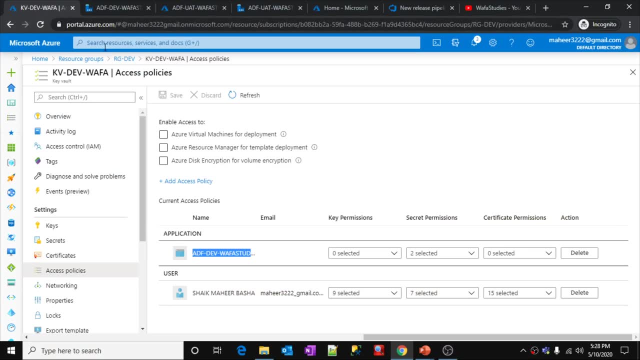 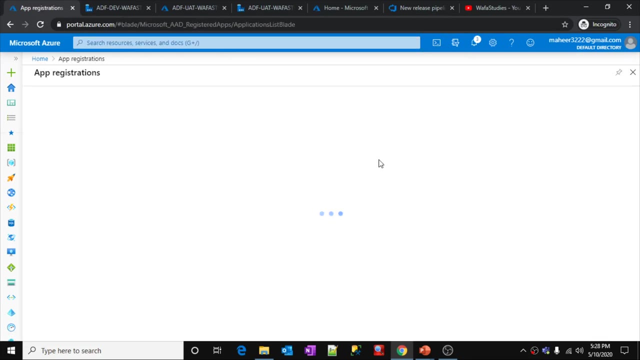 okay, so your service principle, my service principle, already get created, okay, so i will show you that also. okay, let me show you now itself. so let, if i go now here, let me search like i go under app registrations, so service principles will be available under app registrations, okay, 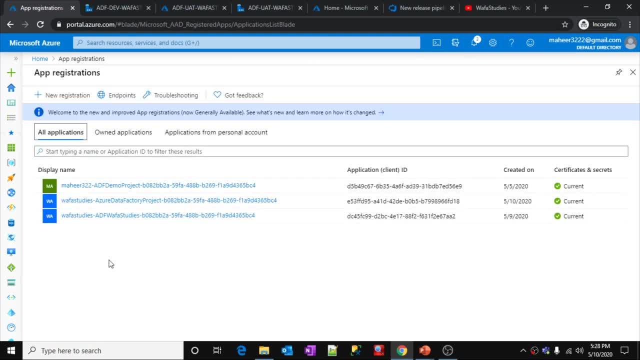 so let me search it from here. see, you can see here wafaa studies- sorry, this one. wafaa studies, azure data factory project- this is my project name, if you remember. see, this is my service principle. just now got created. you can see the data also. so, similarly, i have already. 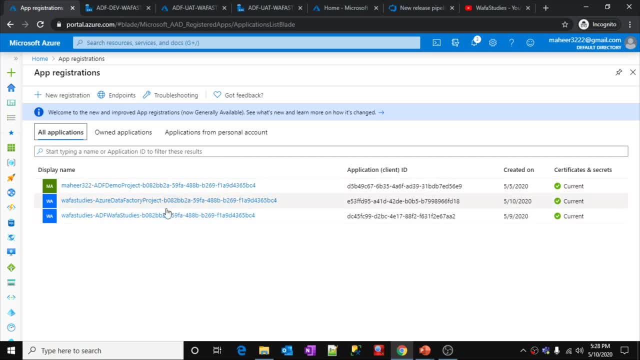 tried, actually from devops, so these two are coming from there. i am no longer need of these service principles. i can delete them, so, but they are there right now. that's fine. so this is our service principle, which got created just now. okay, and by seeing the name itself, 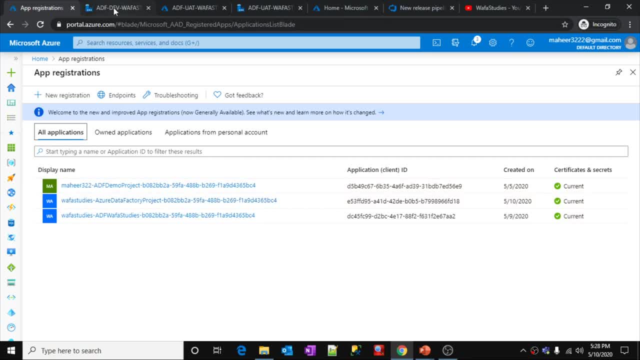 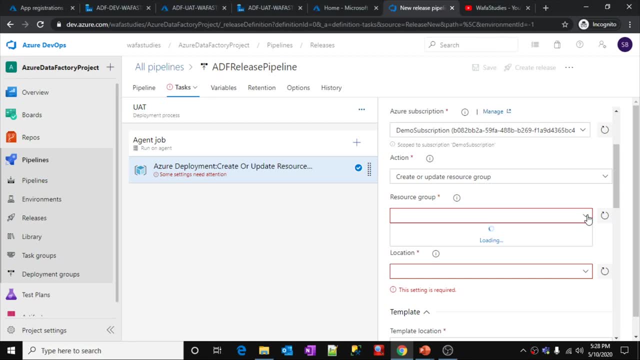 this is my devops account name. this is my devops project name. okay, so that is fine. let's go to our release pipeline here once again. so here we need to select the resource group on which you want to deploy changes. right, so i want this deploy. 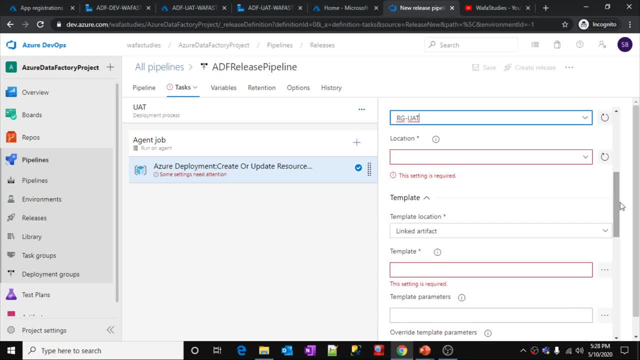 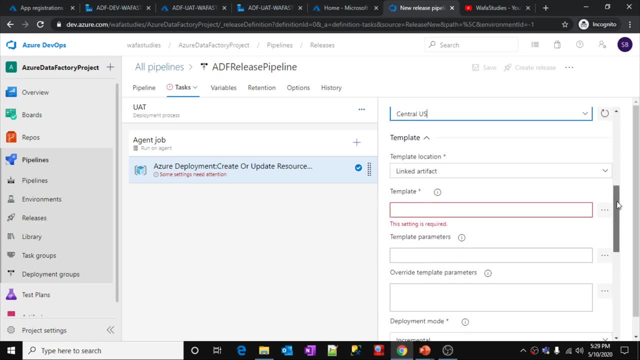 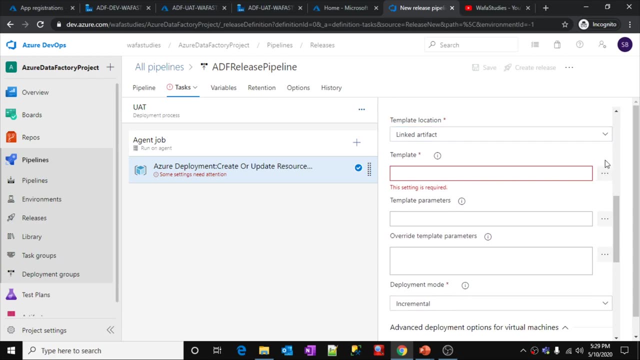 changes into my uat resource group. okay, then you need to select a location. okay, so i am going to select the central us. okay then here. this is where you need to select the template. what you need to do is actually here. you need to browse. this browse option is going to open. 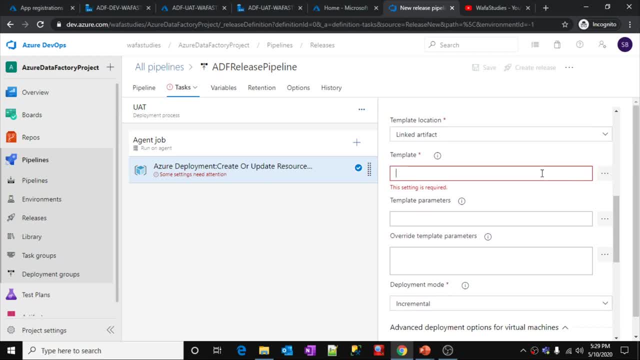 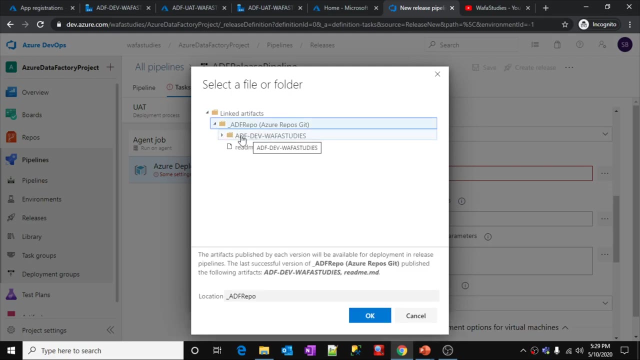 your adf underscore, publish branch and all the templates from there. okay, so let me click this browse button here once again. yeah, it is opening it here inside the linked artifacts. let me open this. see. let me open this data factory folder. see, there is a json right template arm. 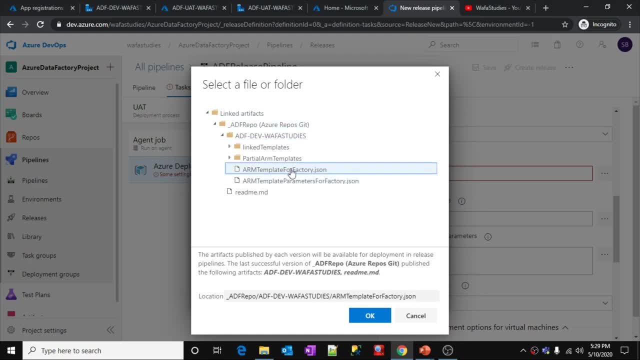 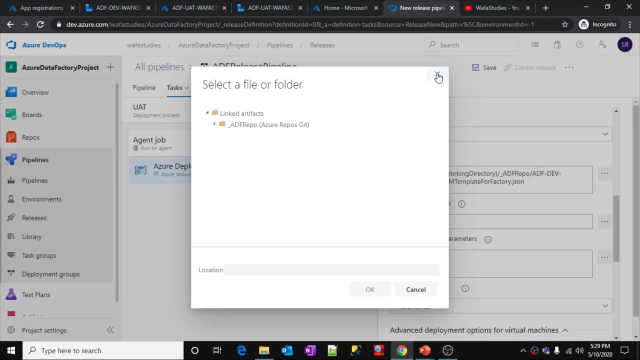 tablet. i have shown this previously. right. so that template, the data factory template, you have to select and click ok, so that is going to be added there. okay, so let me close that. let me close it. see, it got added here automatically. now you need to select the parameters. 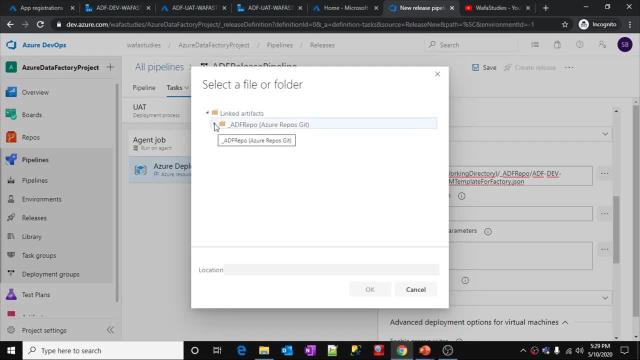 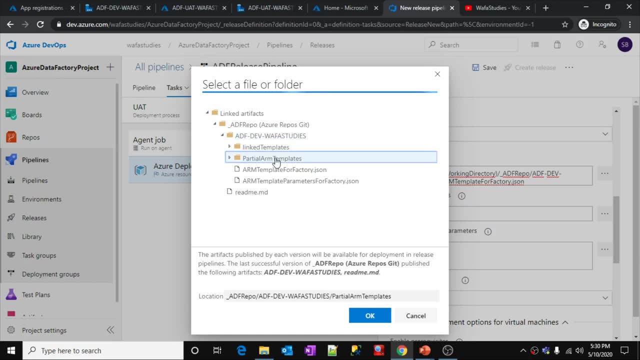 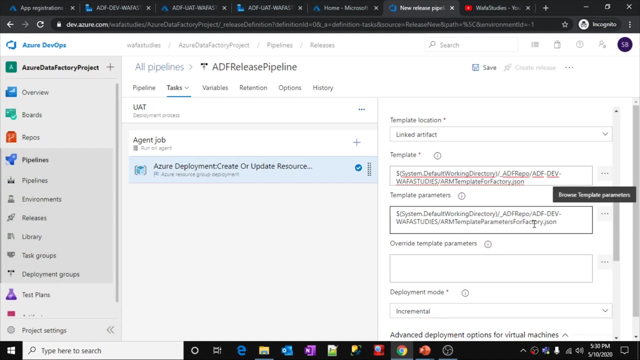 template. let me click this browse icon once again. now let me open your. let me open this. and then let me open this. let me select this. sorry, let me select where is this? this is the one parameters template, right, so let me click this. okay, see, i have added my parameters also now. 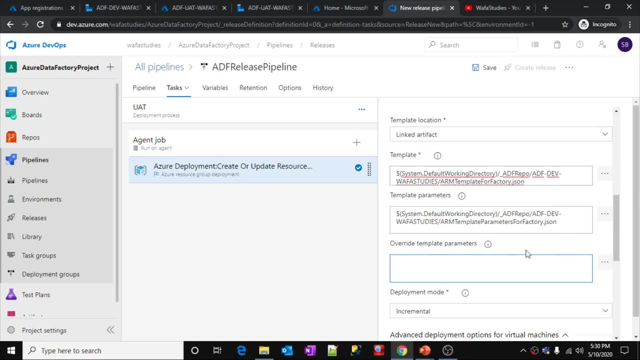 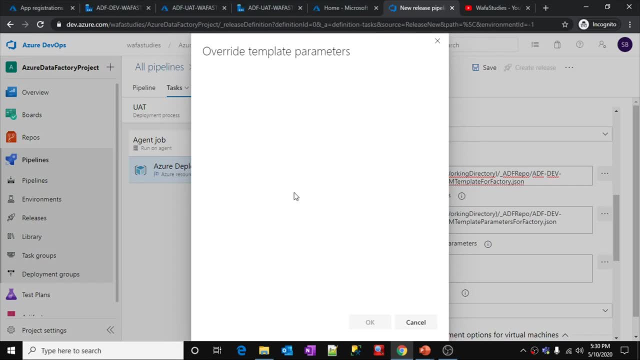 let me click this parameter: override parameters, template parameters. right, so what you need to do? you need to override the parameter values according to your environment. so if you do that, only your uat data factory will properly work with the uat resources. so in my case, my uat data factory name is going to be: 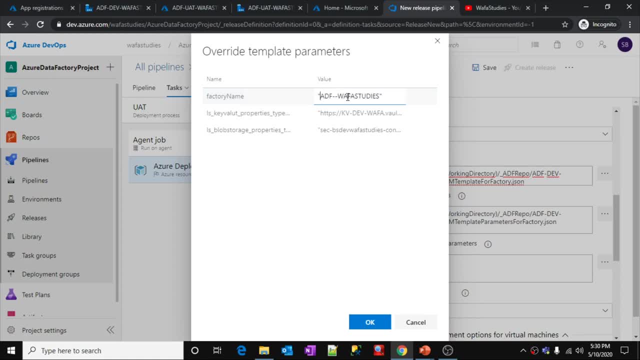 adf, uat, i think one second. let me remove this entire name, so i should give the uat data factory name. this is my uat data factory now. second thing: you should use the key vault for your linked service in for dev environment. it is using dev. 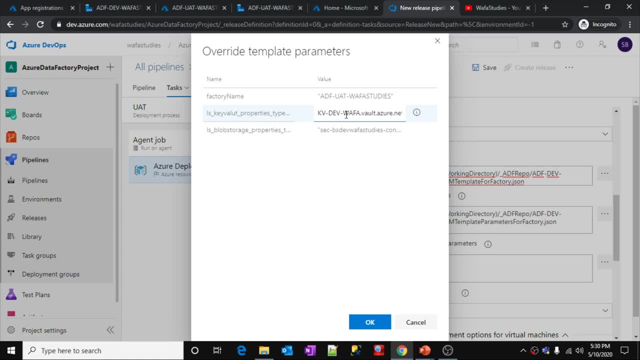 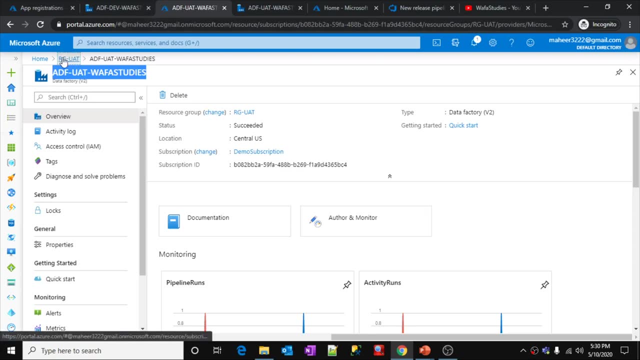 key vault. if you see here kb, hyphen, dev, hyphen, wafa, but for uat it should use the uat key vault, right. so let's go to. let's do that. let's go here, let's go to uat resource group. let me open uat. 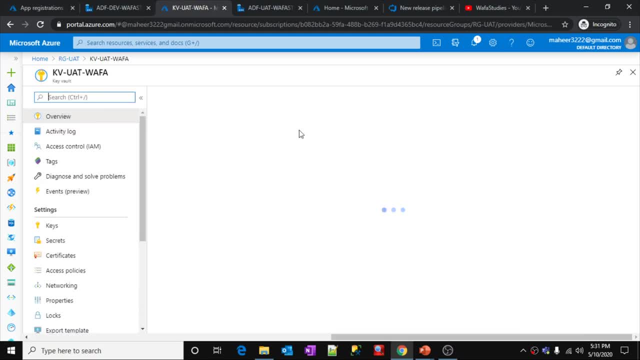 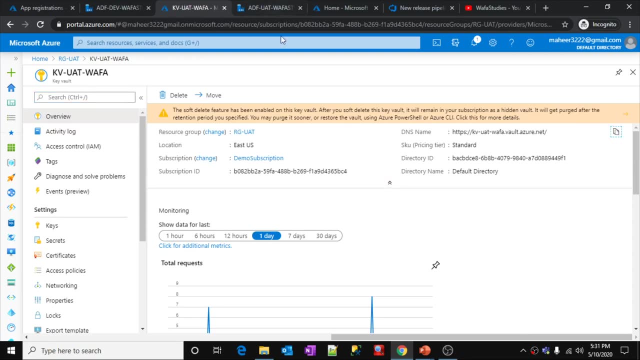 kb. wafa. uat key vault. okay, so let me take the url from here. i should override with the uat key vault id- here i mean uat key vault url, because i am going to deploy the changes to the uat environment, right. so for that is the reason. 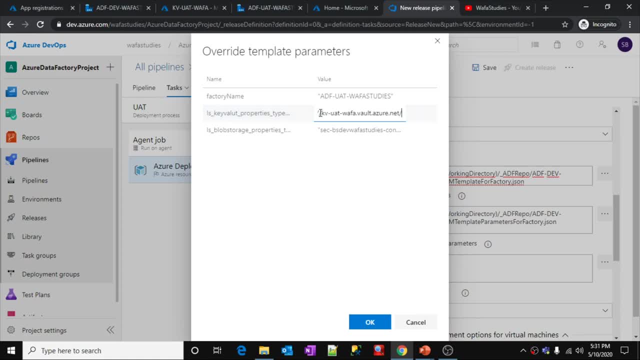 okay, so let me delete everything here and then provide the uat key vault name. then i need to provide the secret name from the uat, right, because this secret name should be coming from the uat key vault, right? so let me delete this secret name here. 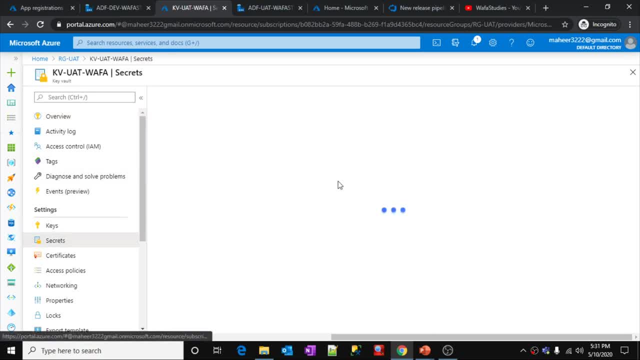 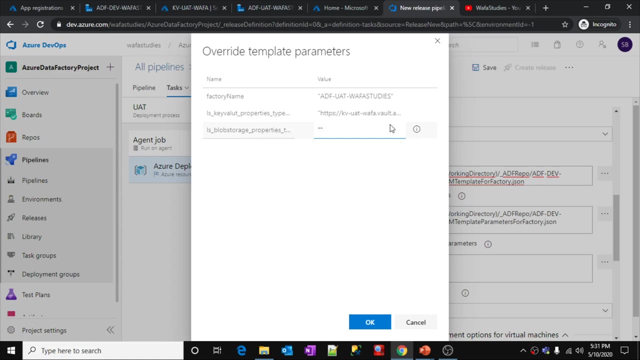 let me go to keyword once again. let me go to secrets. so here i should have a secret. i have already created that with the. this secret is going to hold uat related blob storage connection string. okay, so let me copy this. let me go to release pipeline. let me paste that. 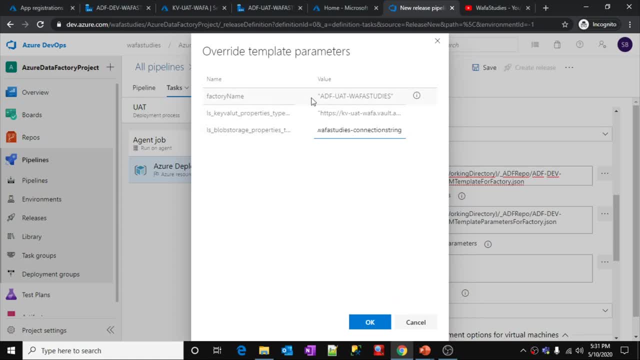 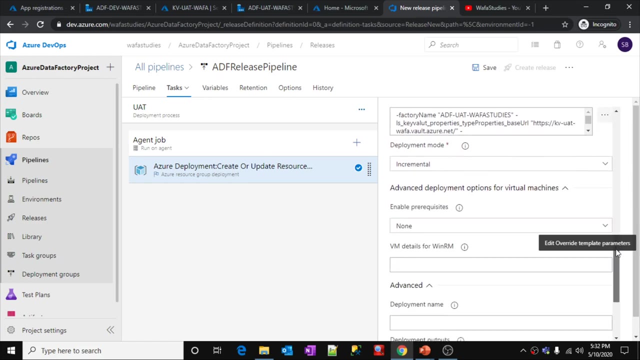 so i have configured everything with the uat values now, because i am going to deploy this to the uat stage. right, okay, one second did i, did everything properly. yeah, i think i am good. so data factory name: also uat. right, okay. so click. okay. okay, that is fine. so deployment mode is in. 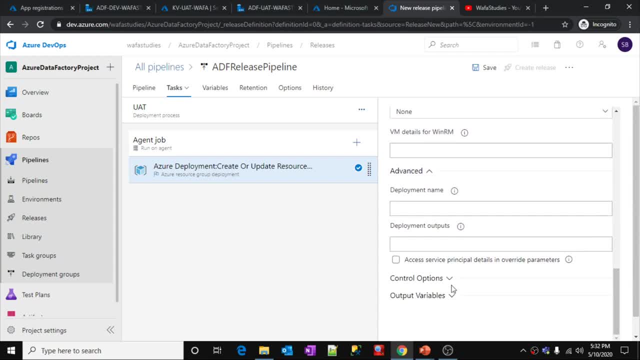 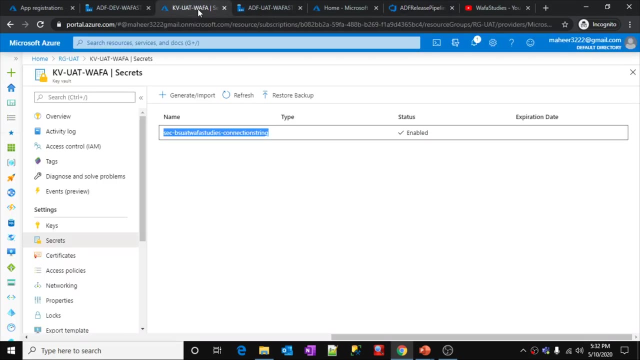 that is fine. okay, so these are all values, is fine, so just click this save button and click this ok button. this is going to save this ADF release pipeline. okay, so your release pipeline is successfully created. now, before executing this release pipeline, let me go here inside the UAT key wall. let me 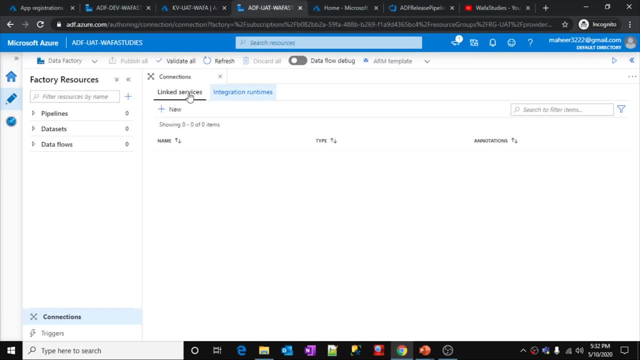 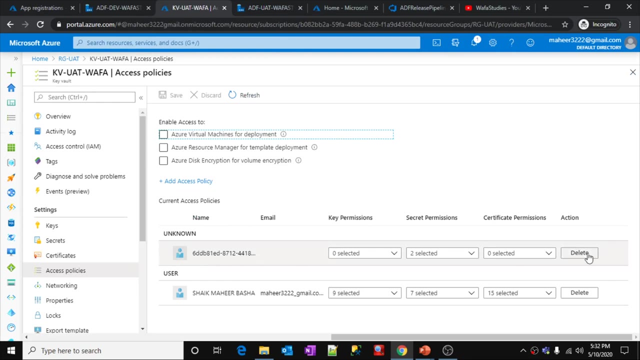 go to access policies. I think this UAT data factory just now I created, right, so when the new pipeline and new data sets come here after deployment, my data factory should be able to access UAT key vault secrets. right, for that I should have the permission for my data factory, right, let me create that. let me delete. 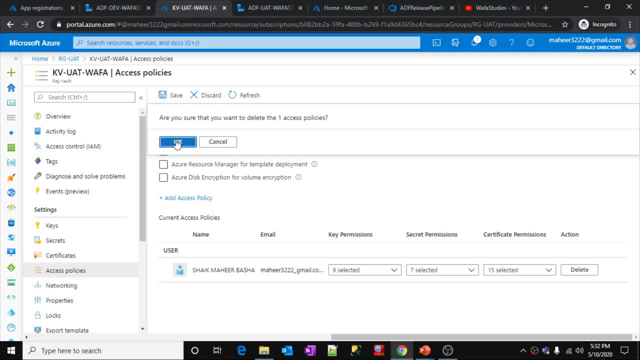 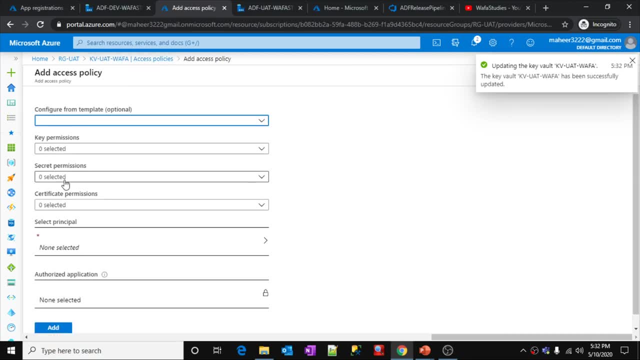 this. this is the old setting. let me save it first. then let me add the access policy. just now I did the same for the UAT key vault, also for the UAT data factory right. the same thing I am doing under secret permissions. I am going to. 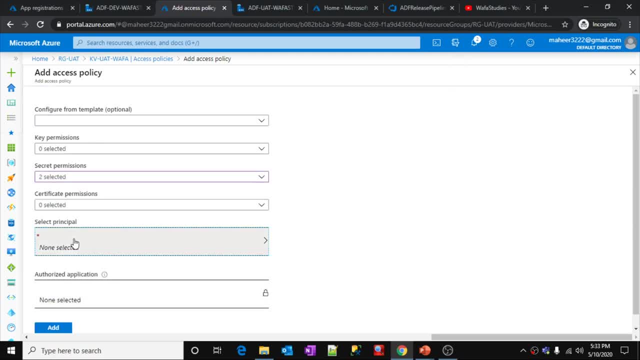 select, get unleashed, then click this select principle. so here I need to select the UAT data factory. MSI, the means managed service identity, so the easiest way is provide the same name as far as, whatever the data factory name you have your MSI name also going to be. 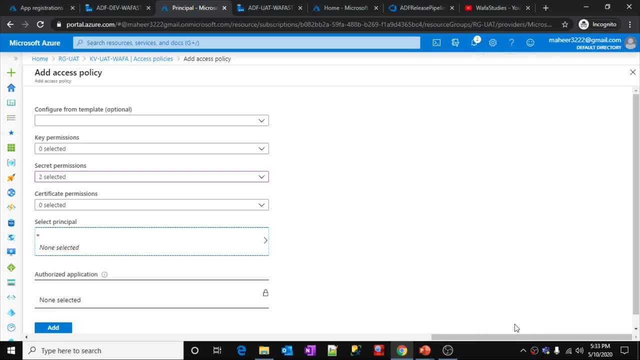 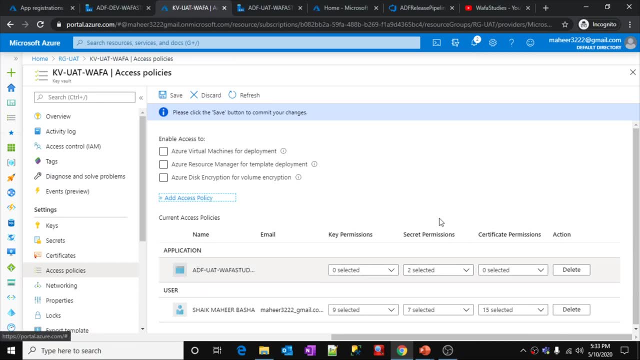 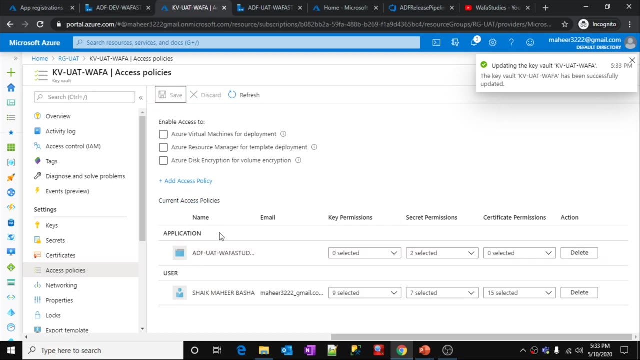 same you can see here: ADF, UAT, office studies. click this select button here and then click the add button here. okay, so this: this added my UAT data factory MSI here with the secret permissions. so now let me save this. so that means my data factory is now able to access my UAT key vault right. this setting should be. 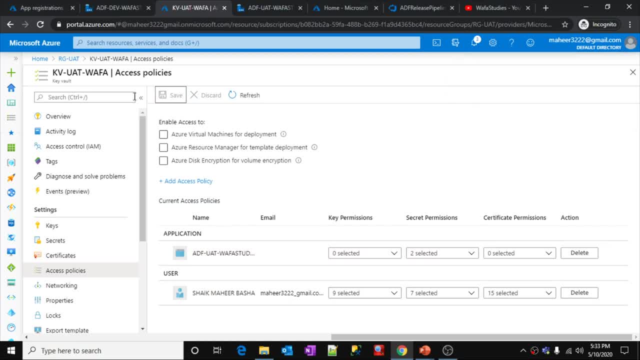 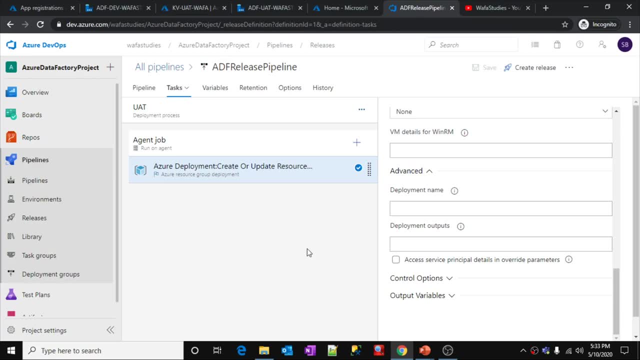 there, right? or else it, when it try to access the secret from this key vault, it will throw error. you don't have access, that is there. it will throw. let's go to release pipeline. so we have completed this release pipeline. now you can trigger your release from here directly, or let me go to these releases freshly. 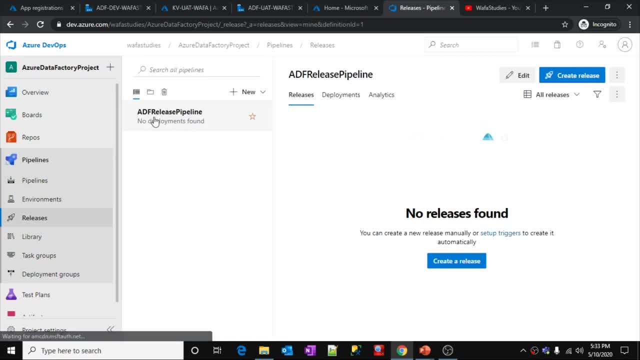 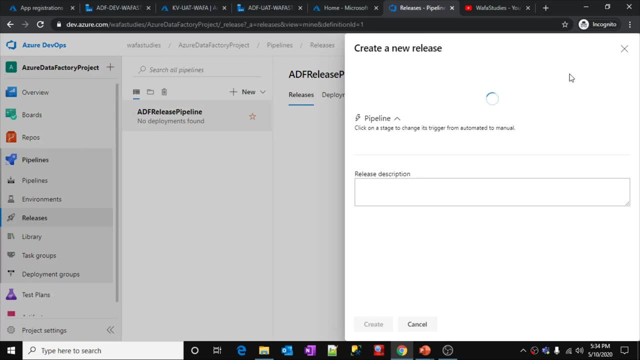 so that I you can see properly. you see, this is my release pipeline: ADF release pipeline. right and right now, there is no release created. okay, no releases found. so click this create release for this release pipeline. so click this, create release. so what it will do? it will ask you to create a release. that means once. 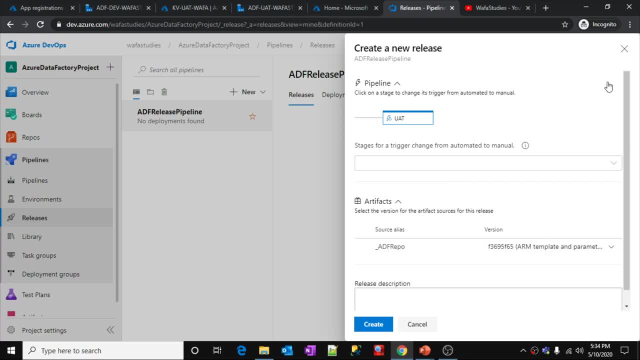 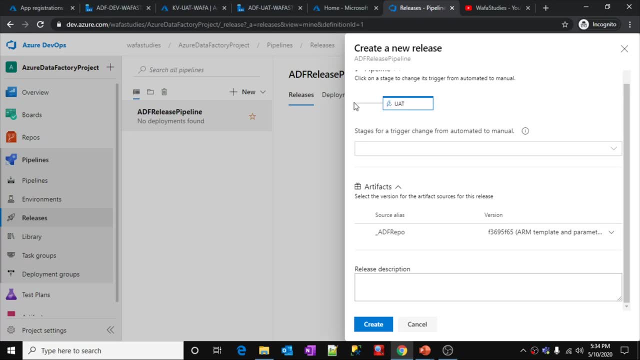 you click, you create the release. your deployment will start. okay, so let me scroll down. I am NOT going to change anything here. see, it will show you in which stages it is going to deploy. right now it is going to deploy into UAT stage. so click create button here. so this is going to create a release. you can see. 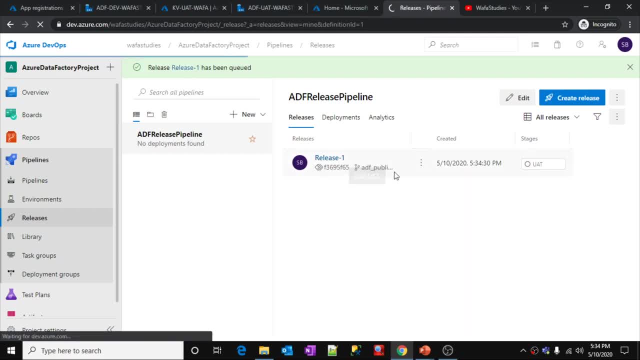 release one has created- right, you can see the status also here. release one UAT. right, it is running. so let me click this release one. it will show you the progress also. let's wait for few seconds. it is loading right, let's wait for two. no, it will take from five to three. I think the network is slow. my side guys. 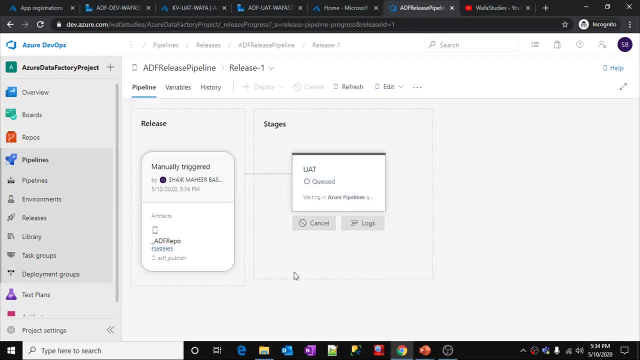 please bear with me, okay. see, you can see the status right manually triggered. you can see status already triggered and also you can see the UAT stage deployment is in progress. out of three tasks, two task is already completed. the final task is running. okay, so let's wait for. 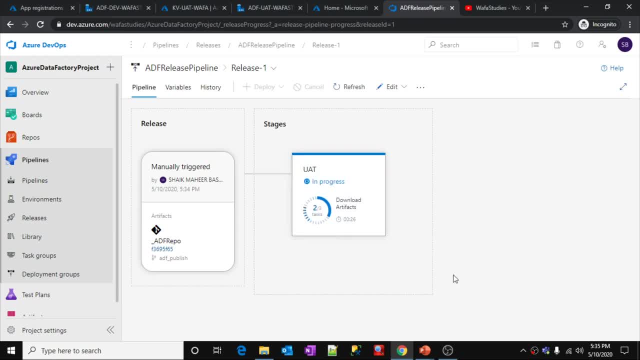 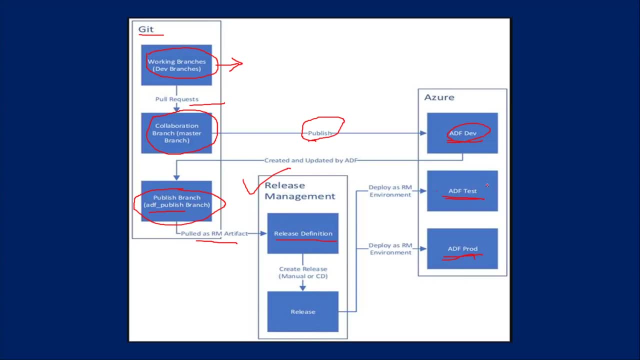 the task to complete. once the task complete, what will happen is, as I explained in this diagram, all the changes from the ADF publish. it will take and it will deploy them to UAT data factory. in this case, in the flight it is the test data factory. in my case it is UAT data factory. right, let's go there. so. 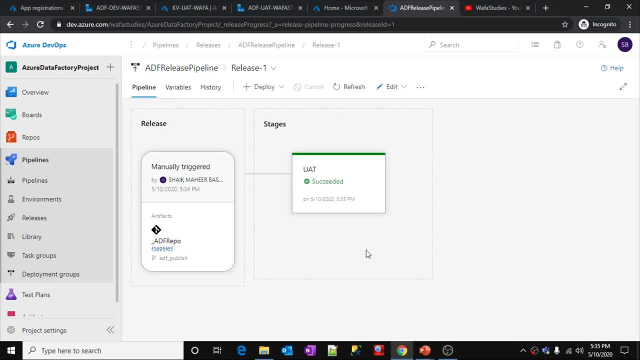 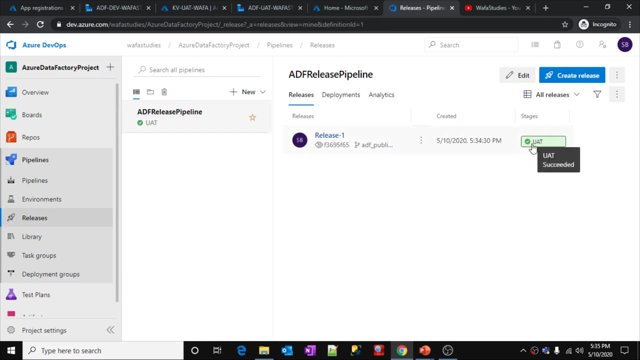 third task is running currently. status is in progress. okay, you can see status here. so that means successfully deployed. let me click this releases once again here. let me show you there also. you can see here. release one stage stages is UAT. only one stage we have. that is the reason. only one stage it is showing. 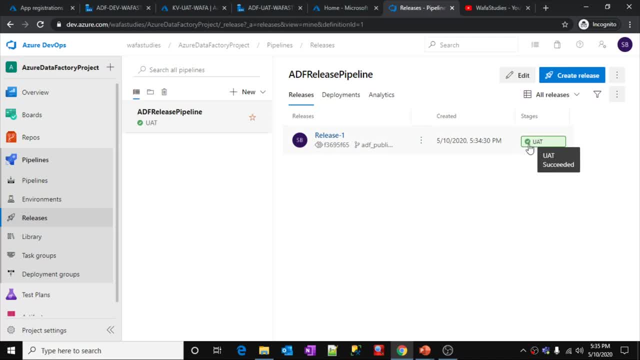 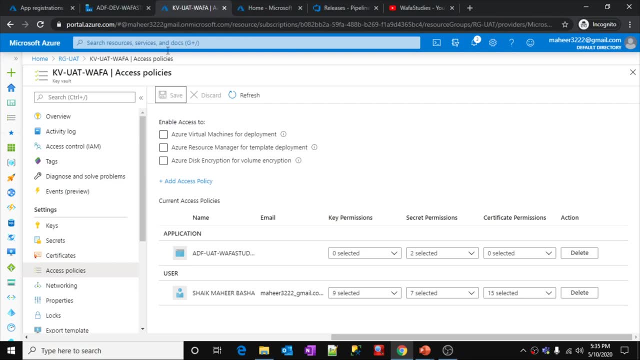 here and the status is green tick. that means it is successful. that means successfully deployed the changes to my data factory. now let me go to my data factory. let me close this, let me go here and let me go to my UAT resource group. let me open my UAT data factory, ADF, UAT for studies. 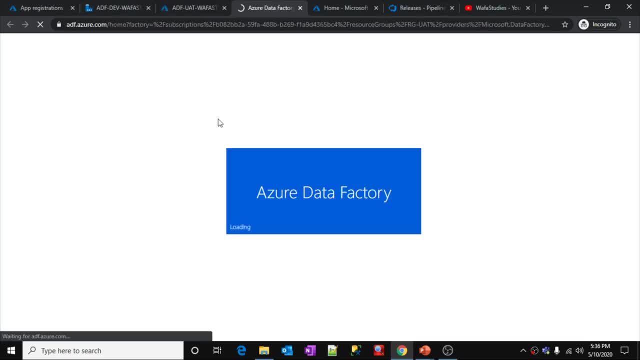 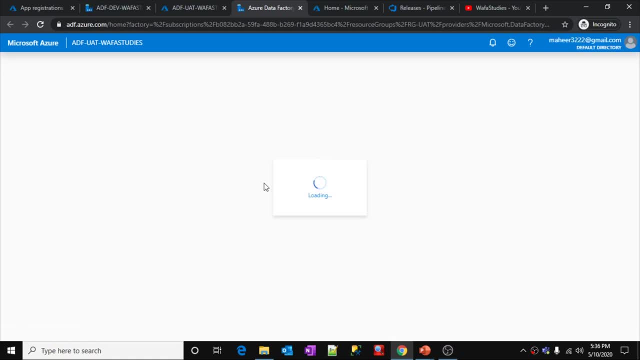 let me click this author and monitor tile here to open my data factory. so this time automatically, I should get that pipeline one and the copy activity and the data set and the linked services and everything. everything will, should, should, come automatically. and also the beautiful thing is we have provided the 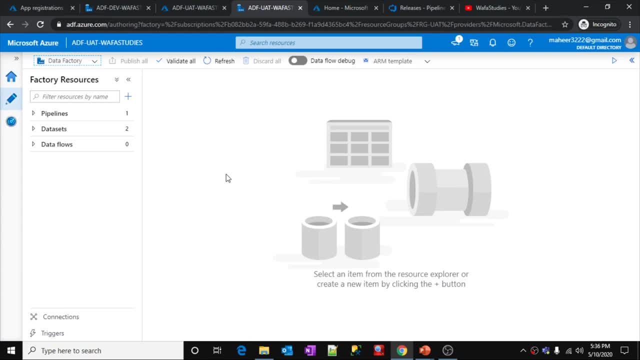 parameters right, using the key vault services and we have used the secrets and everything. and inside the release pipeline also, we have used those values right. because of that, this UAT data factory is going to interact with UAT resources. that means inside this RG UAT resource group it is going to interact. 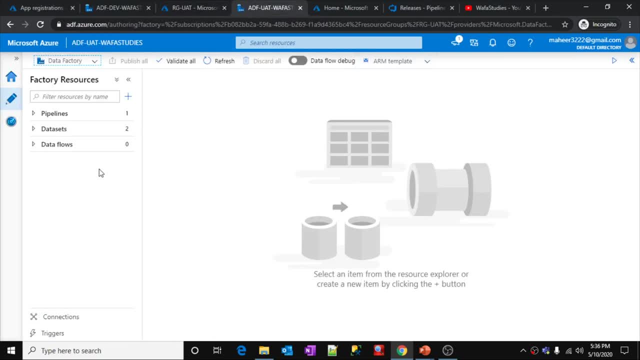 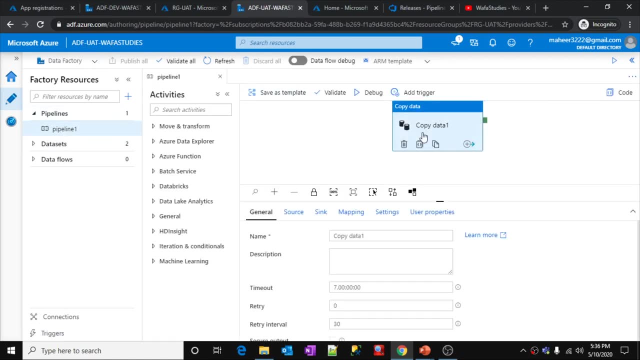 with UAT blob storage. let me show you that. see, I have one pipeline automatically inside my UAT data factory. previously there is nothing, but now I have. let me select this copy activity. let me go to source: see, I have an employee data set, also already created it here. okay, right, let me go to sync, see. 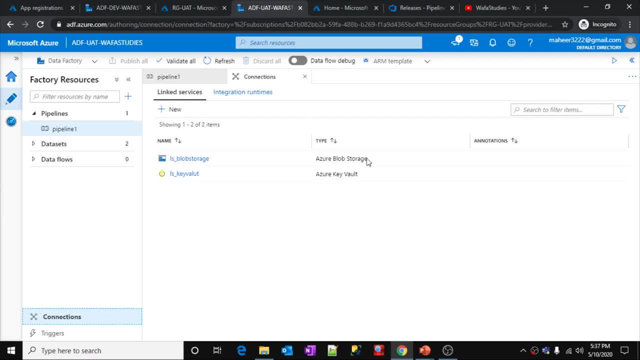 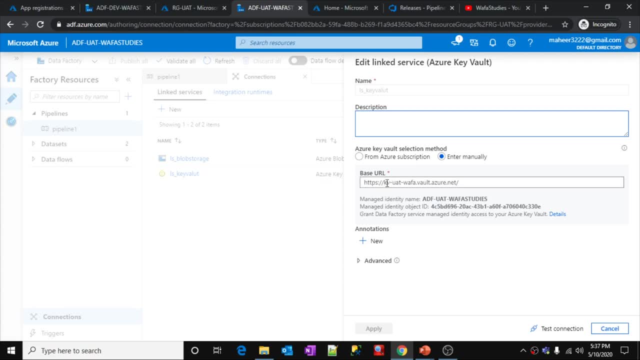 I have the output data set and everything. let me go to connections. okay, see, I have the blob storage connection string. key vault connection string. let me open key vault connection string. see, this key vault is pointing to UAT kvault. you can see automatically it is happening. 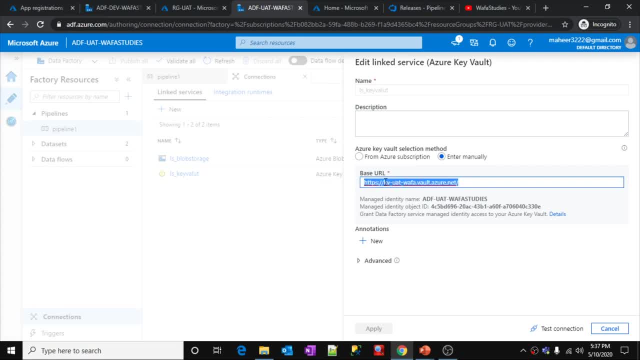 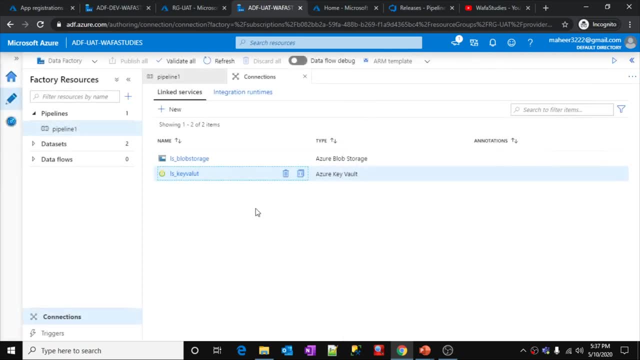 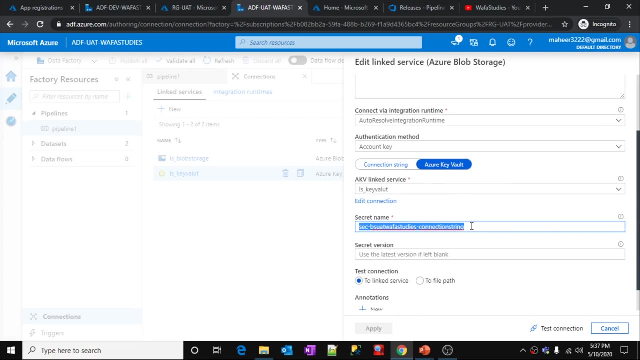 because using the template parameters, we have defined the UAT kvault URL there, right. that is the reason when it is deploying to UAT environment, it used the UAT kvault right, okay. so if I open this blob storage related connection string, see here the secret name is from the UAT right. let me click this test connection. 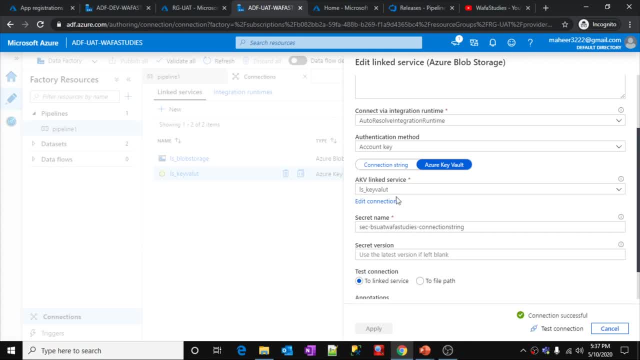 you should. it should successful work. the test connection, because few minutes before we have added that pulse is also on the keyboard right see connection is also successful. that means it is able to access this secret and take the connection string from there and it is able to access the blob. 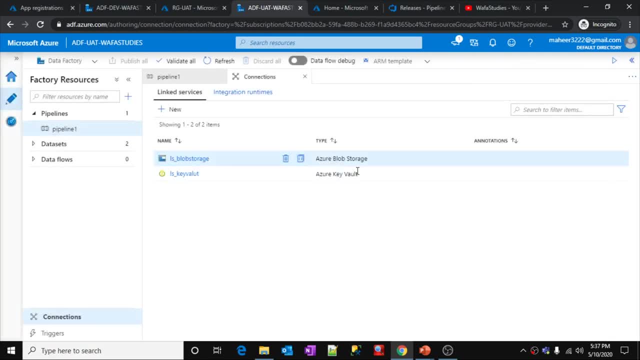 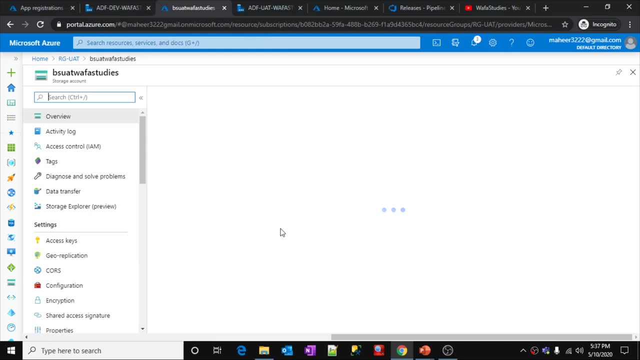 storage in the UAT. okay, so let me cancel this button. so let me go to. before running this pipeline, let me go to UAT blob storage first. okay, so let me see if I have a output folder there already and if I have a employee file already there. 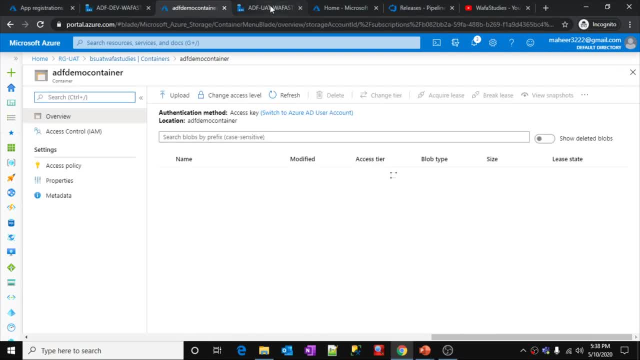 so, if it is there, let me delete that and let me run it from the UAT data factory so that it will make sure that, okay, our data factory is really interacting with the UAT blob storage and you and UAT key vault, so we can make. 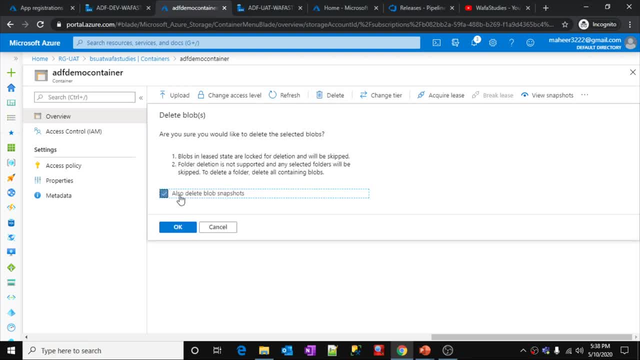 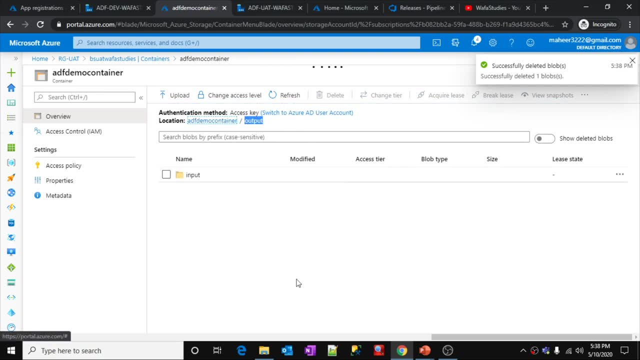 sure that right? so let me delete this employeecc file from the output folder. let me click OK. so right now I am in the output folder and I have deleted it. let me go back to my container. so right now I am in a in a UAT blob storage there is: 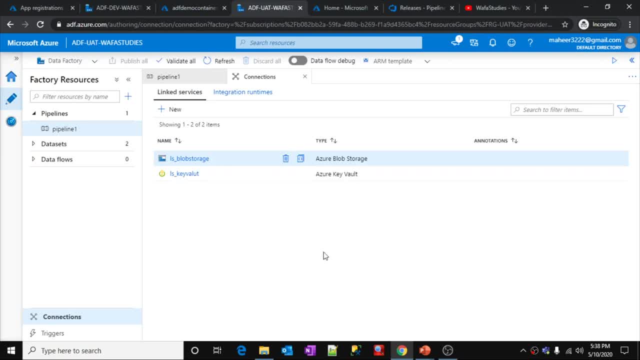 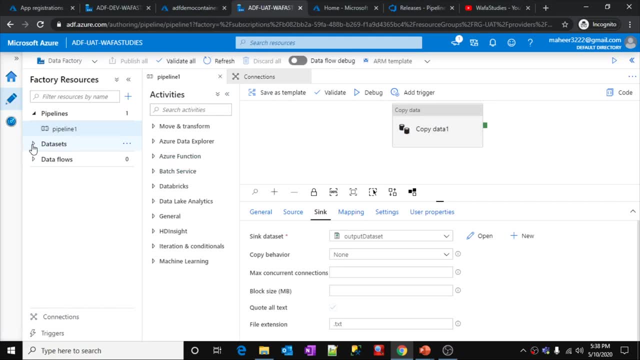 only one input folder. there is no output folder. there is no output folder, so I am in the output folder. now let's try to execute this. so, as I said, all the configurations are automatically changed to the UAT resources. that means UAT key vault, UAT blob storage. so that is the reason. now, if I execute this pipeline it. 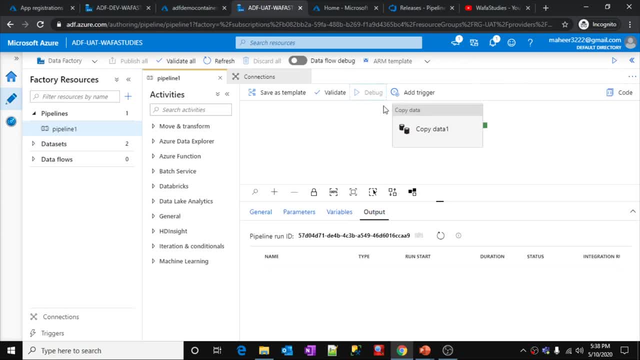 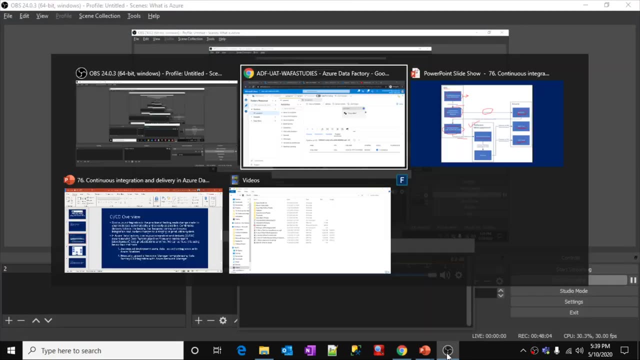 has to make the changes in the UAT blob storage. so let's, let's see right now my pipeline is running. let's wait for a couple of seconds. the copy activity is in queue status. you can say copy activity is in progress right now. okay, let's see for the copy activity come. yeah, you can see the copy activity. 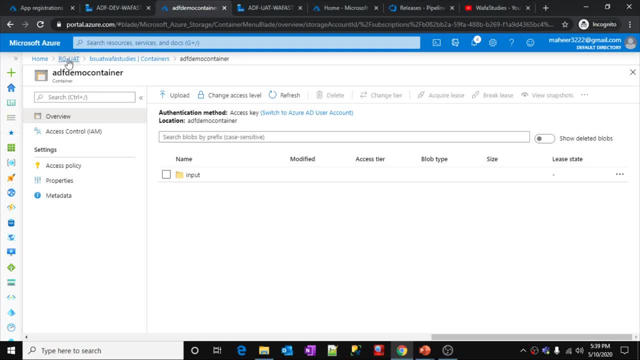 is completed successfully. now let's go to UAT blob storage. this is the UAT blob storage inside the UAT resource group. right, okay, let me refresh this here. see output folder got created. and see employeecc file also got created. and see the time step also: 10th May 539, so 10th May 539. so just know the file got. created. you can see that. so that means my UAT Bğimón multimeter file will bebleummar. the file got created. you can see that. so that means my UAT B Nevada Breckli file of exported one specific day, 10th may 539. so the open file has been saved. now let's see. 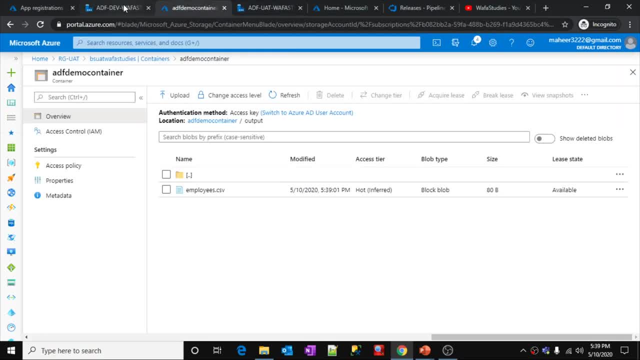 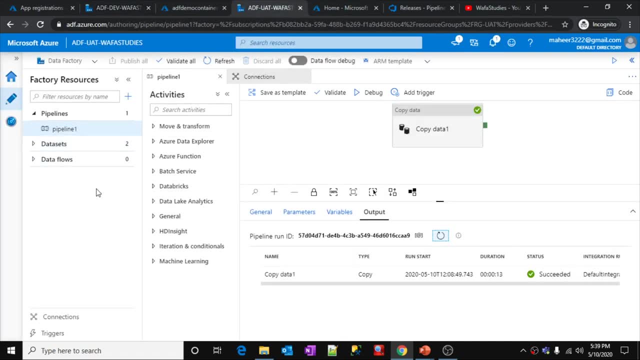 My uat data factory is working with my uat blob storage and my dev data factory is working with my dev blob storage and all the configurations are automatically changing to the uat resources. because of the beautiful, because of the template parameters, what we used inside the release. 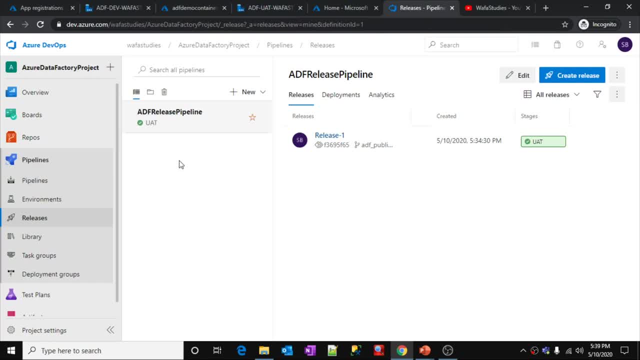 pipeline, right, so that's so. actually, you create the continuous integration and continuous deployment pipelines for your data factories in the azure devops, okay, so let me open this, let me edit this release pipeline once again. so right now, let me show you that right now, i have used only one stage, right uat stage. if you want to add another stage, click this. 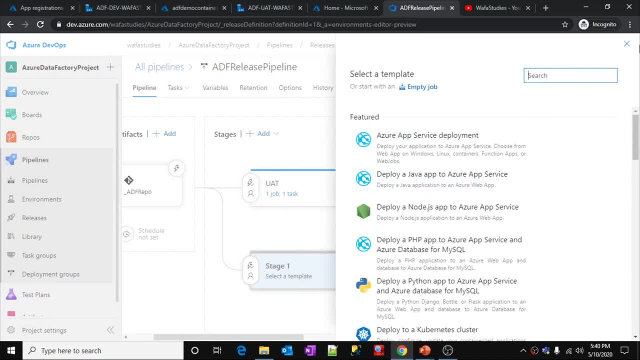 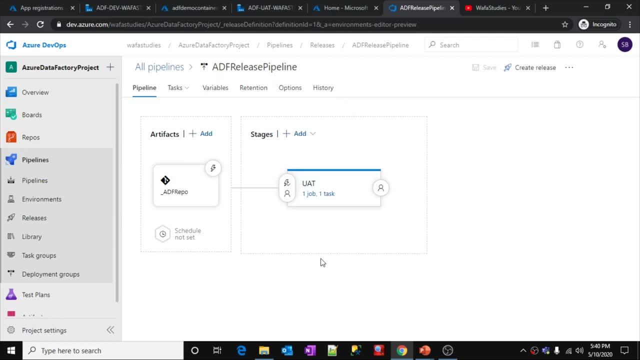 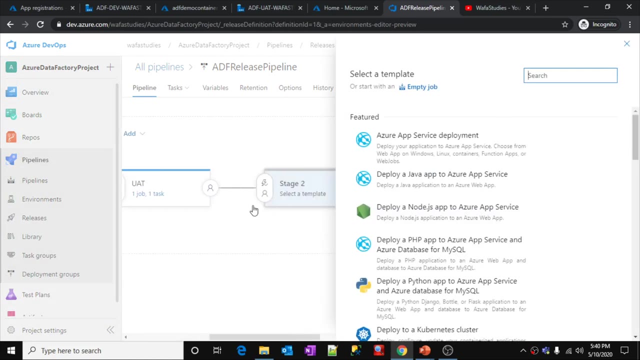 new stage. then it will ask you to give another stage name, like this: you, okay, let me close this. so here you can add the new stage also. okay, okay, it got closed, but you can add it. you can add it or no? no, i think this is not the way. maybe here, i think, yeah, see here the. 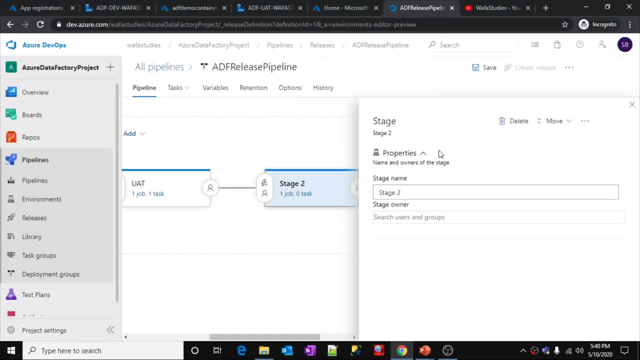 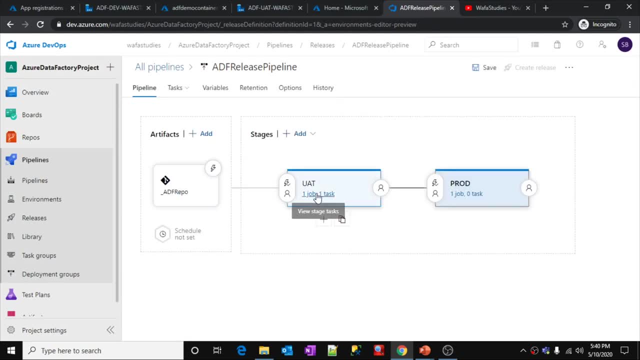 stage 2 came right, so maybe this time also empty job, maybe? so let's give a name for this one, this prod. okay, prod is the stage name. let's close this. see uat stage and prod stage, even for the process, whatever the settings, i did it here, same way you need to do it here. so then these artifacts. 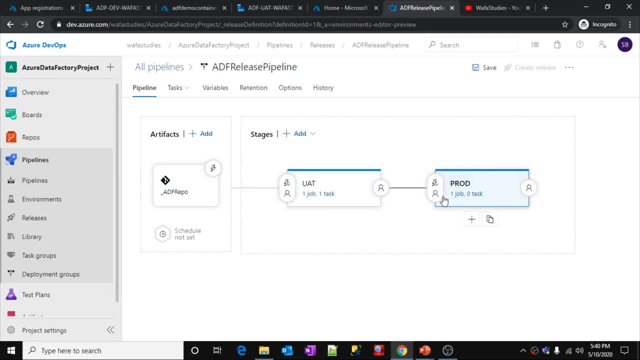 will go to uat stage and also it will go to pro stage also. so that's how it is okay. you can do that, okay. and one more thing: uh, for example, i triggered this manually by clicking the create release. right, you can schedule it also. or you can click this continuous deployment trigger. 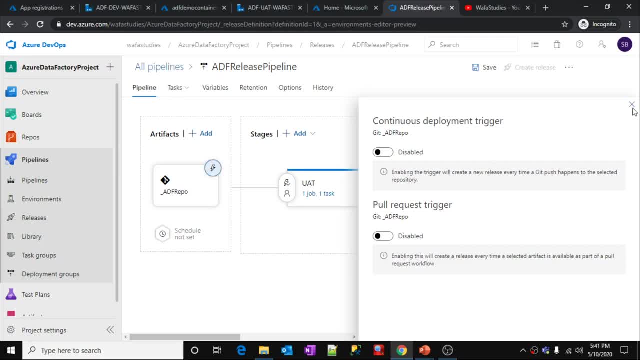 once you enable this, what will happen is, once again: once you enable this, what will happen is whenever any changes will get deployed into this, uh, ADF, this, this is nothing but ADF. publish repository right inside your data factory, sorry, inside your uh ADF demo repo. ADF underscore. 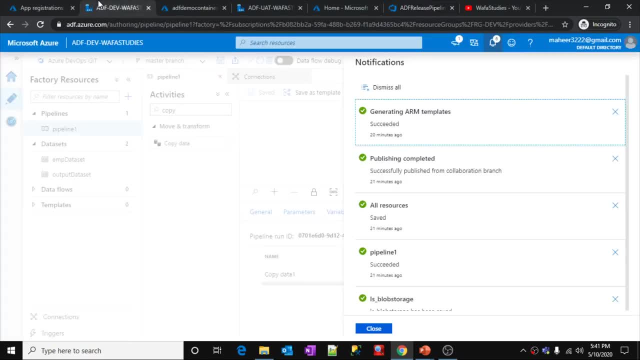 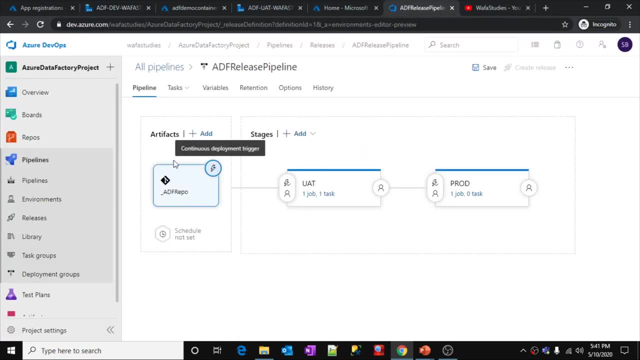 publish branch, right? so whenever you deploy anything from your dev, whenever you deploy anything from your dev, automatically your ADF underscore publish branch is going to updated, right? so in that way, this trigger. what to do to this trigger? it has to be run in the correct way. 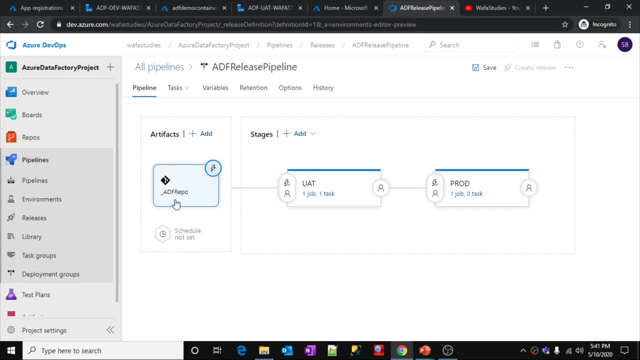 it will do, it will detect. okay, something changed in the adf underscore publish for branch. so immediately trigger this release pipeline once again. whatever the new changes came here, immediately deploy them to uat and immediately deploy them to prod also. so you can do that. okay, that means you. 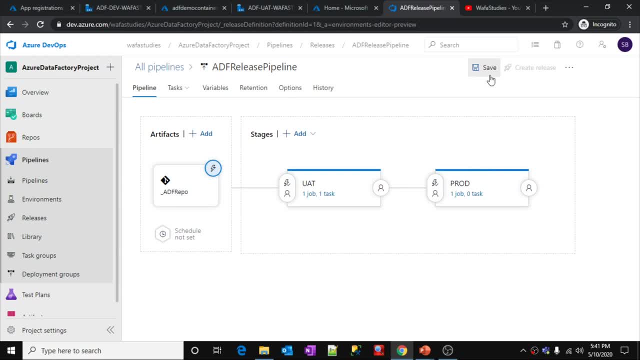 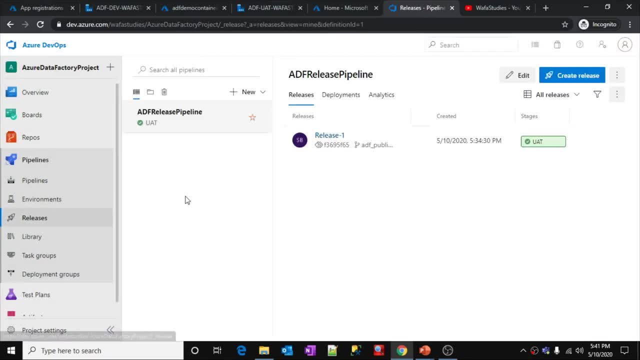 no need to come here and you no need to. uh, okay, i don't let. i don't want to save these changes. let me go to here: releases. let me click this new. so if you want to create manual trigger manually, you need to click this, create release. right, you no need to do that. if you do that, you no need to. 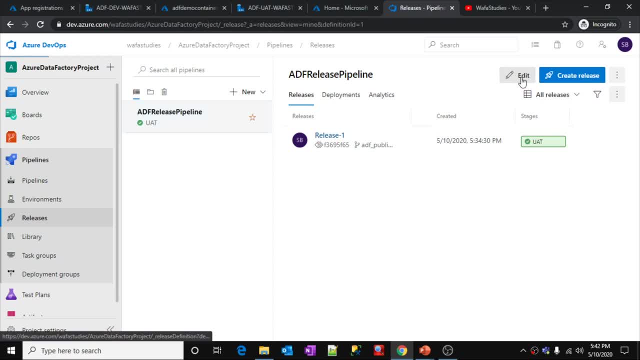 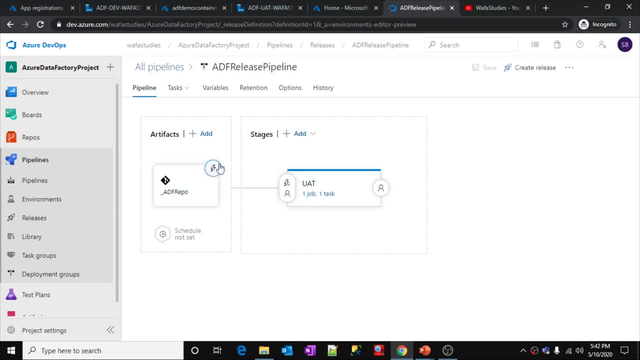 click this create release. whenever any deployment happens from the dev data factory, that is going to automatically trigger this particular release pipeline. once you enable this one, you need to click this button to enable the continuous deployment. okay, so that is what is asking. if you want to, okay, okay, okay. so i am not going to do that for now, anyhow, i am just telling you. 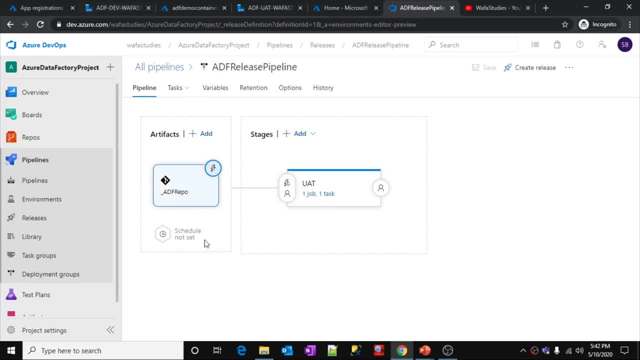 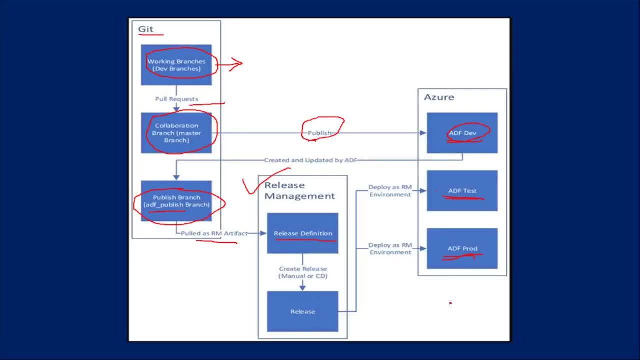 in case. if you want to do that, okay, so this is how actually your release pipelines works. hope you got a clear idea how the release pipeline is working. let's go to you our presentation. okay, so we have discussed this slide in detail. okay, so thank you for watching. 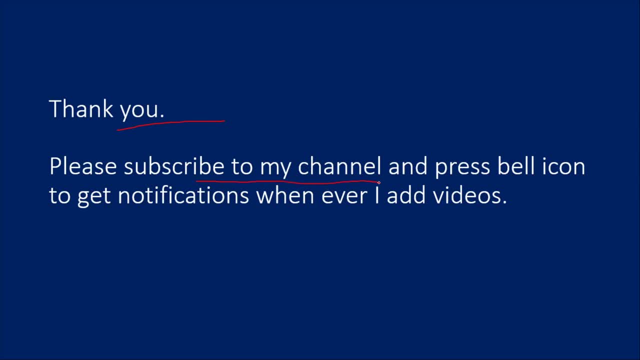 this video. please subscribe to my channel and press bell icon to get the notification whenever i add videos. thank you.